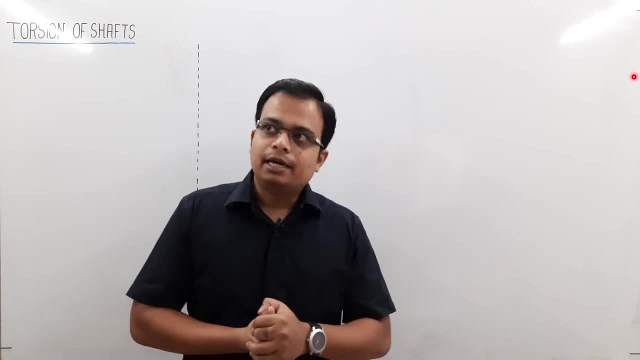 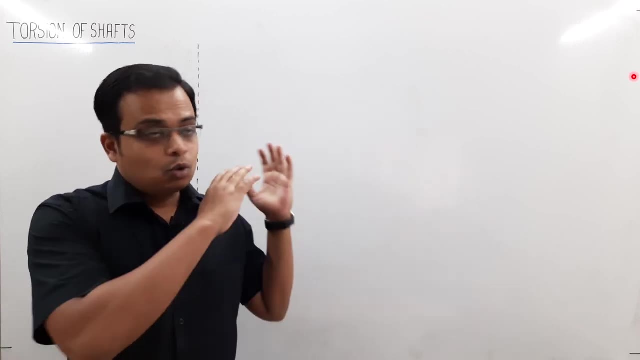 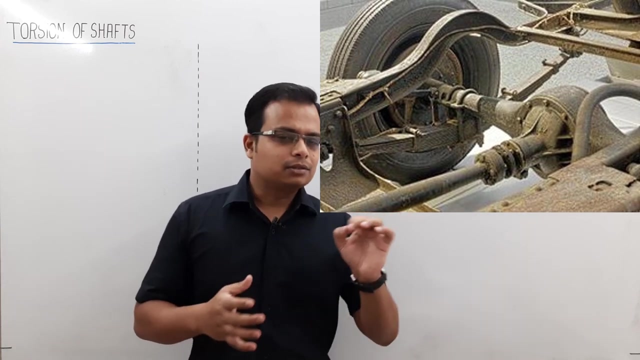 must be wondering. so why, all of a sudden, we are studying about shafts in mechanics of solids. we have been studying about beams- yes, they are very important structural members, and so are these shafts. yes, you heard that right. just take a look at this. what is this? this is the drive shaft of an of an automobile. 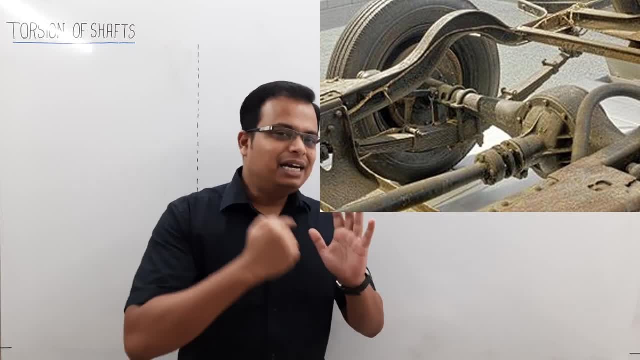 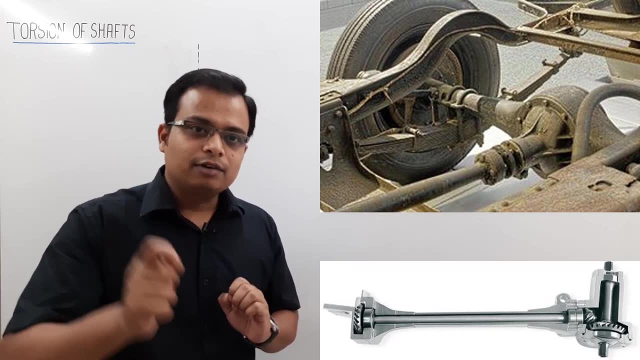 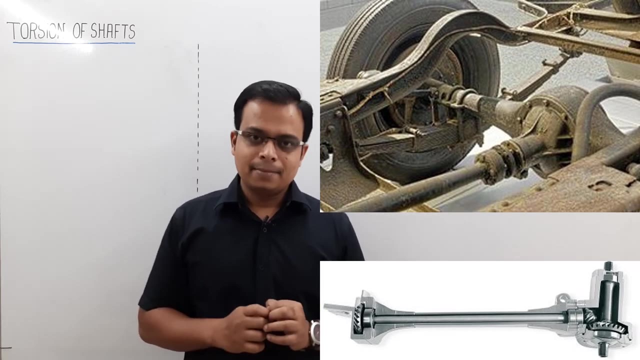 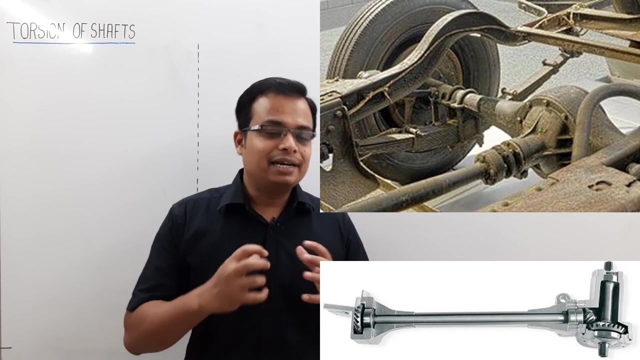 this shaft tends to be rotating continuously as long as the vehicle is on right, and obviously there is some kind of torque involved. you heard that right, there is some kind of torque involved. as an automobile engineer, as a mechanical engineer, it is your prime responsibility to understand how this shaft behaves and, based on that behavior, you should be able to design it. 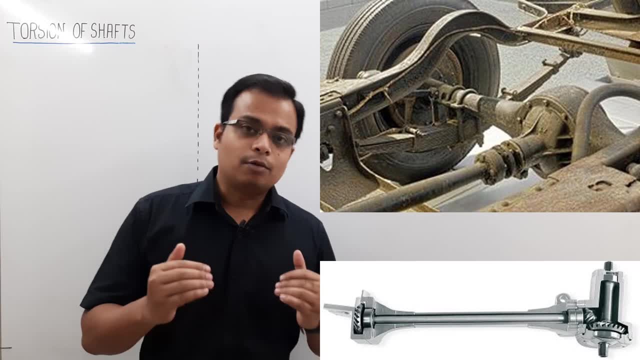 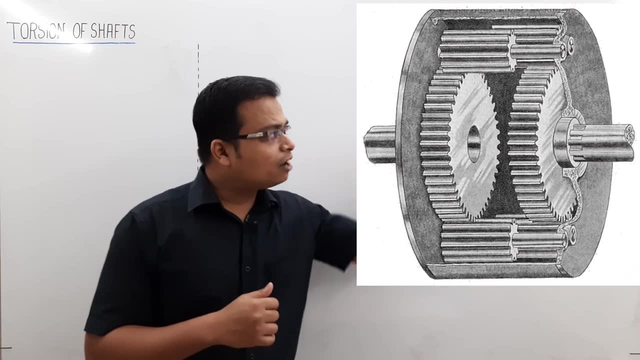 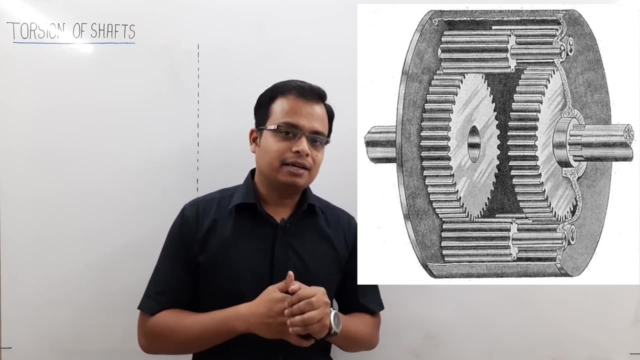 and ultimately be able to work out whether it is going to fail or pass right. so these things are very important. you must have seen some arrangements like this. you see this shaft over here carrying some, some pulleys. it might be carrying some gear gears also. so obviously there are transversal loads. yes, there are in the x, y and z direction. 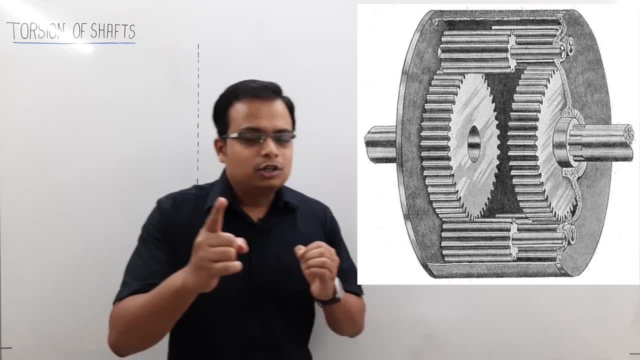 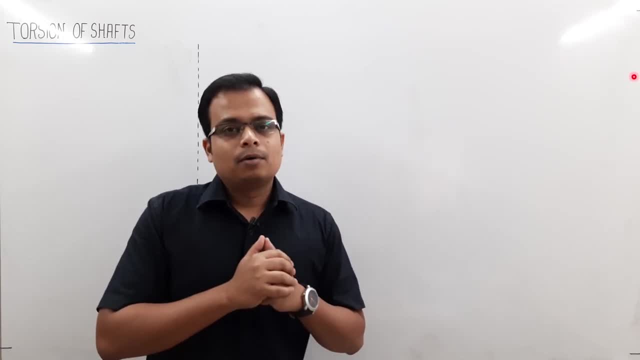 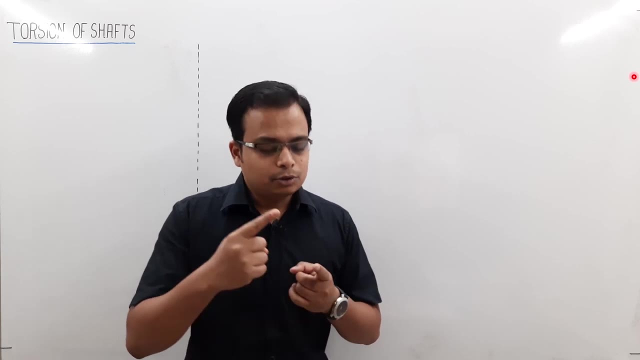 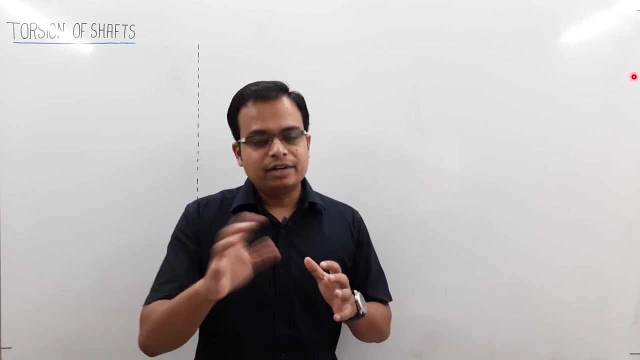 but obviously there are going to be some- not loads, but some kind of torque which is actually acting on its cross-sectional area, on the surface, tangentially, obviously, right, so this creates some kind of stress. whenever you talk about tangential forces, you talk about tangential stresses, which are popularly known as shear stresses. so all of that will come into the. 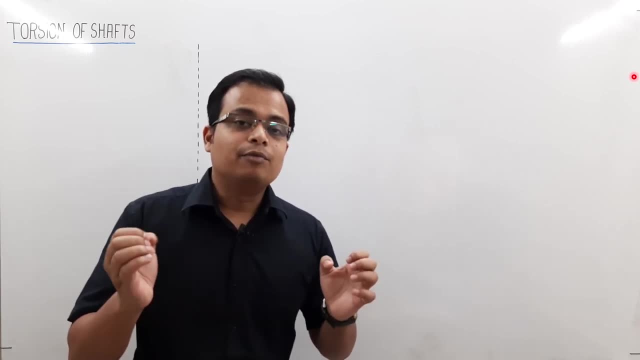 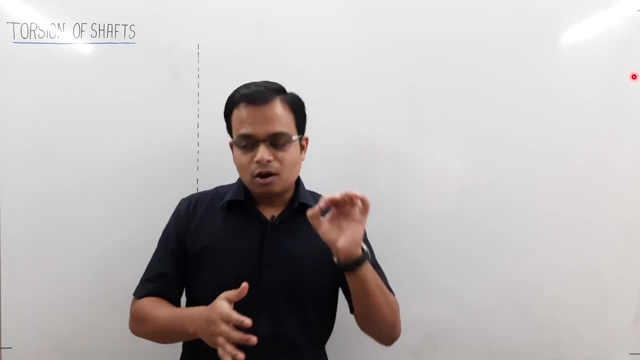 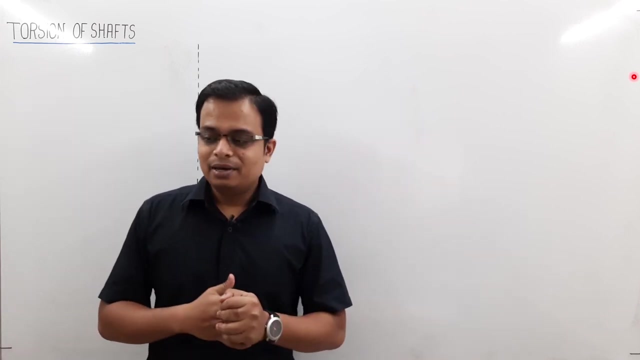 picture right. so we won't be talking about loads. rather, we will be concerned with what happens to a shaft when it is subjected to a torque, and that is going to be the agenda of today's session. and, without further ado, let us begin the first chapter of today's episode with an experiment. 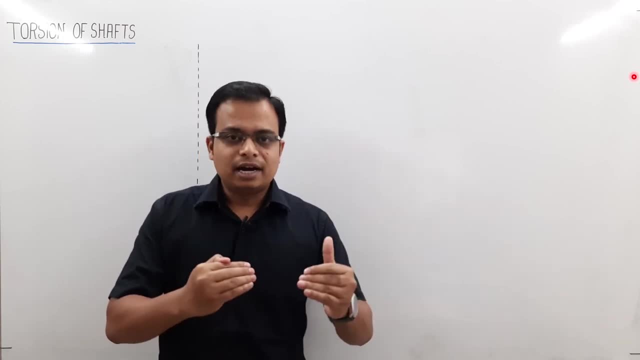 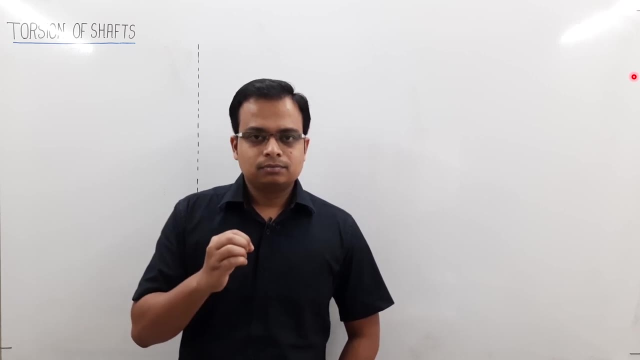 there are going to be several chapters and i'll be taking you through all of that and it is going to be fun. now, small piece of advice for all of you: if you want to finish this video in a small duration of time, watch it at a higher pace, preferably 1.25 x or even more right, and if 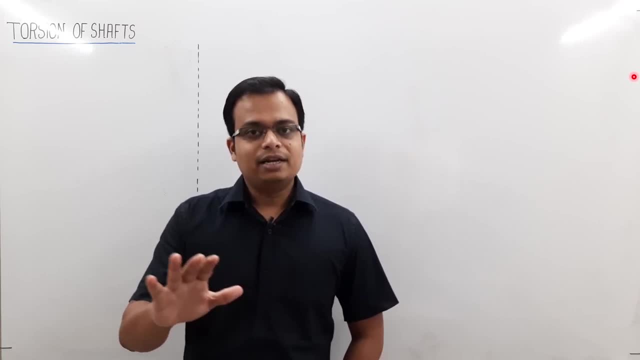 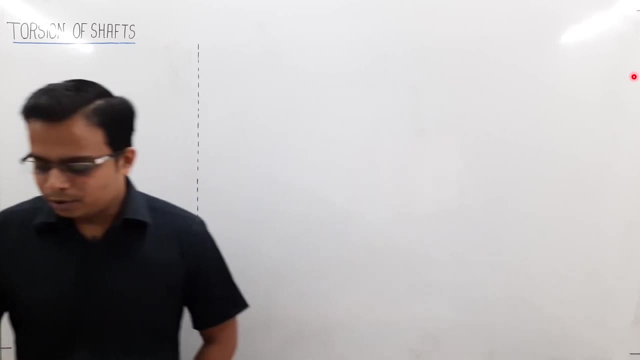 you've got time, just like i have, then don't worry, watch it at the normal pace. and here we go. it won't take much time, right? everything will be simplified and here we go, let us start the experiment. so what do we need for an experiment? we need a specimen. this is the specimen. consider: 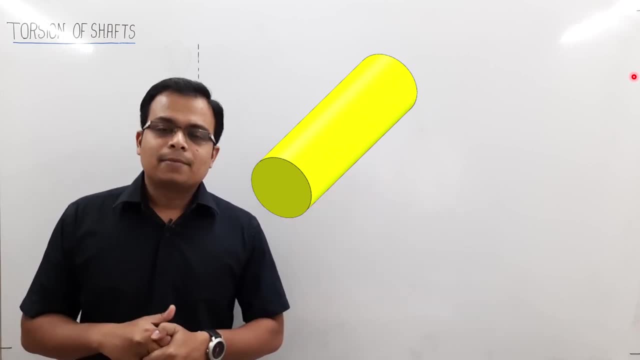 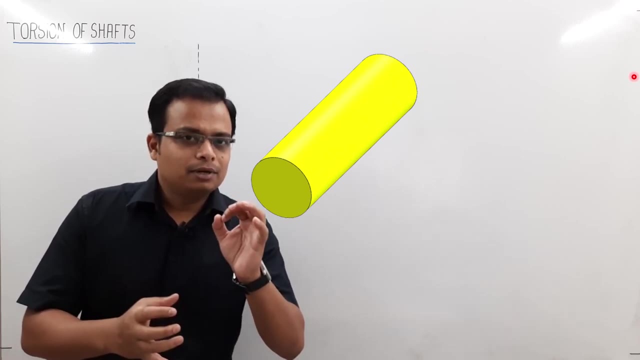 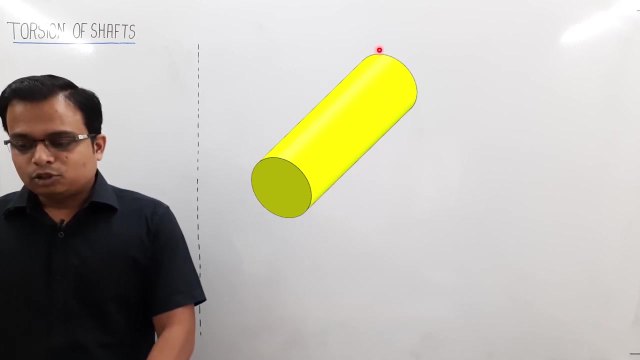 this specimen is not complete. you know there are, or there is, a lot of preparation which needs to be done before taking it to the torsion test. just just try to grasp and consume whatever i say. okay, the first thing which i'll do is this specimen happens to be having two ends front. 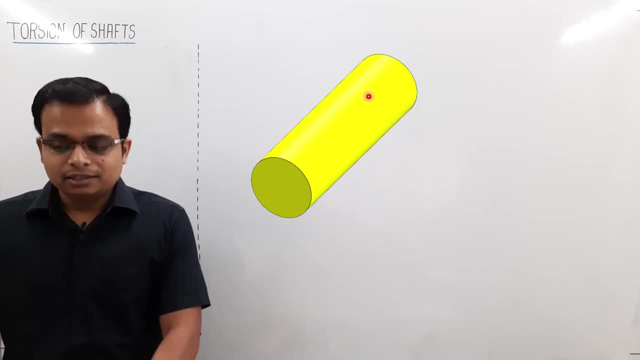 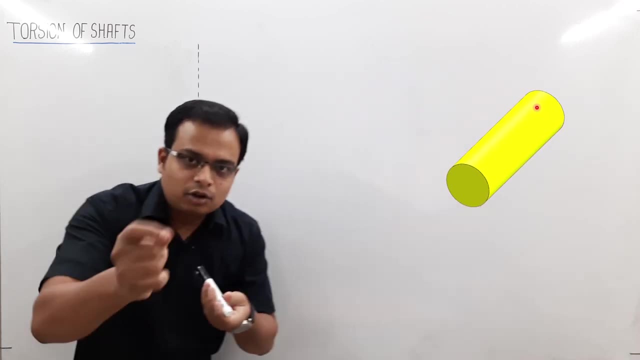 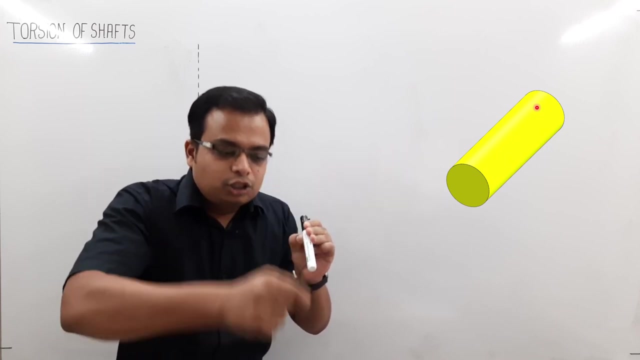 back circular, circular, center, center. when you join those two centers right from here, this center, the line that you have is a longitudinal axis and what we'll do is we'll have a sketch pen and let's say: this is the shaft. we'll make lines parallel to that longitudinal axis, something. 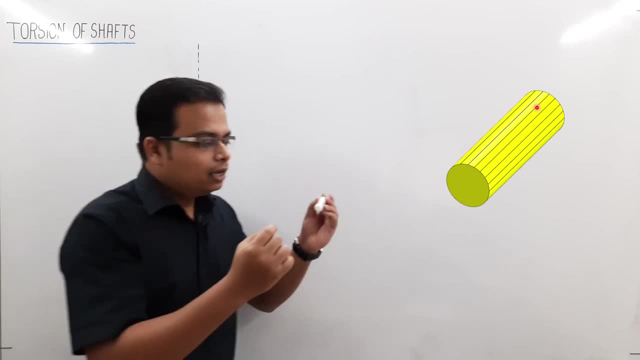 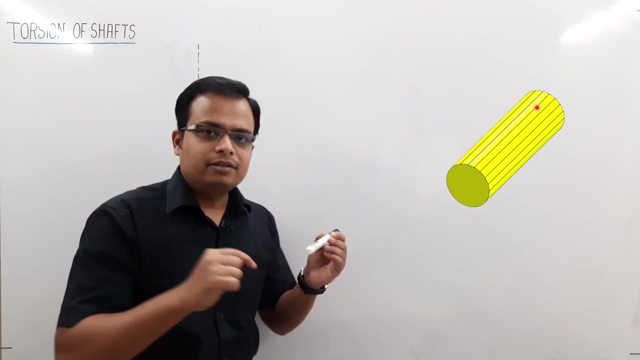 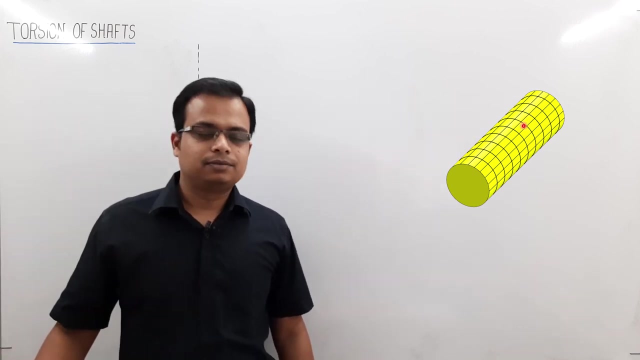 like this. hope you got the point. secondly, with the same sketch pen- this is the mild steel circular shaft that we have- we are going to make concentric circles. right, this is rather a fictitious experiment. right now, let's say something like this, and then you can see whole lot of rectangles. anyway, we'll. 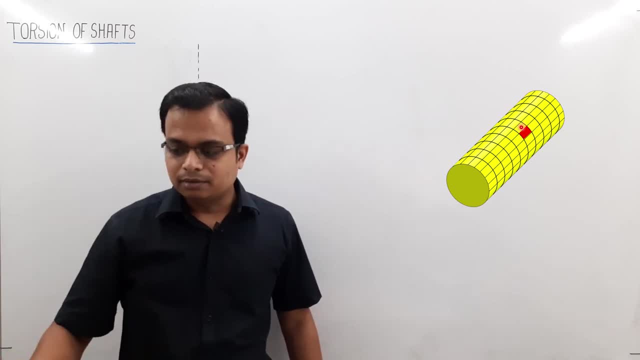 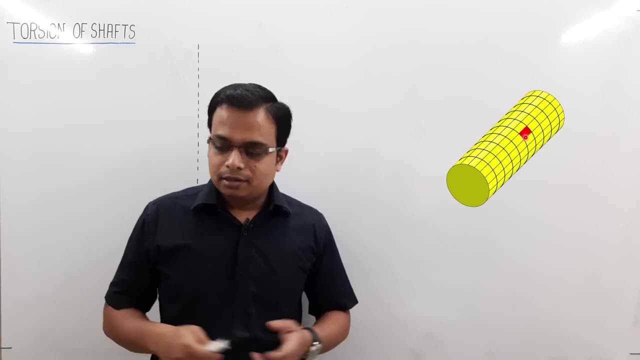 have one, any one rectangle, and we'll sketch it, let's say, with red color. it would look something like this: beautiful, isn't it? now, obviously, all of you are having cell phones, okay, or a camera. let's say, and you are going to take a picture of this rectangle, exactly if this is the shaft and this, 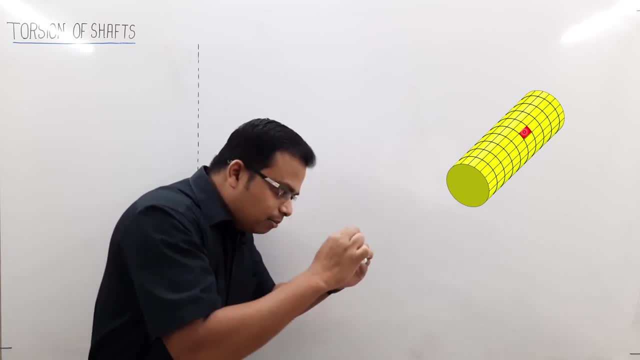 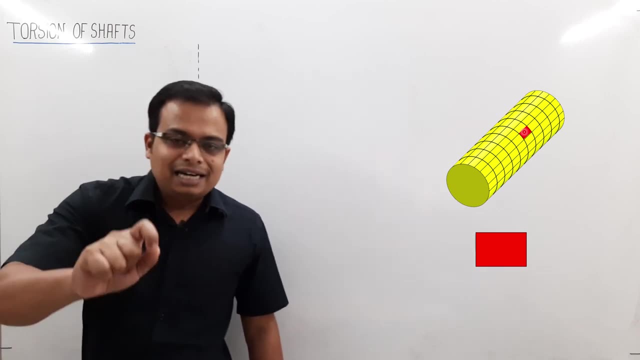 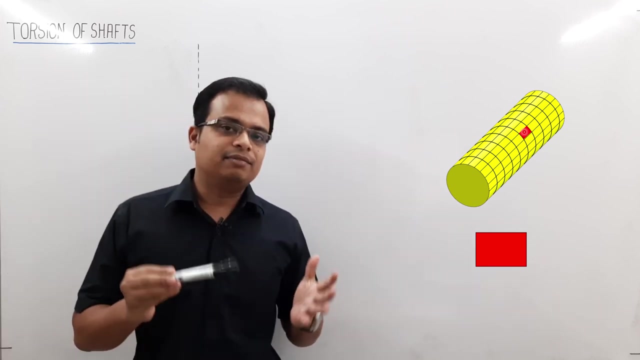 is the rectangle. you are going to keep it, keep the camera camera exactly above it and you are going to take a snap. and this is how the snap looks: like: lovely. that is the preparation of this specimen. now, what we'll do is we'll take it to the torsion testing machine, and let me just 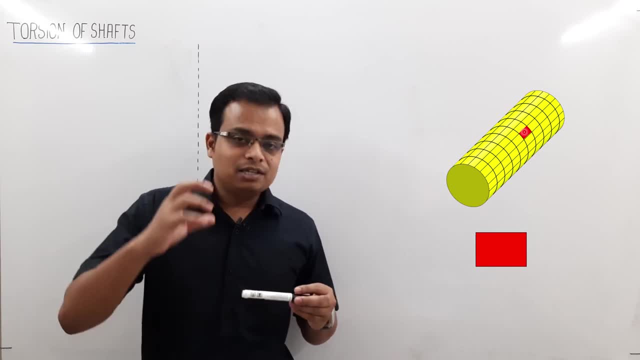 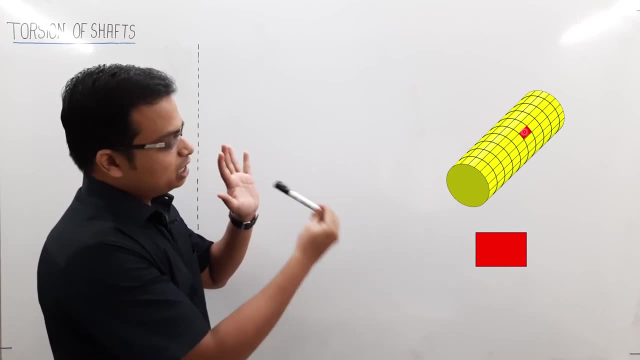 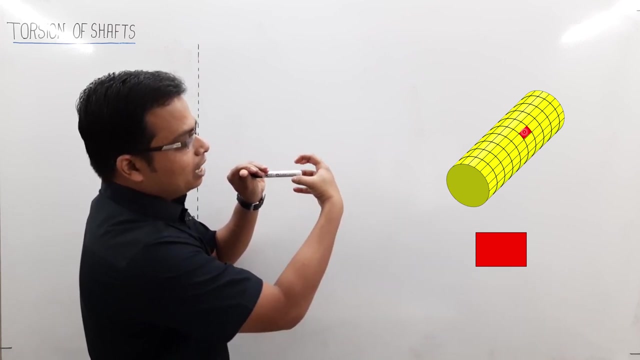 give you an idea of how. what is the main objective of having a torsion testing machine? so basically, what we do is: it's got two jaws, one joy is over here, so we'll fix this specimen over here something like this: and this is the jaw where the other end of the specimen will be fixed and we are going to 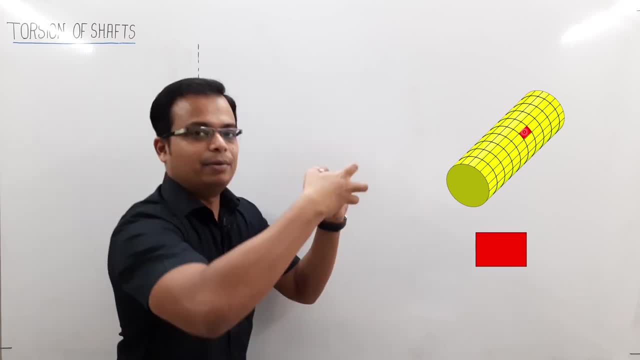 apply some torque. torque is something like this- a twisting moment, you can call it. this is the twist, right? so what we're going to do is we're going to take this specimen over here and we're going to apply some torque. torque is something like this- a twisting moment, you can call it. this is the twist. 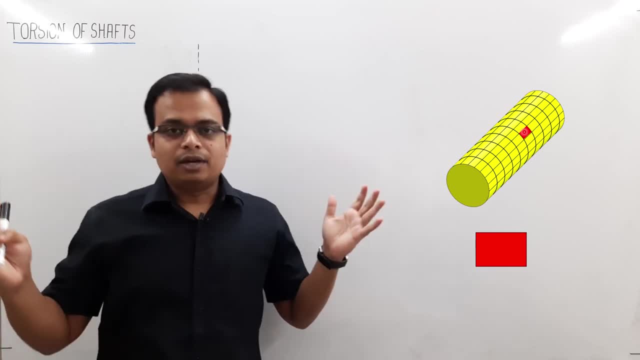 right, so we're going to apply some torque torque. is something like this: a twisting moment, you can apply some torque torque. is something like this: a twisting moment, you can apply some torque torque. that is exactly we want to observe and, based on that philosophy, a whole lot of relationships. 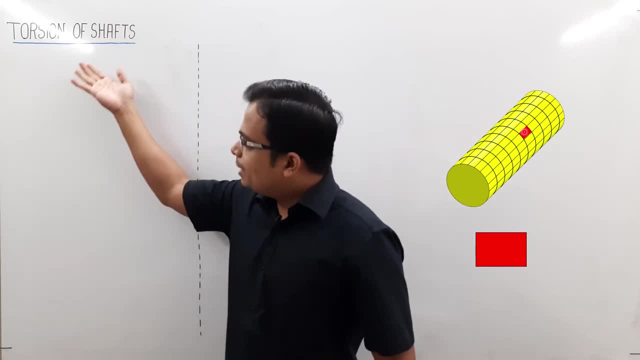 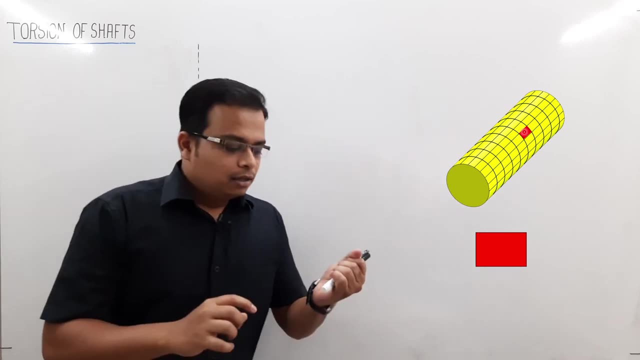 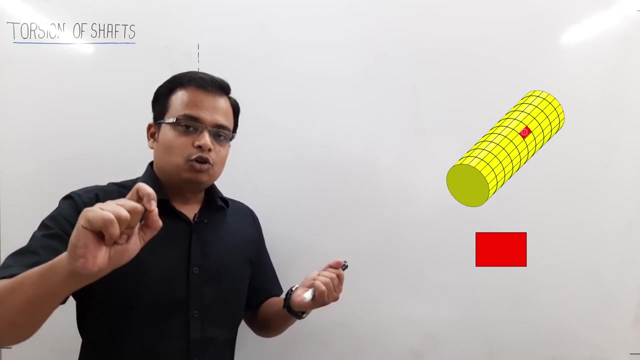 will be developed and in the course of time i'll be putting them up one by one over here. you will understand that very soon, okay, so when you give it a twist, right, don't give much of a twist so that it is unable to regain its original shape and size. that twist should be to that extent. 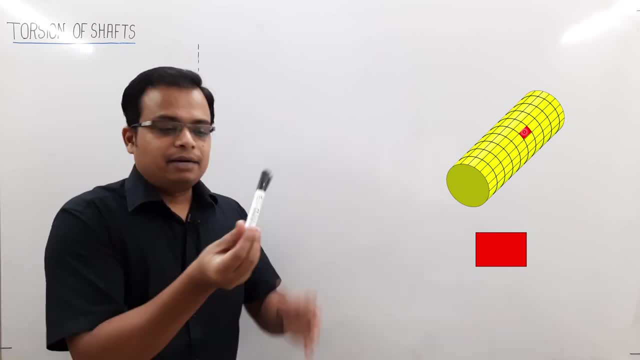 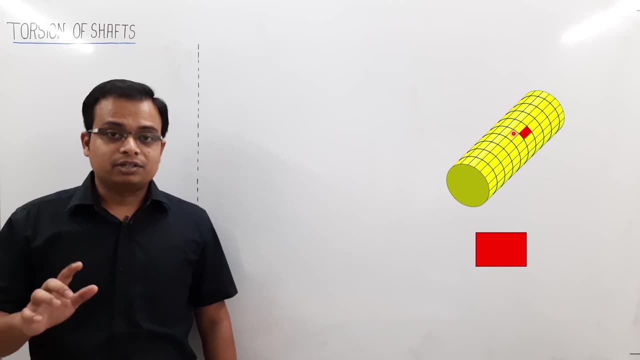 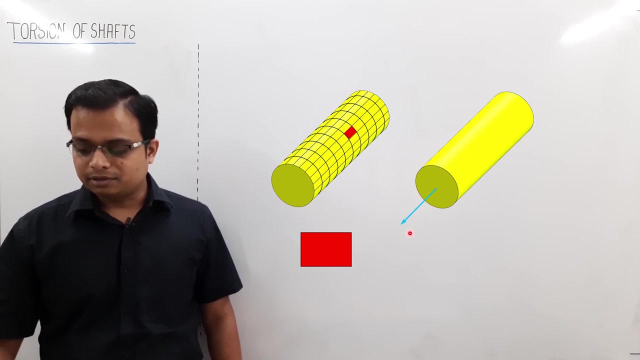 that after you remove it, after you remove the torque, the mild steel specimen should look exactly like this. right, it should be able to regain its original shape and size, so elastic constants will come into the picture. this is how the specimen would look now with respect to this axis. we'll apply the torque somewhat along this face. that is the torque. 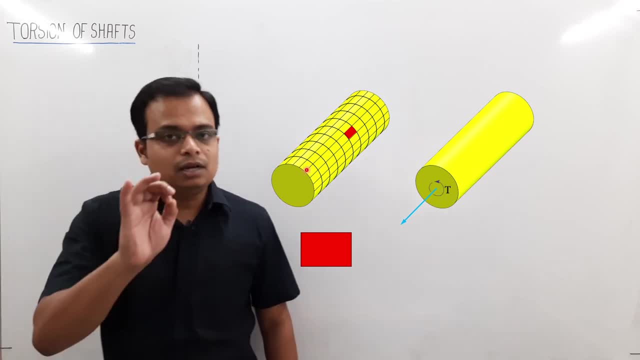 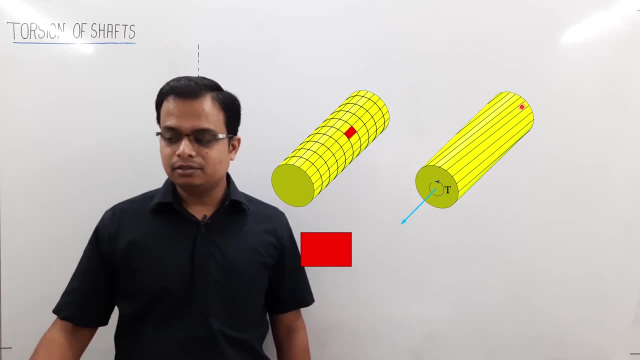 and all the lines. these lines here happen to be parallel to the longitudinal axis, and now they will no longer be parallel to the longitudinal axis. you can see that very easily. see, this looks inclined, isn't it? here they are parallel. they are parallel to themselves, but apart from that, 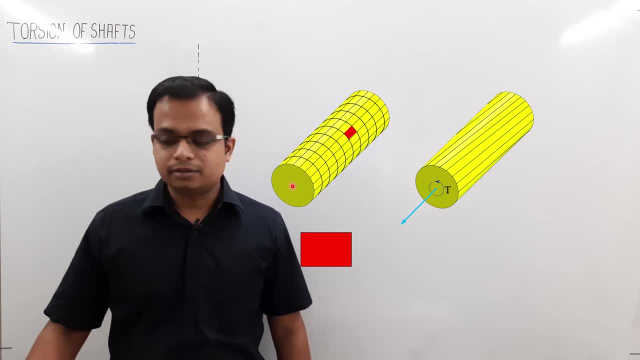 they are also parallel to this longitudinal axis passing through the center. obviously here, yes, they are parallel to themselves, but but all of them seem to be making some kind of angle with the longitudinal axis. with this axis, let's say, okay, let me make these circles also. the circles will. 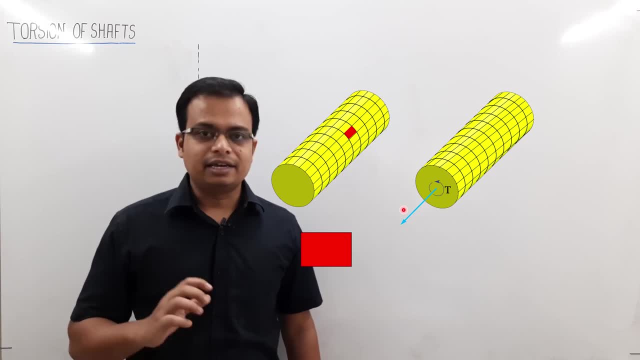 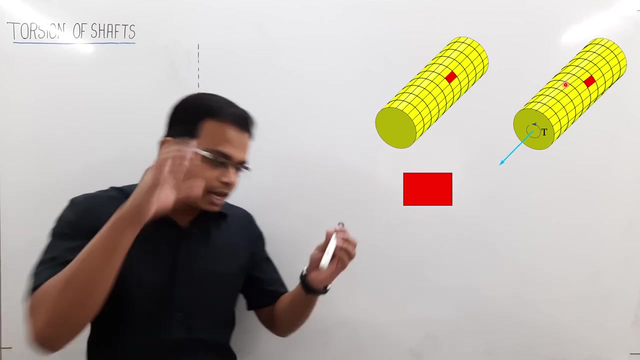 rotate at their own places. radially they'll rotate, but nothing else is going to happen, whereas these lines- well, the directions of these lines- have changed before the experiment and this is after the experiment. and now let us take a look at this red patch. here we go. that's the red patch, and if you again hold a camera exactly above it, if you 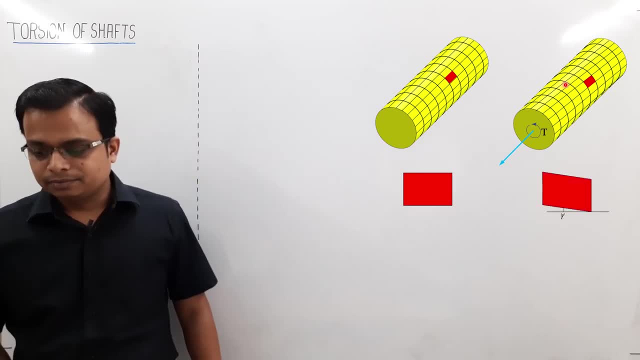 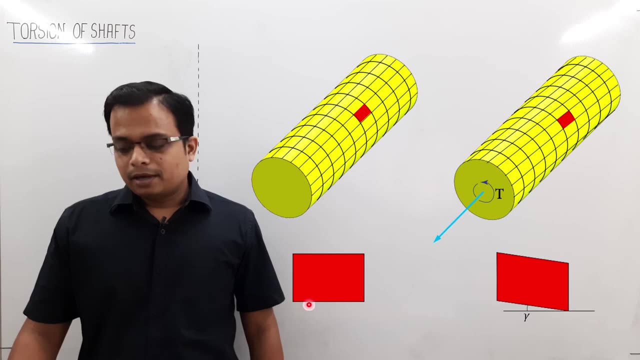 click a picture. what you shall see is something like this: strange, isn't it so? when you apply the torque, something strange has happened. so these two sides, originally at an angle of 90 degrees. now, these two sides, this one and this one, they are no longer at an angle of 90 degrees. or let me frame the sentence in this fashion: initially, this was: 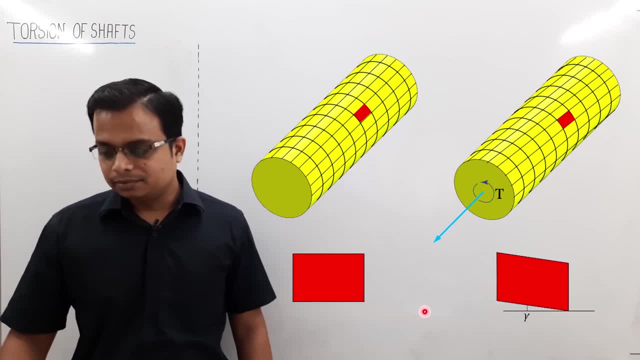 absolutely horizontal, or let's say it was parallel to the longitudinal axis, but now it is no longer horizontal. it seems to be making some kind of angle with the longitudinal axis. how much that's gamma. this is nothing but the shear strain. whenever you talk about changing angles, you talk about 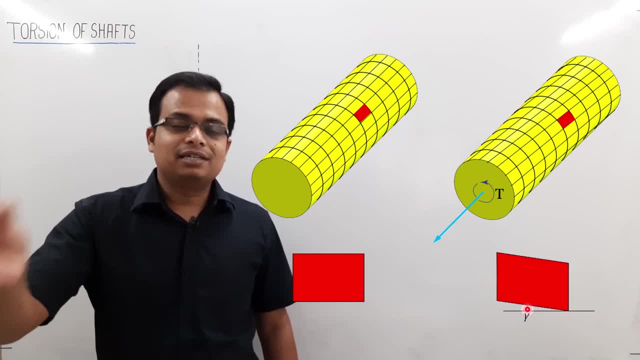 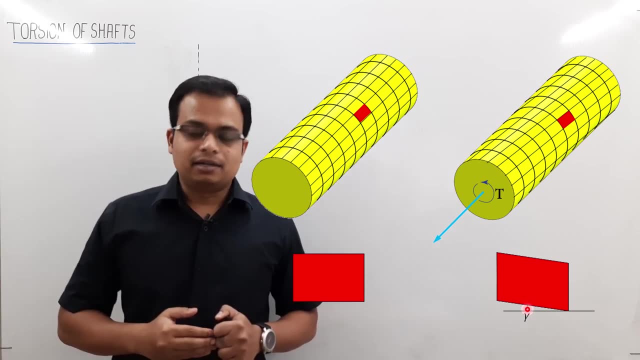 shear strain. when you talk about shear strain, the kind of stress developed is shear stress. that's it. this gives us the motivation to go for it, and that's why we are talking about shear strain. so let's go ahead and investigate what is the matter. so we'll break it down to very small pieces. 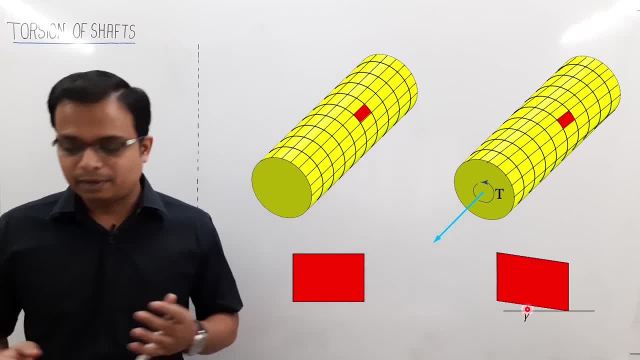 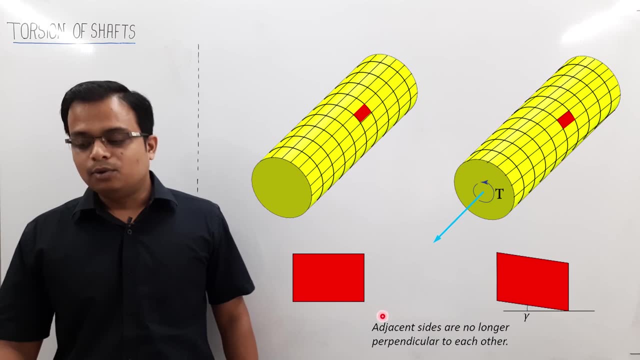 and we'll understand the matter and we'll develop relationships. so that was the experiment, and the conclusion of the experiment is that adjacent sides, these two sides, let's say this one and this one- are no longer perpendicular to each other. okay, here you can see that are no longer perpendicular. 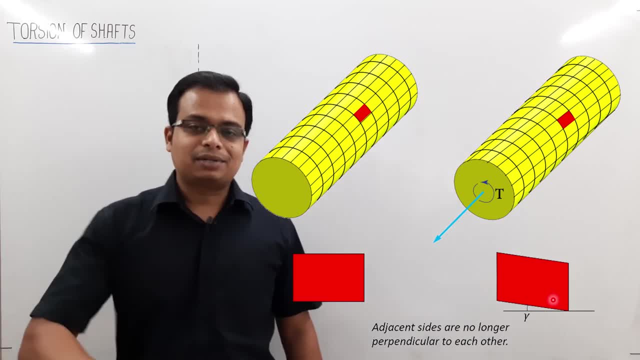 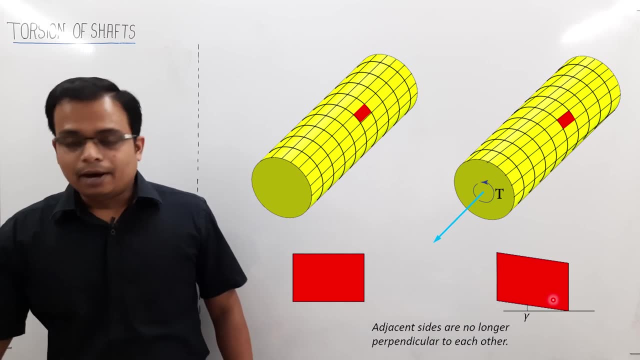 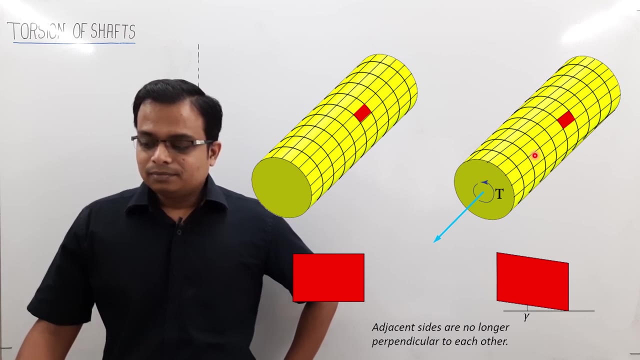 to each other, which indicates the presence of some kind of strain, which is known as shear strain. and this is the department of shear stress. and now, now just take a look this line over here, just listen to what I say very carefully. assume that this line happens to be part of a plane which passes. 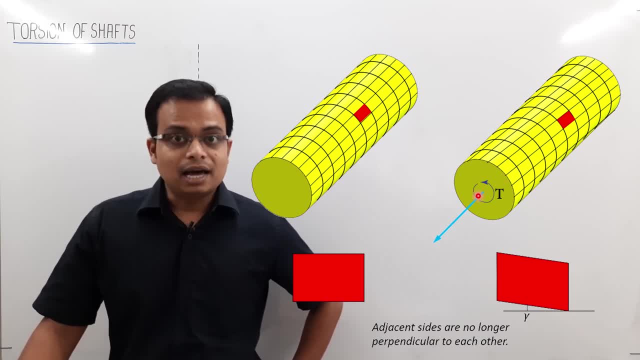 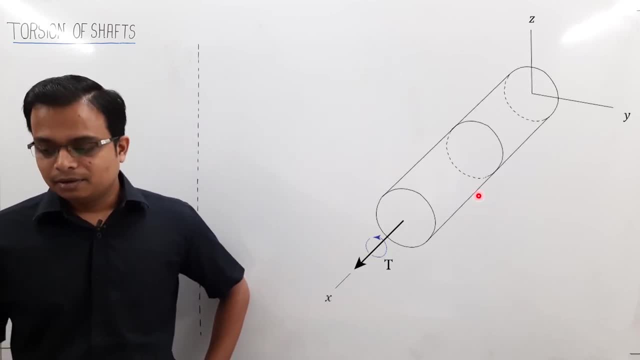 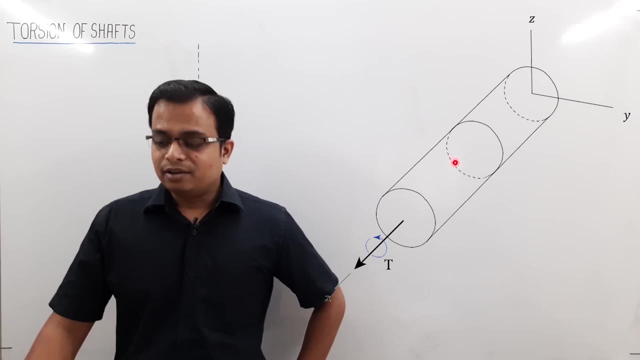 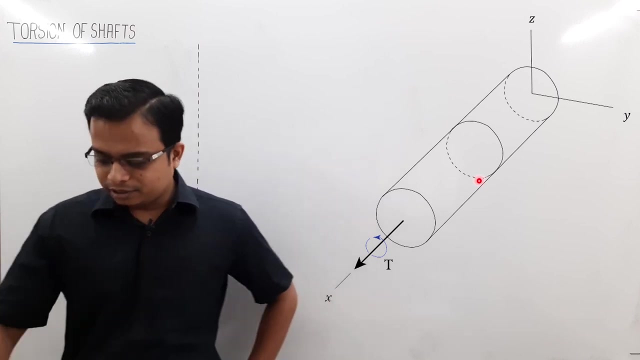 obviously through the, through the longitudinal axis. okay, let me make it rather: here we go, lines then and planes now. this is still a solid. I've made it transparent so that we can visually see how the internal part of this circular shaft is. just take a look at this, and what we'll do is we'll make two points over here, one over here. 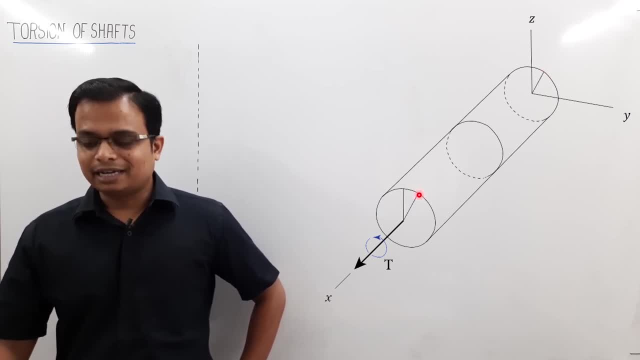 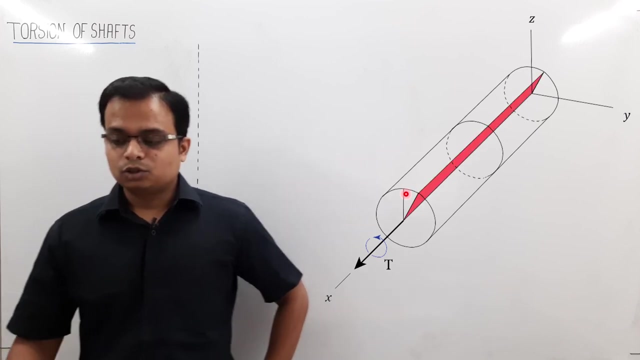 and one over here, and we'll make radial line something like this: right, exactly a photocopy of this. this angle and this angle is same. okay, now what we'll do is we will make a plane. we'll make a plane containing these two lines and would look something like this. so originally the plane is like this. okay, now, when the torque is, 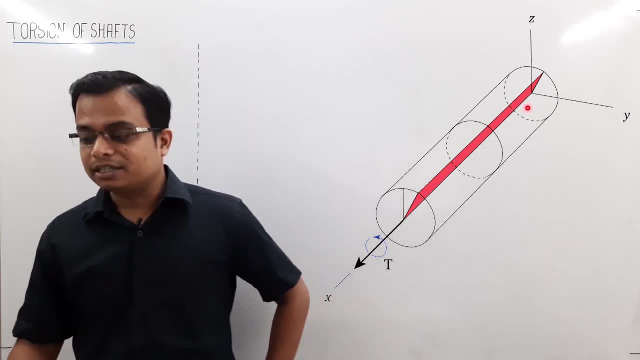 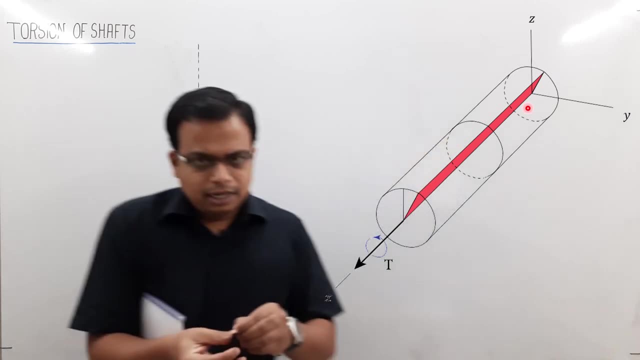 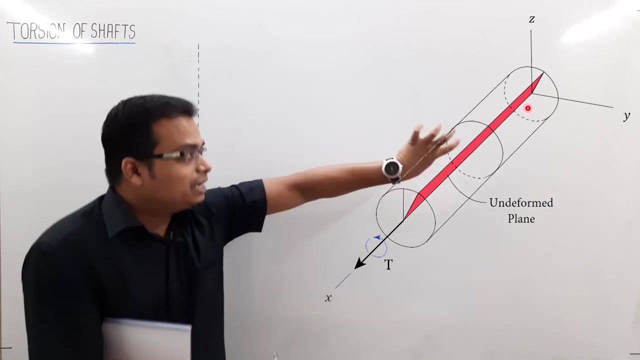 applied. what will happen? just think about this. what will happen to this plane once the torque is applied? one sec, one sec. just think about it. what will happen to this red colored plane? this, initially, is undeformed, right a torque has not been applied. what happens once the torque is applied? 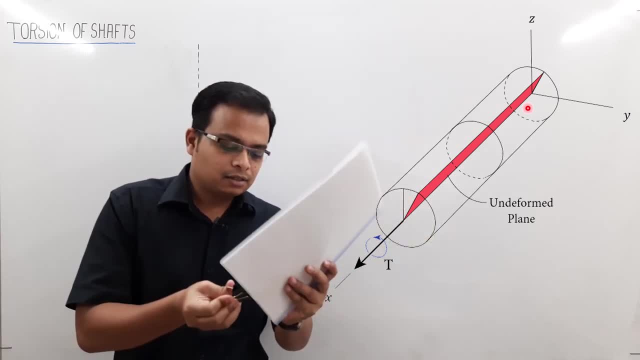 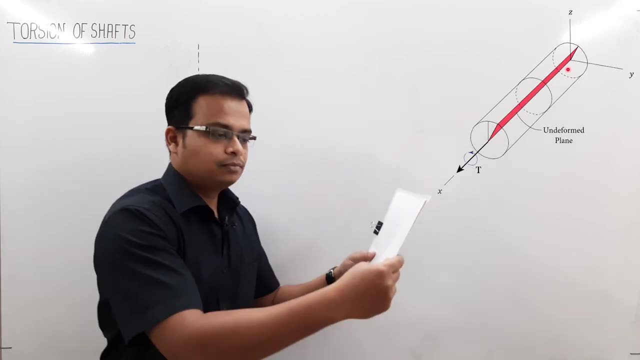 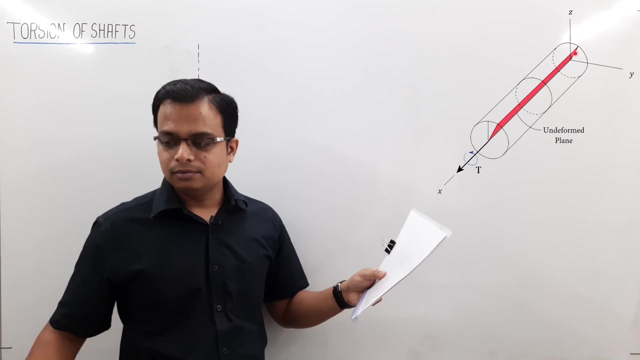 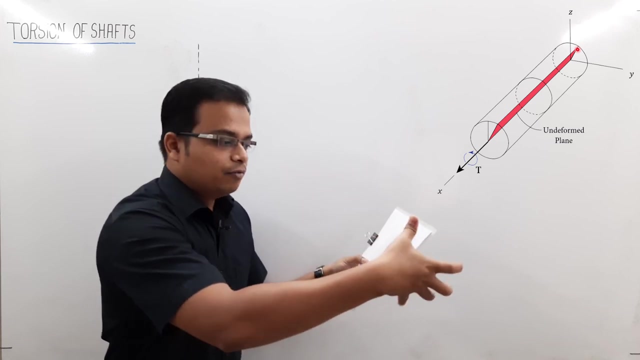 think about it very interesting, let me tell you so. originally it's like this: just just take a look at this originally. this is the plane: okay at a certain angle. you see this angle okay to the right, to the right, and according to me this is to the right slightly. now this plane will be deformed. 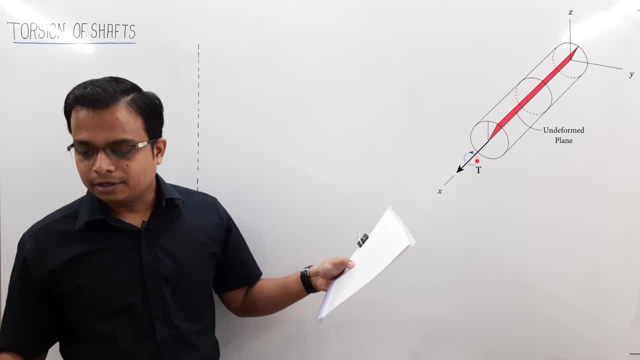 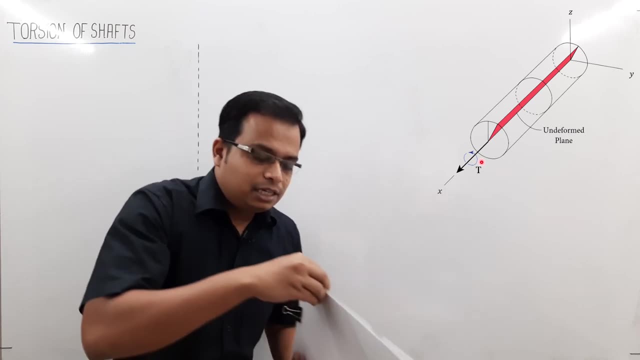 once you apply the torque in this direction, you see this torque. yes, so this is the torque. so what will happen to this red colored plane once the torque is applied? one sec, one sec, one sec. what will happen? this plane, this portion is fixed right, but let's say you are walking along this. 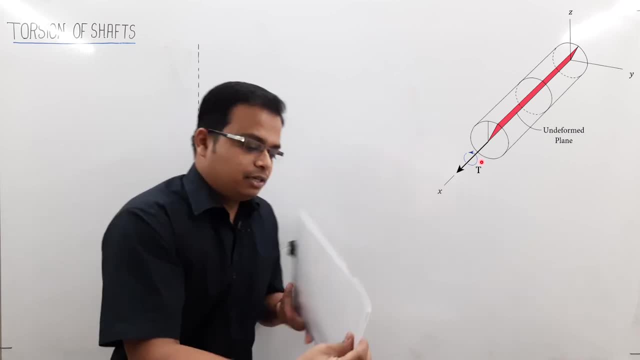 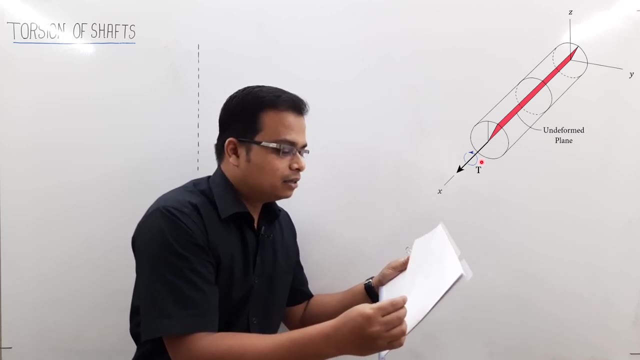 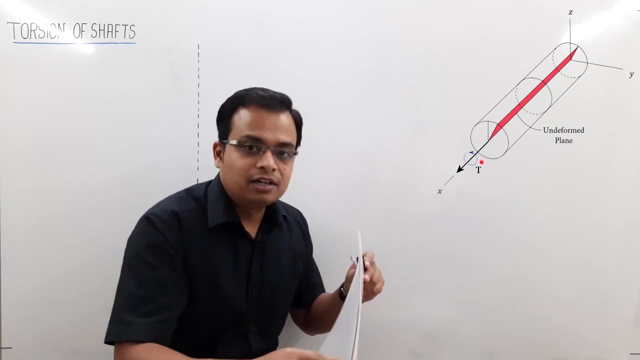 shaft. you are walking along this shaft. what will you see? let me tell you, the plane will now, will now get itself a new orientation. something like this, like this- hope you got my point- and if you walk over this shaft, you will realize that the angle of twist keeps on increasing. from this, 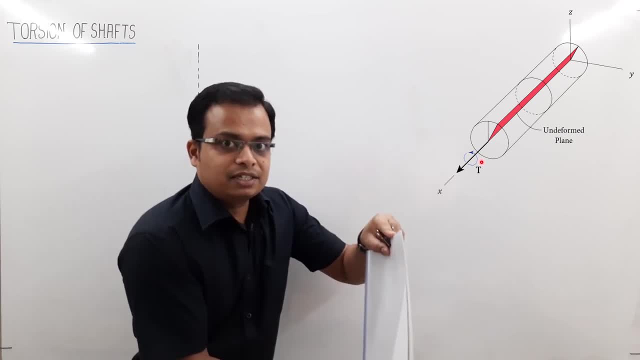 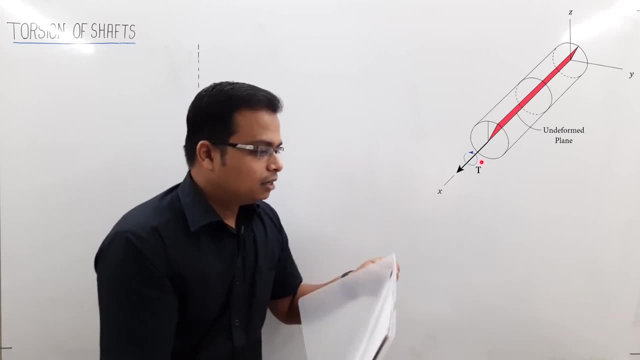 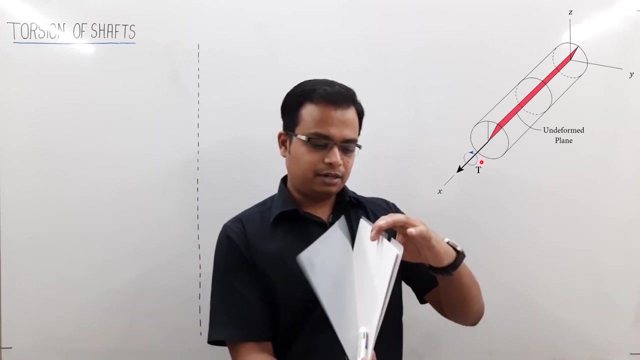 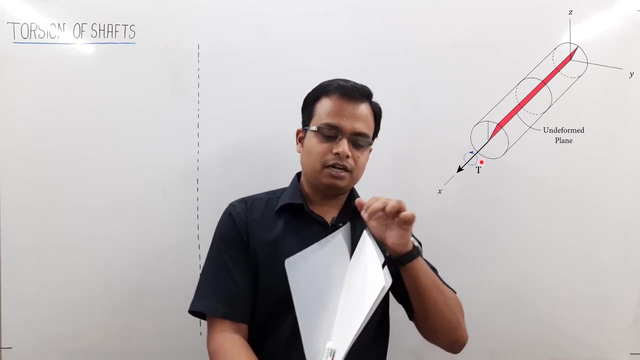 fixed end to this free end. angle of shift keeps on increasing from this fixed end to this free end. very difficult for me. just a second, guys, i can put something over here one sec. yeah, that's better. that's better. take a look, this is okay. yeah, so if you keep walking over this, 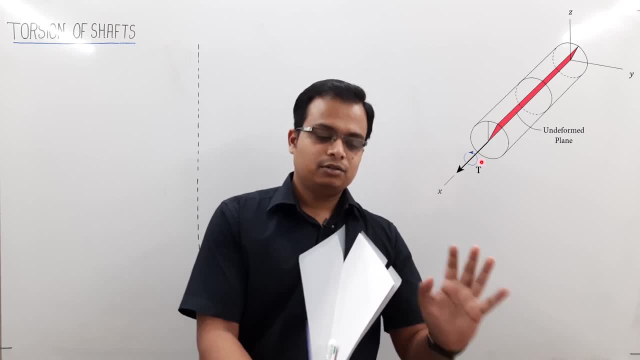 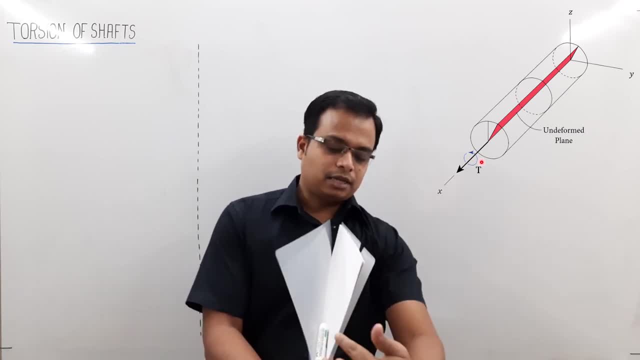 because we are comparing. so if you keep on walking over it, you'll realize this. this angle keeps on, you'll realize this. this angle keeps on increasing this angle of twist this angle. okay. so, if you have increasing this angle of twist this angle, okay. so if you have a line over here and a line over here, 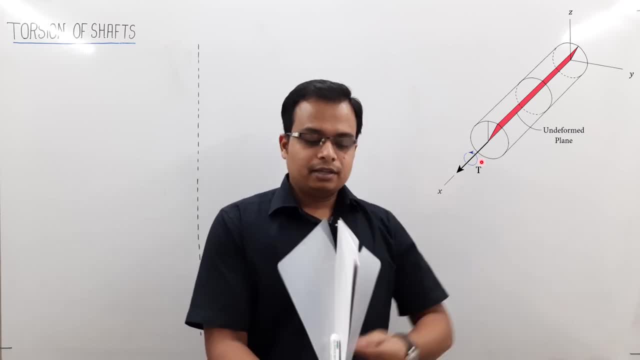 a line over here and a line over here also, there is going to be some angle again if you, if you, if also there is going to be some angle again if you, if you are here, then if you make a line over here, are here, then if you make a line over here and if you make a line over here, then an angle would. 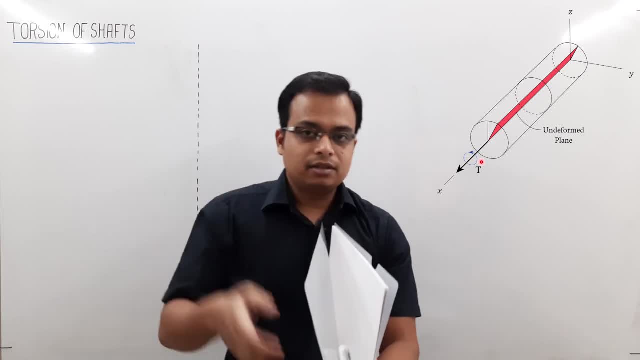 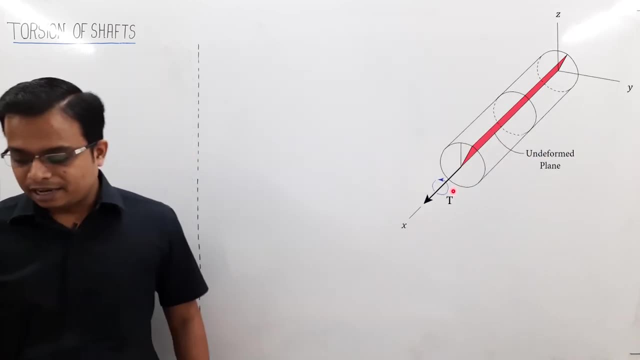 and if you make a line over here, then an angle would again increase. so the angle keeps on increasing, again increase. so the angle keeps on increasing on walking over the shaft. this is something that we we realize. that's the angle of twist. let me show you the plane which is deformed. that is the 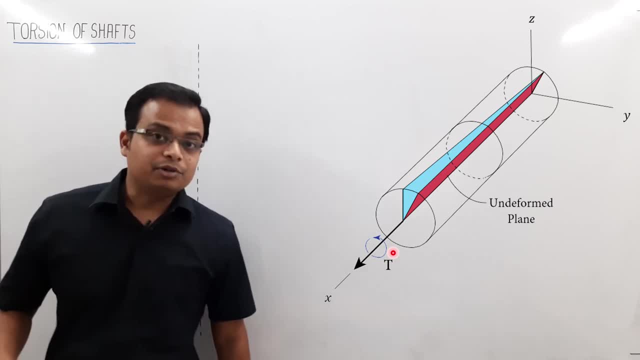 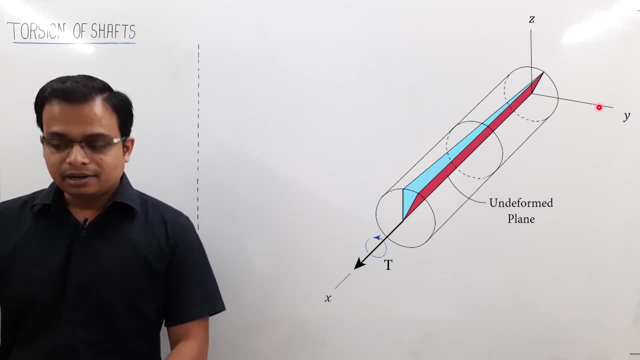 deformed plane. this is exactly what i was trying to demonstrate to you guys. so if you, if you are walking over this shaft right, this angle keeps on increasing and at a certain distance, x. at a certain distance, x, let's say, and this is, by the way, the deformed plane. both red and blue are the 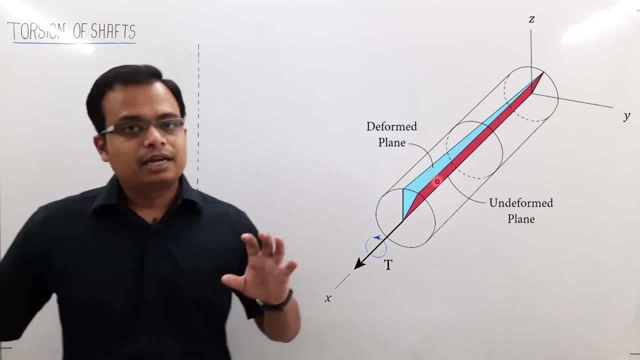 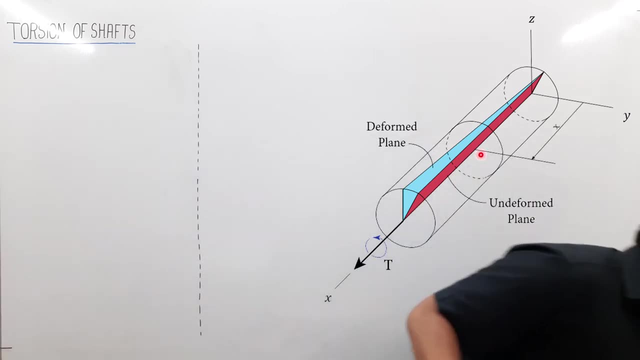 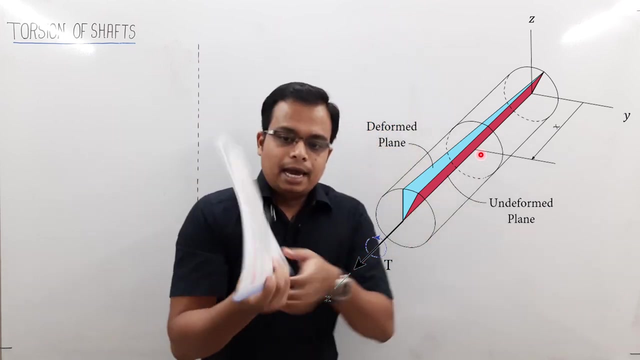 same planes- it is just for the sake of comparison- have kept both of them active now at a certain distance. x. what we'll try to do is we'll try to make two lines once again. that is the shaft. oh, where is the shaft? you can say that this is the shaft, this is the shaft, right, and this is how. 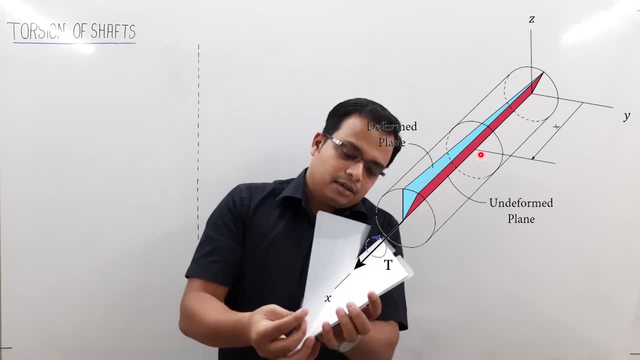 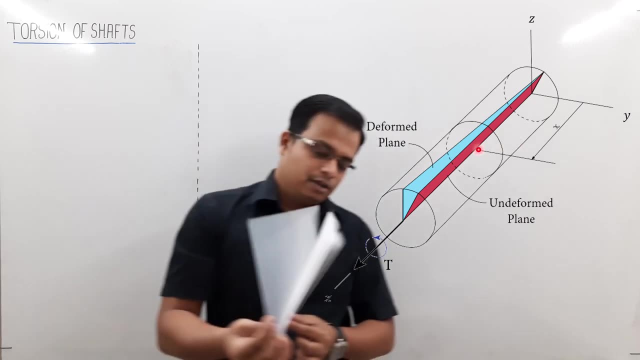 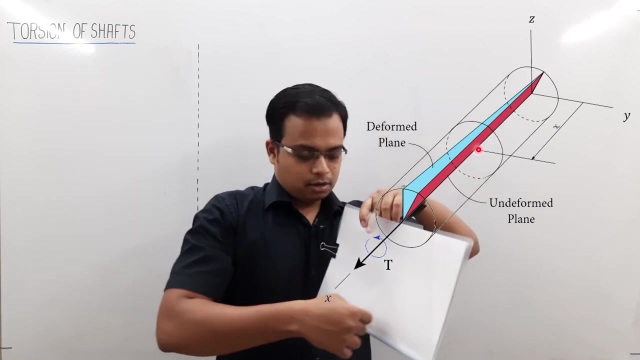 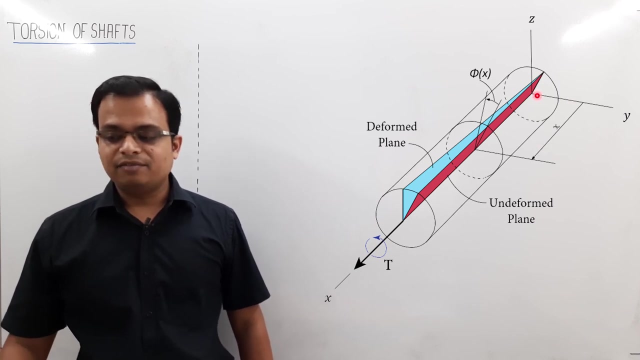 after applying the torque, the planes has changed its orientation. so somewhere here, somewhere here, at this point, at this point, at this point, we are going to be making lines undeformed, same spot deformed. so at a particular distance x from the fixed end, we've got a unique value of the angle of twist that is phi, x. so basically phi. 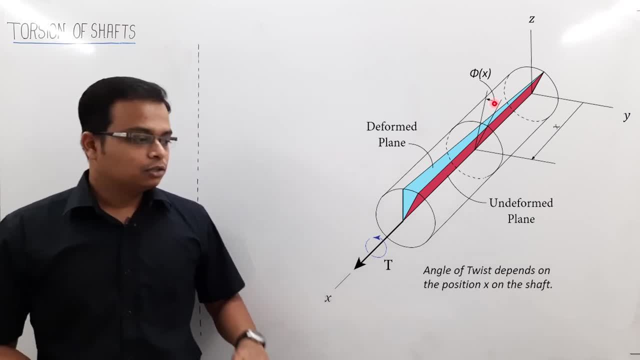 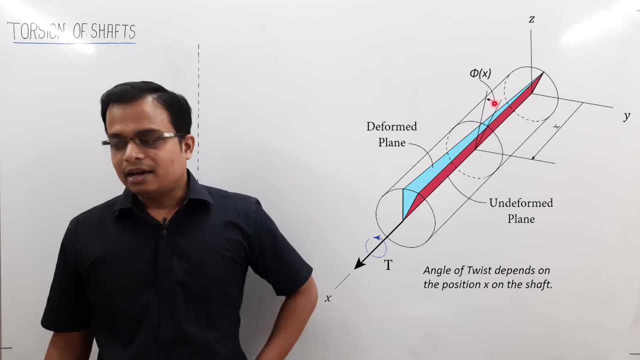 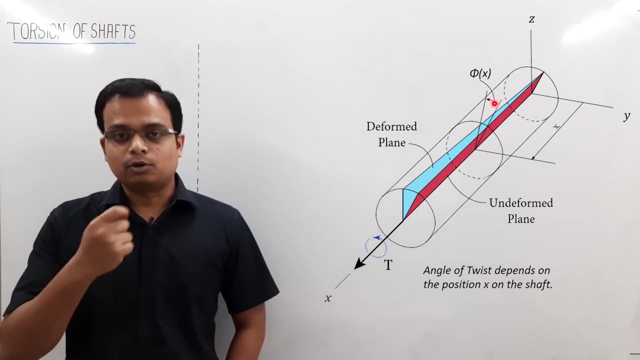 is a function of x, and that is a very important conclusion for all of us so that we can go ahead. hope you got the point right. these things are pretty complex and i'm sure if you read the textbooks, you have to read it over and over again in order to cross grasp it completely. 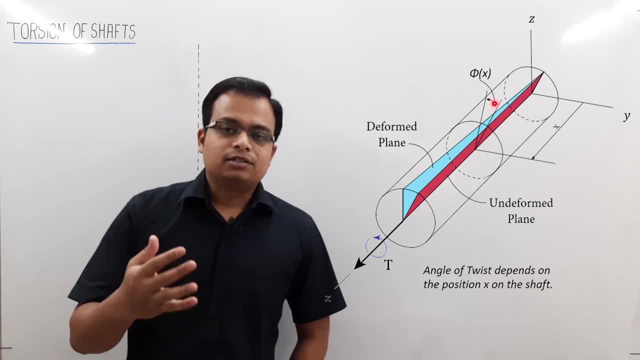 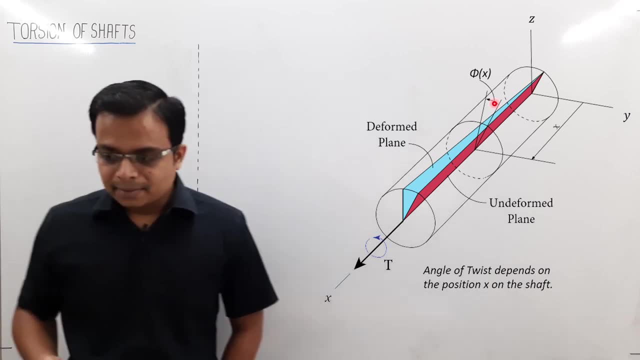 and don't worry, once you see the video, you refer any textbook, all the things will will be absolutely clear to you. make sure you solve the problems, objective, subjective. well, that depends on you and anyway, i'll be taking more classes on torsion and i'll be making you guys solve some really. 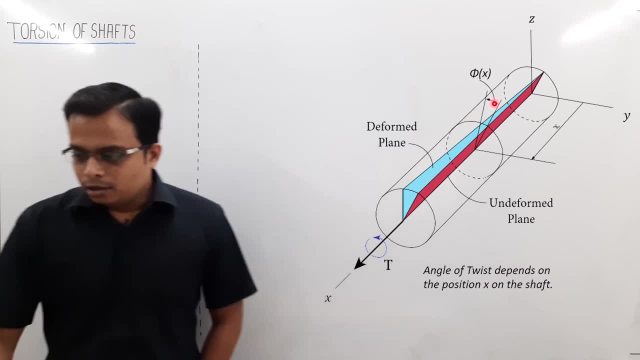 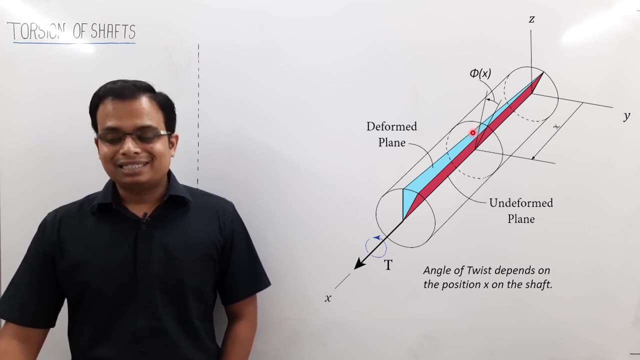 beautiful and tough questions, right? so at a distance of x from the fixed end, you've got this angle of twist. phi x is the angle of twist. that is. phi x is the angle of twist. that is. phi x is the angle of twist, phi. okay, so if you are walking over the shaft, you will realize that this angle over here is more. 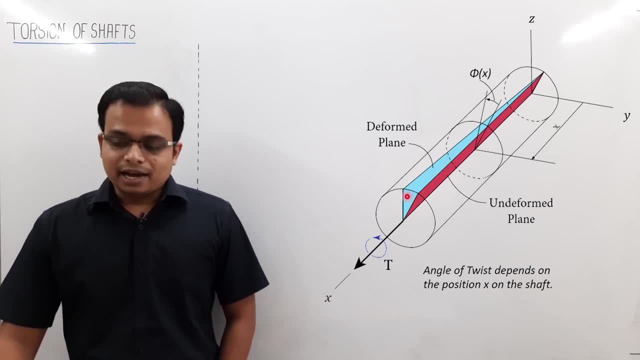 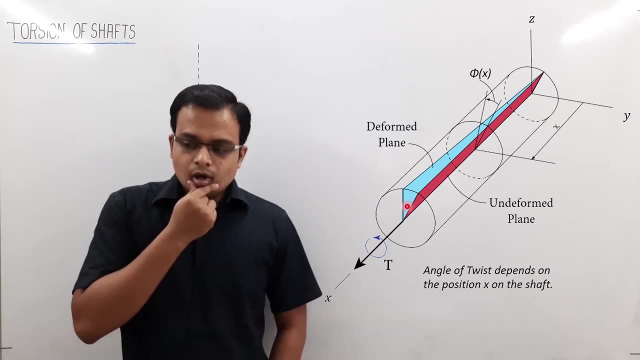 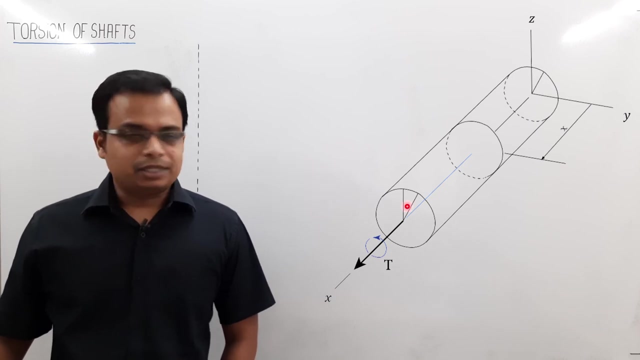 this angle is further more, and the maximum value of the angle of twist is at the free end. that is a conclusion which we can derive from what we have done. lovely, how can we proceed now? just take a look now. what we'll do is again that same same specimen we have. okay, i've. 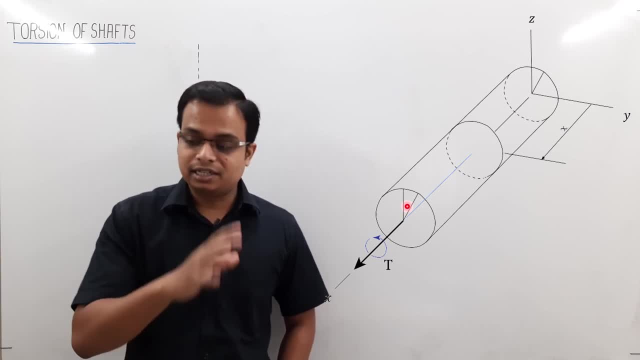 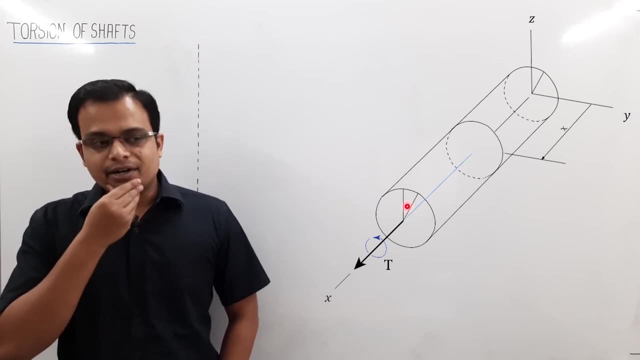 kept it transparent. don't think that this is a skeleton. it is solid, still stolid. so what's going inside family of discs is a cylinder. if you've got a whole lot of discs of a certain amount of thickness, let's say 10 mm thickness, and if you stack them together, 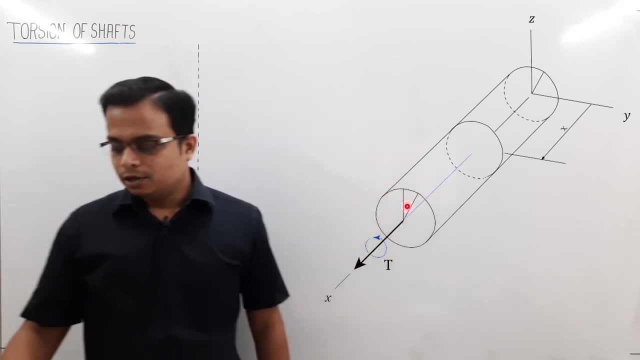 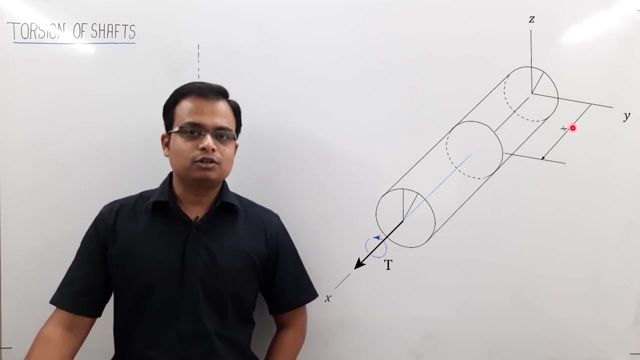 having a common longitudinal axis. what you have is a cylinder. so basically, um, a cylinder is made up of discs. you can say that let us have one. here we go. just take a look at this. this is the cross section. how far is it from the fixed end? it is at a distance of 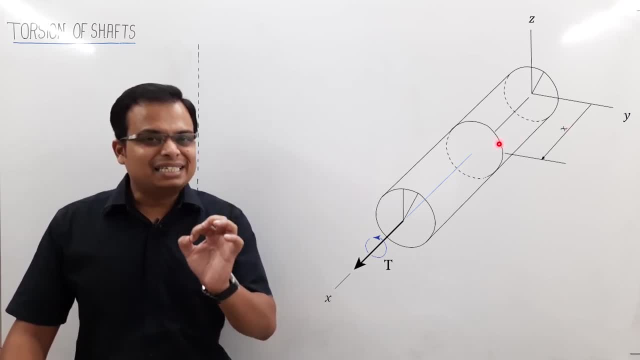 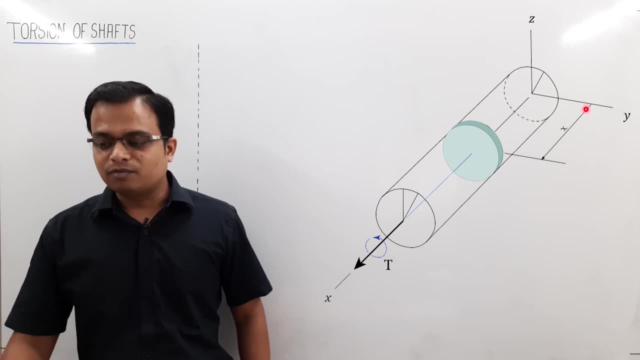 okay. so we have placed the disc in such a manner that the back portion- this one over here is the back portion of the disc- is at a distance of x from the fixed end, okay, and the front portion will be at a larger distance, slightly larger, not more. anyway, inside this disc we'll consider an 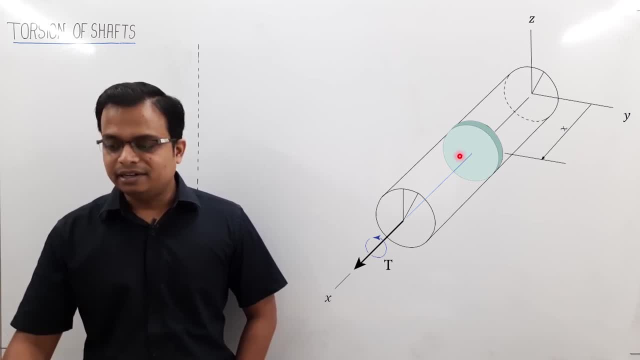 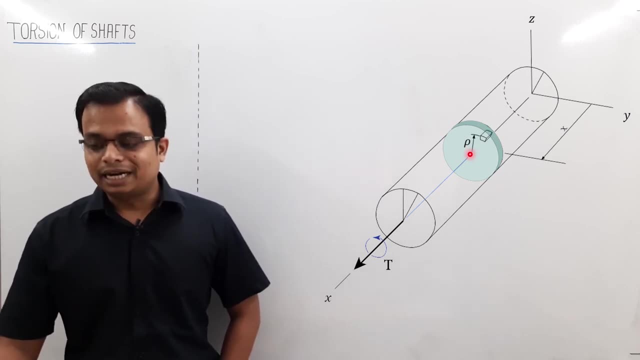 element and this element, once again, let me show you inside the disc. we'll consider an element which is at a distance of, or let's say, which is at a radial distance row from the center of the disc, from the longitudinal axis. here is this element. don't worry, it looks. 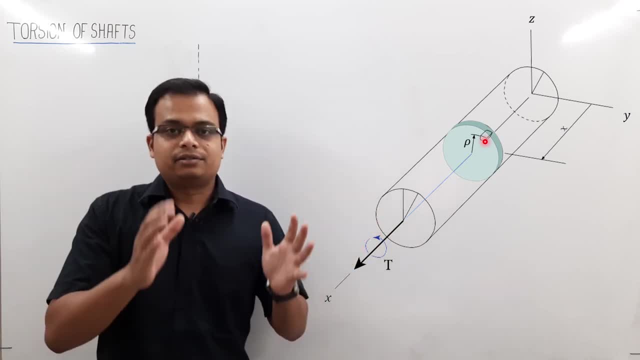 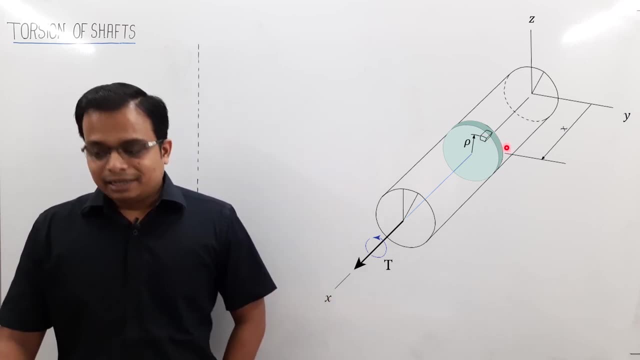 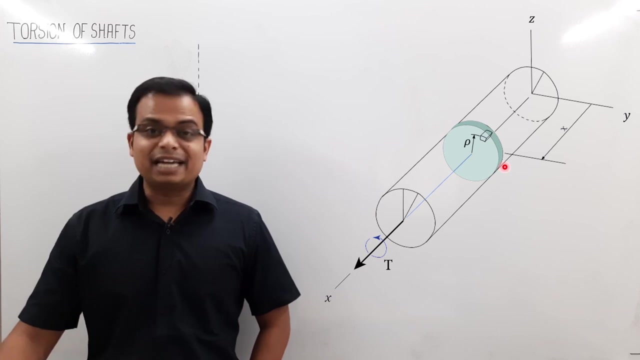 very small. we are going to enlarge it and we are going to analyze it. everything will become very simple now, as i told you, the disc is having a certain amount of thickness, so the back portion of the disc is at a distance x, so the front portion will be at a distance of x plus delta x. 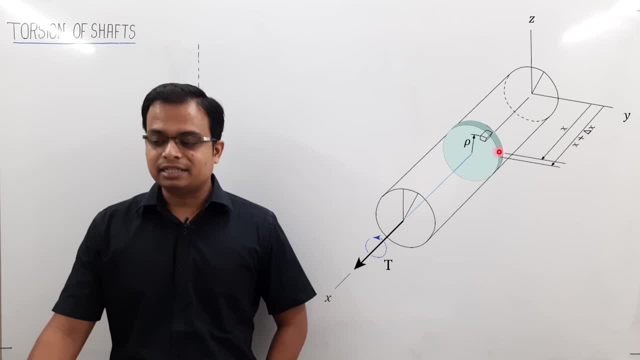 that's it and therefore you can say that. so this disc is having a thickness of x, right, okay. in the same manner, just like the disc is having a front and a back portion, similarly this element is also having a front portion and a back portion. the front portion: 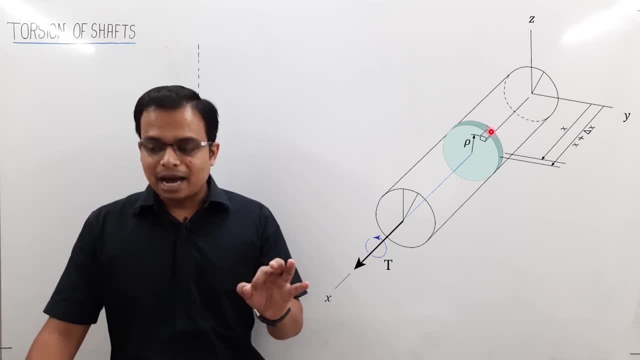 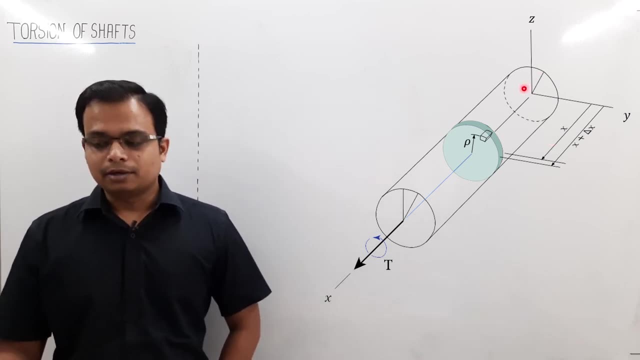 is at a distance of x plus delta x from this fixed end, and the back portion of the element is at a distance of x from the fixed end. this is the friction. let's say: okay, so time to take this session forward and time to enlarge this element and analyze it. so you remember one thing: 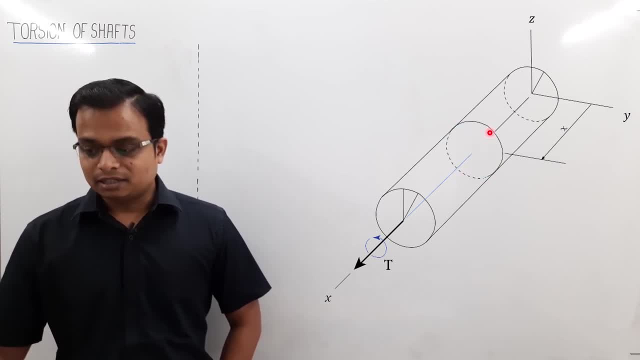 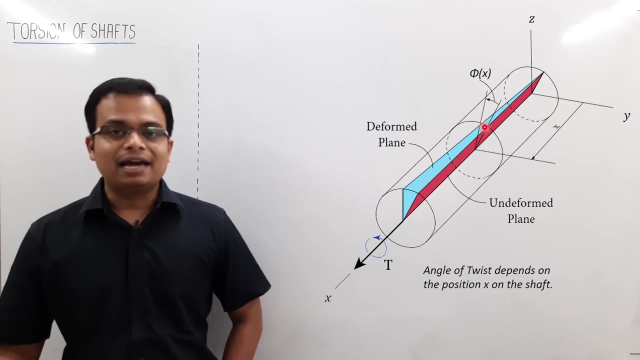 how much was the angle? how much was the angle? let's let me show that once again to you. how much was the angle over here? the angle made was phi x. i showed you in the previous article the angle was phi x and here we have kept a disc, isn't it? we have kept a disc over here, so phi x is the angle. 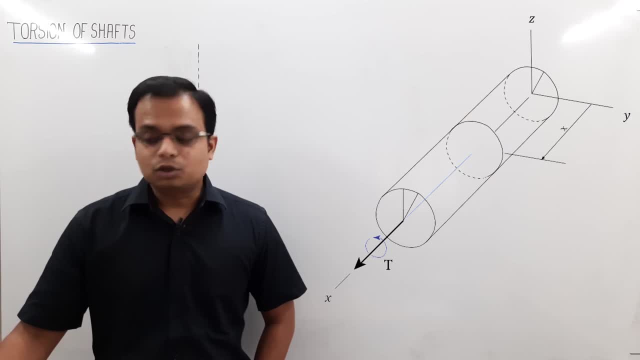 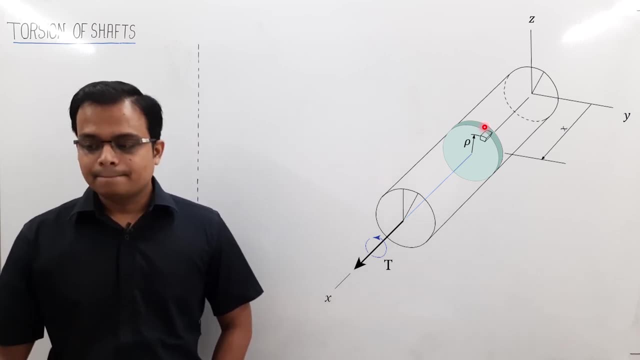 at the back portion. phi x is the angle at the back portion of the disc, okay, or at the back portion of the element. that's it now we can proceed. so there is this element which we will be analyzing at a radial distance row from the center of the disc, or the longitudinal axis, and here we go. let me show that to you. here it is. 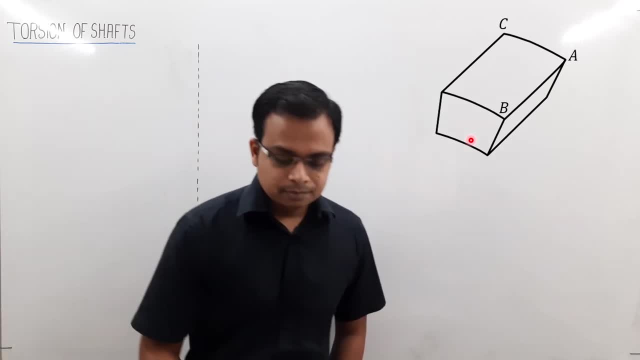 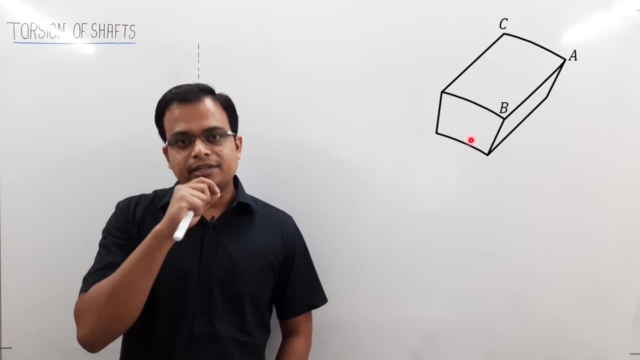 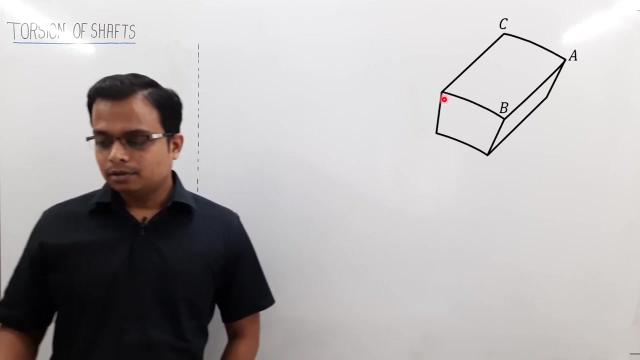 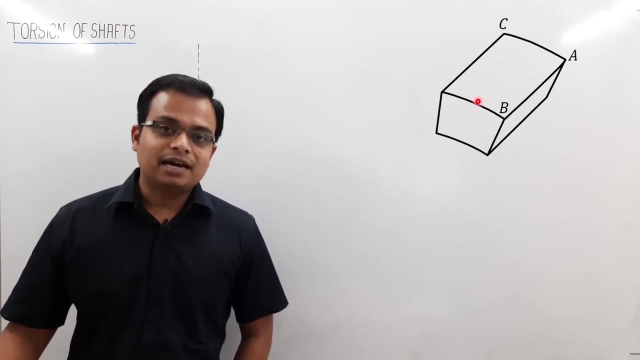 lovely, where is my pen? okay, take a look at this. this element is inside the disc. how far? well, radially, at a distance row from the center of the disc. that's before once the torque is applied. what would happen? well, you'll see some angles. what is the angle? you'll see angle phi. why? because there is strain. why there is strain? because there. 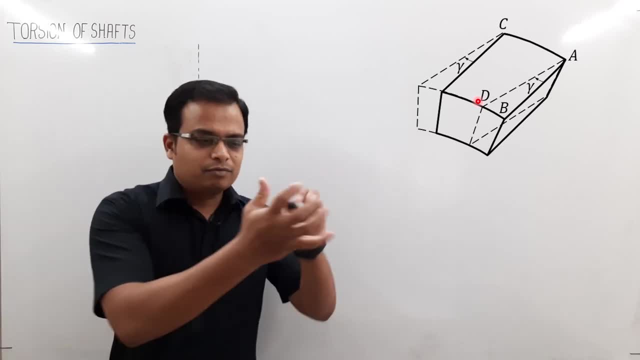 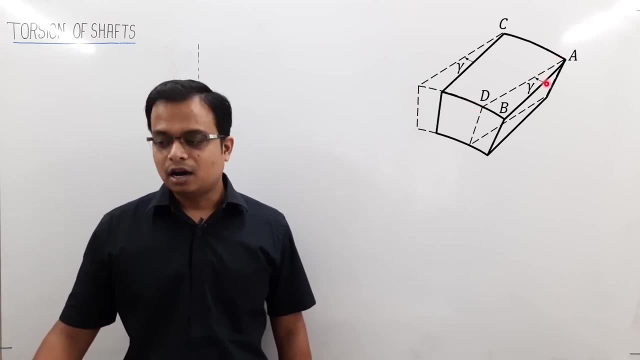 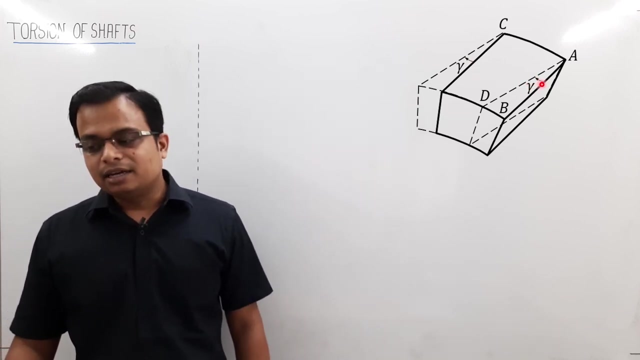 is torque, something like this. this element sort of sort of disoriented itself right. the front face will disorient itself from the back face. how much angle is this? angle, gamma, okay, this, this is extremely small. this angle is extremely small. you can say, and this is the. 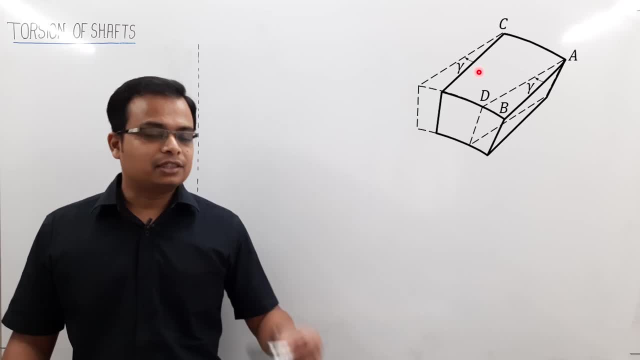 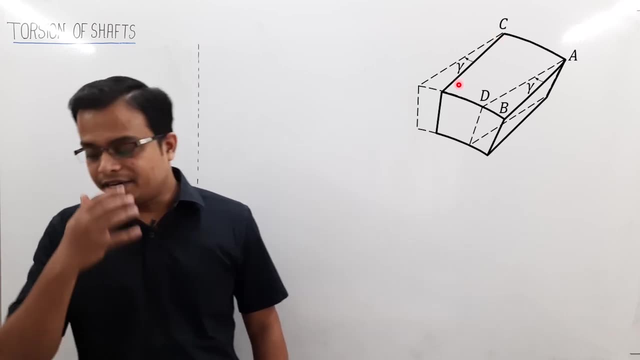 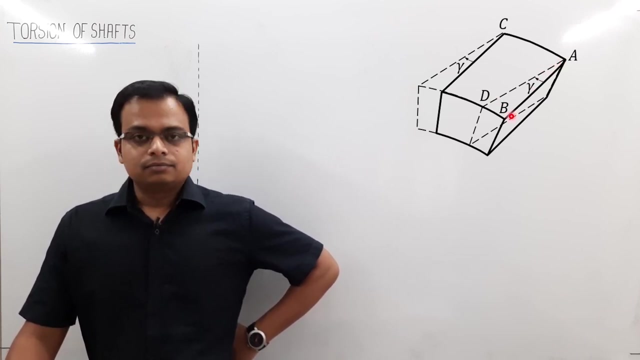 picture that you saw, the red color picture that you i showed you um at the beginning, just five minutes before, i guess. yeah, it was this patch, but we now have to consider this in 3d and we need to analyze it. that's gamma for you. now, ad and ab. they've not changed the. the distortion is very. 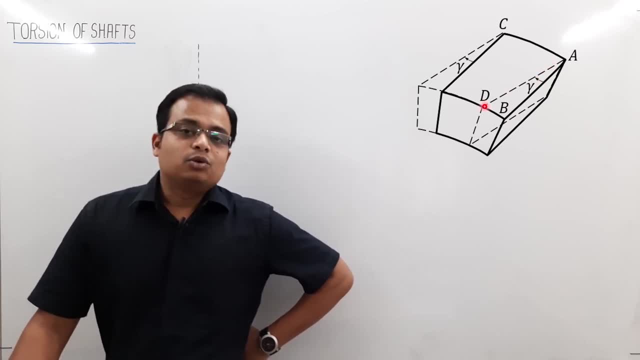 small. so basically, as i told you, linear dimensions don't change, but the angle between adjacent sides change, and here you can see: earlier ac and ab used to have an angle of 90 degree between them, but now ac and ad do not have an angle of 90 degree between them and this indicates the presence of 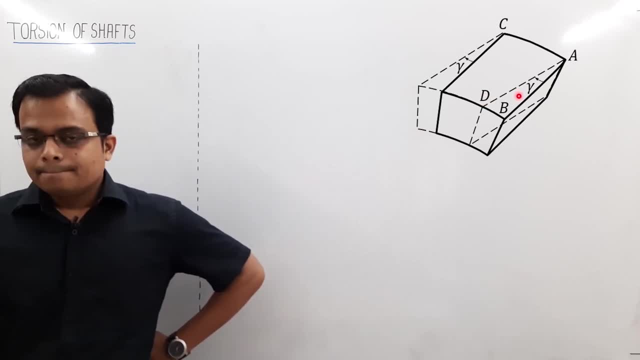 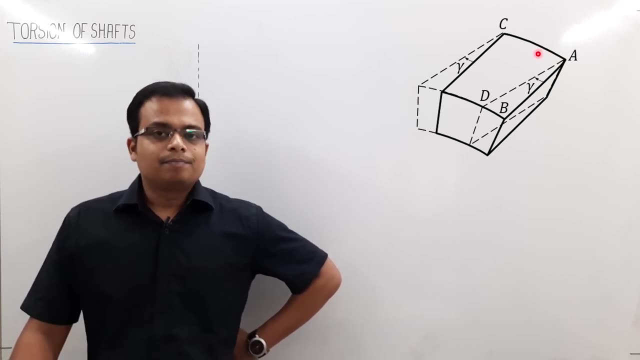 shear strain. okay, one more thing: the back portion. as i told you, the back portion of this element is with the back portion of the disk. okay, was at an angle of 5x. okay, listen to this very carefully. okay, let me, let me. let me make the 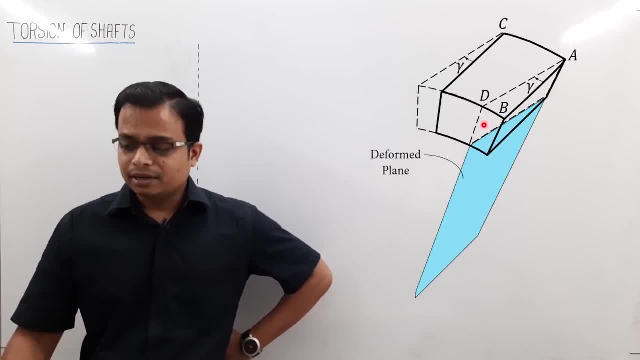 undeformed and deformed planes. this is the deformed plane. okay, it has sort of twisted itself. you can see, though, see this, see this twist, this twist. and this was the undeformed plane. right and back over here, the angle was 5 of x, you should remember this. over here, at the back face, the angle was 5x. 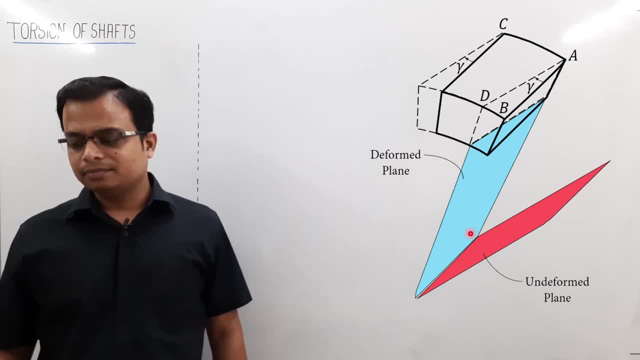 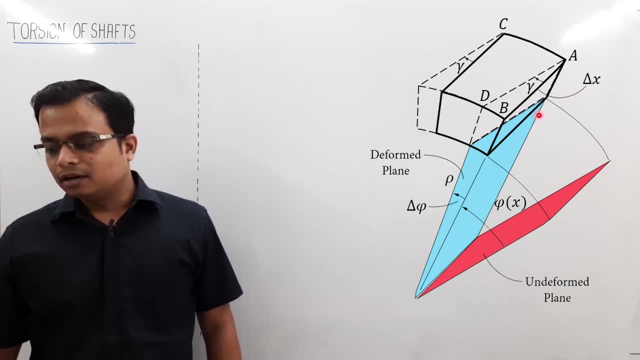 and in the front face the angle would increase by some amount. you can see that. okay, let me put up all those angles, all those dimensions. here we go. this is the back face of the element. how much is the angle? the angle is 5x, i have written it over here. but at the back the element is at an. 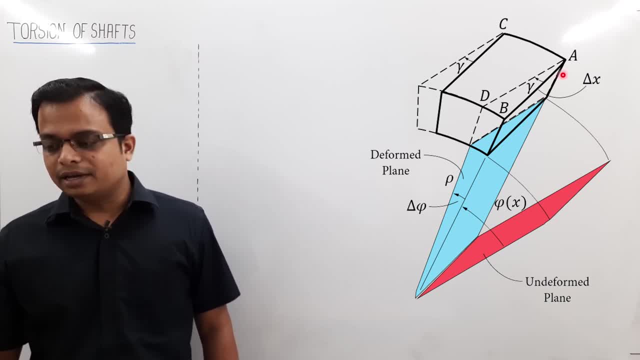 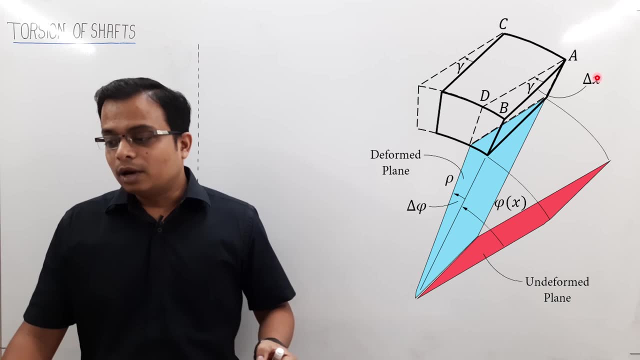 angle of 5x. so at the front, just like over here, you see, the back face was at a distance of x from the fixed end and the front face was at an angle of x plus delta x. so as the back face is at an angle of 5 of x, the front face would be at an angle of 5 of x plus delta. 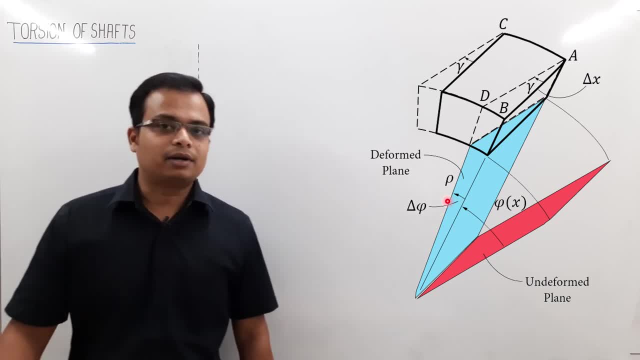 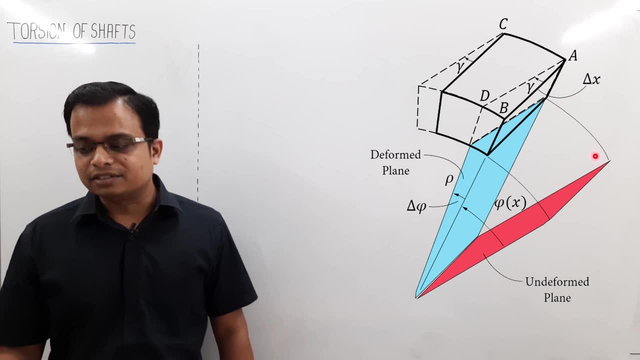 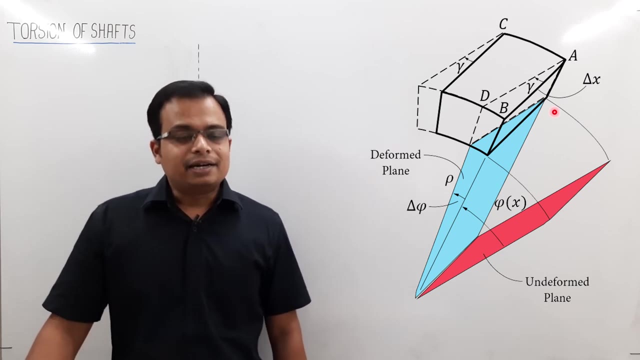 phi. that is the thing which is extremely important and let me reiterate it: the back face at a distance x and at an angle of 5 of x. this angle is nothing but 5x. let me reiterate the front face of the element as well as the disc at an, at a distance of x plus delta x, slightly more. 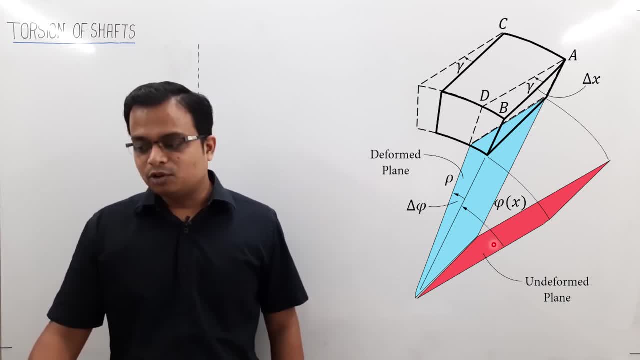 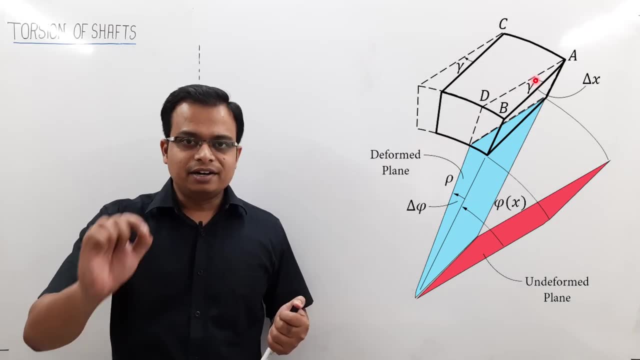 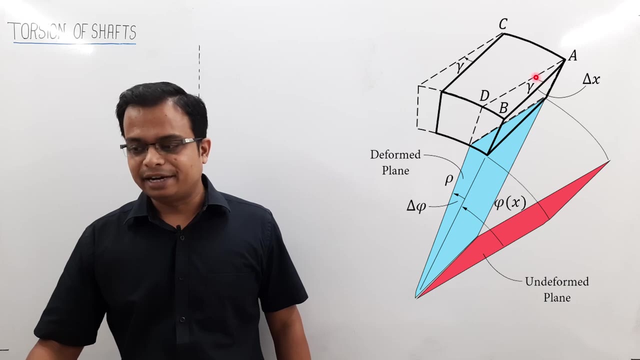 so obviously, because of the twist, the front face would be at an angle of 5x plus delta phi. that's learned till now. let us take this analysis further, to the next level. watch what is the angle subtended gamma. gamma happens to be a part of this triangle a, b, d. right now, this, this angle. 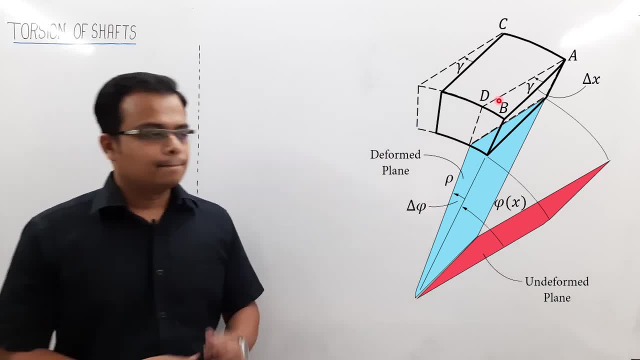 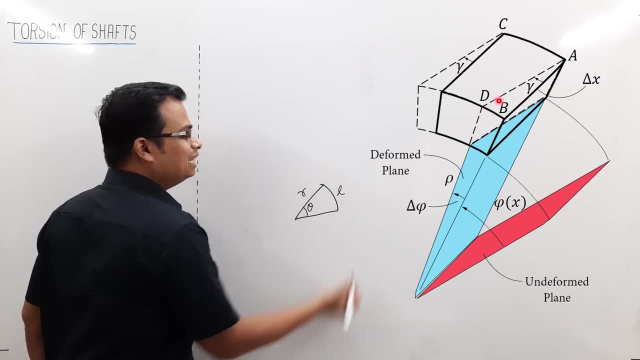 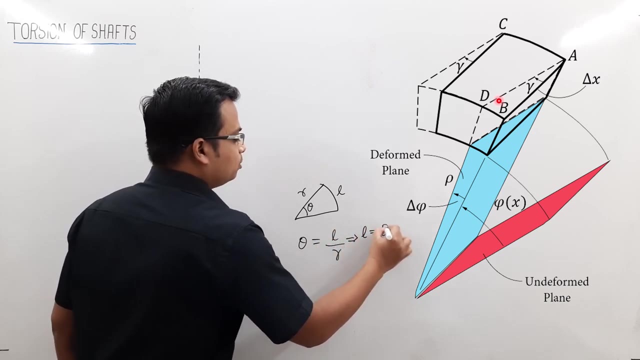 gamma is extremely small. let me reiterate, okay, so i'm sure you must have heard about this relationship. this is angle theta, this is radius r and this is arc length l, so they are related by this formula. radius, or you can say, l, is equal to theta multiplied by radius. that is exactly what we'll 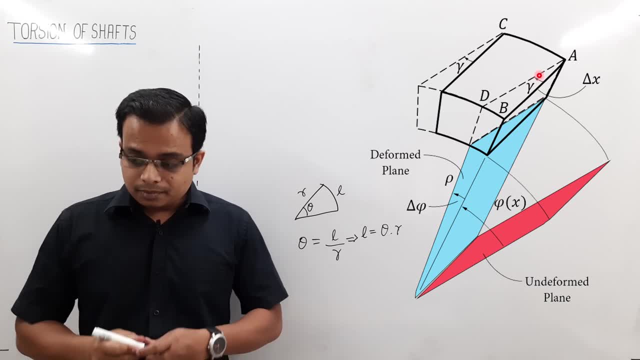 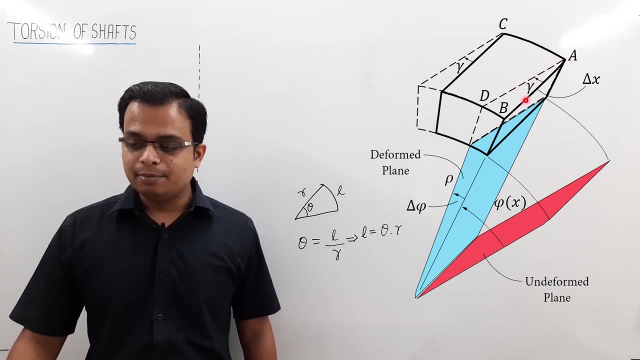 use linear dimensions of ad and ab. they are same. what's changed is their orientation. okay, so you can assume this ad and ab as the radius which whose magnitude is equal to delta x. right, all right. so gamma multiplied by delta x will give you the arc length db. here we go. arc length db. 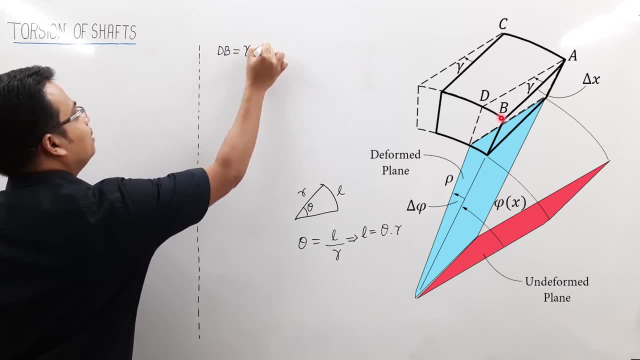 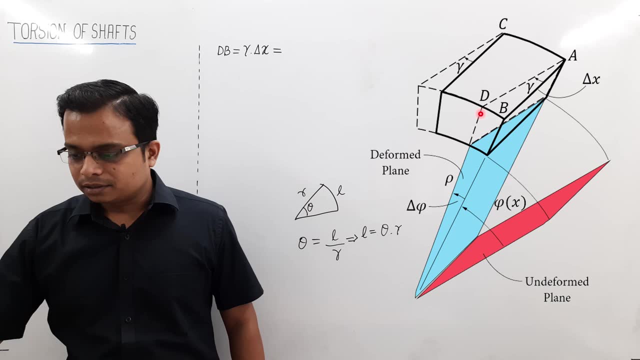 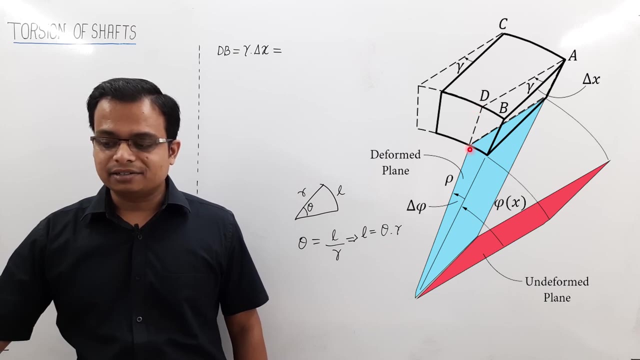 is equal to gamma multiplied by delta x. there is one more way of expressing this db and it can be written from this. you see this: this radius is rho. from this point over here until you reach d, this radius is represented by rho and the angle over here is delta phi. so rho radius multiplied by. 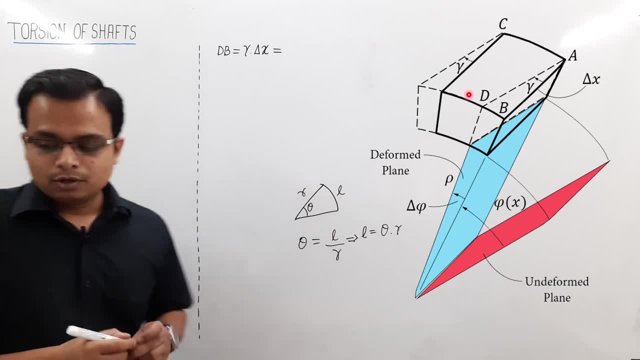 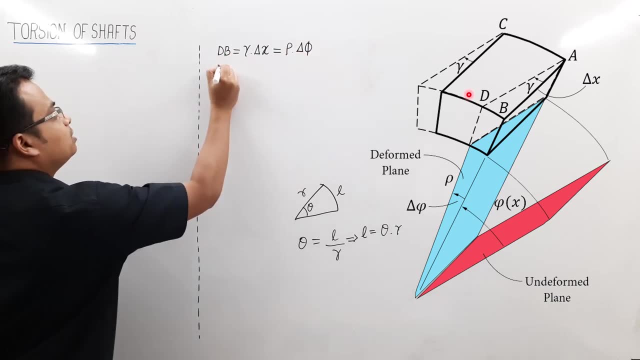 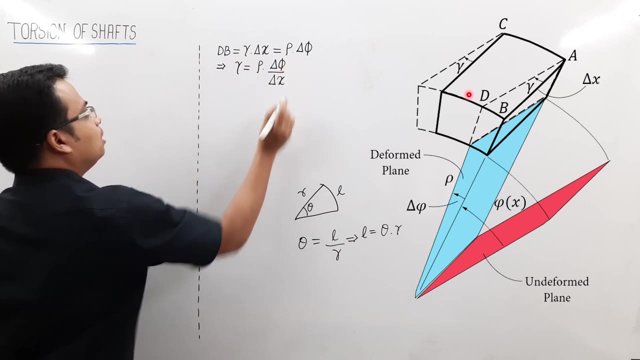 this angle. delta phi will give you again this db: rho delta phi. what is this? rho delta phi, and the better way of expressing this is going to be: gamma is equal to rho times of del phi over del X. lovely, what is this? this is nothing but a ratio, and let we reiterate: 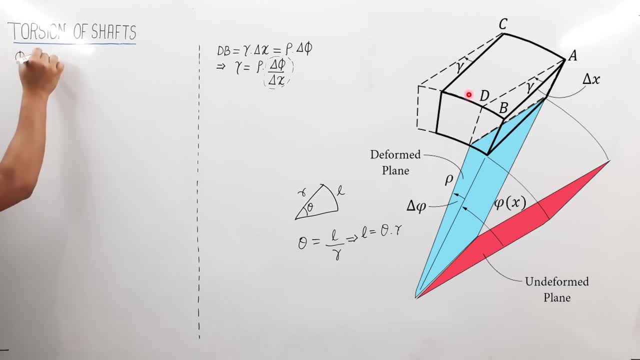 Phi whenever you see something as Phi, Phi is nothing but the angle of twist. okay, let me write this. secondly, you've got X. what is X? X is but the position of cross section. So we are talking about the element. So element has a back. 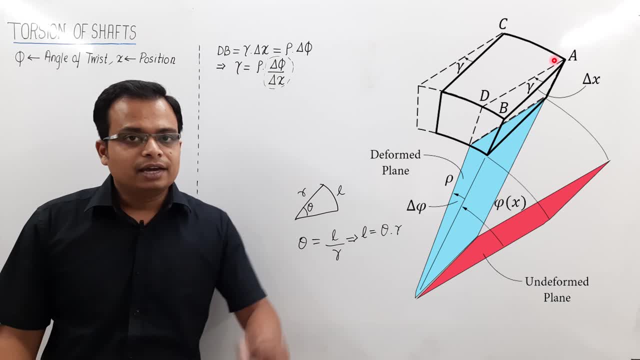 face and a front face. The back face is at a distance of x from the fixed end of the shaft, while the front face of the element is at a distance of x plus delta x from the fixed end, and that is why this element is having a thickness of delta x. You know this, Okay, position. 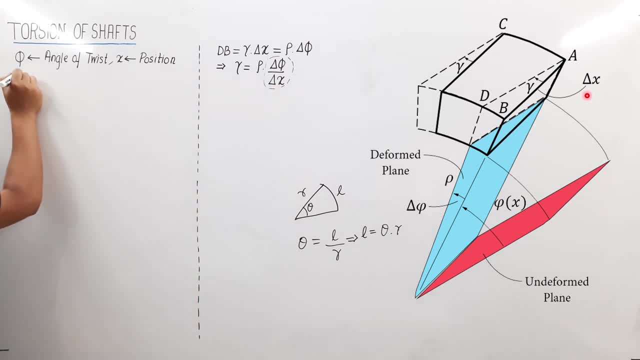 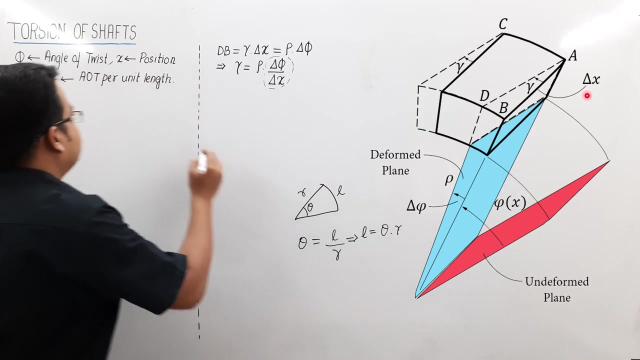 I am introducing a new term over here: Theta. Theta is nothing but delta phi over delta x, and delta phi by delta x is nothing but the angle of twist per unit. Lovely Done, That's done. Okay, So you can essentially write your first relationship. 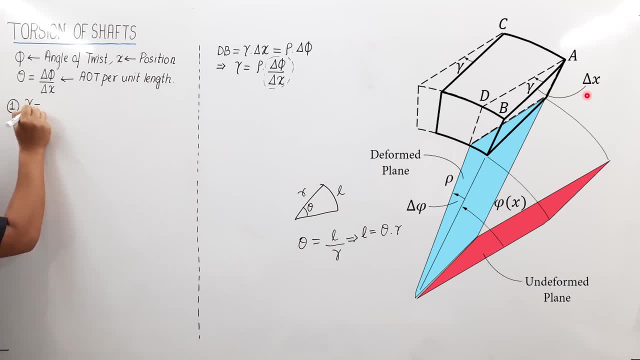 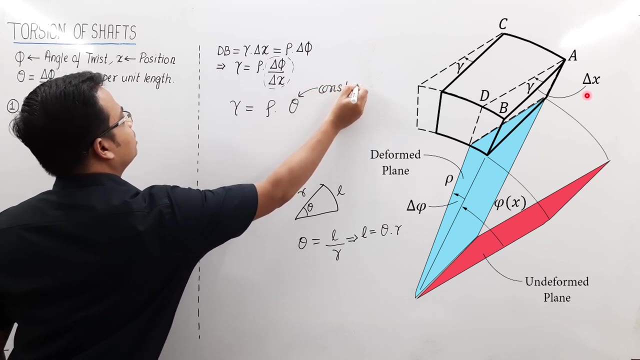 that is, a gamma is equal to rho times of theta. This is a very powerful equation and let me tell you why. See this: Gamma is equal to rho times of theta. What is theta For each and every element on the disk? it is constant. Theta remains same. This ratio, delta phi by delta x, For any element. 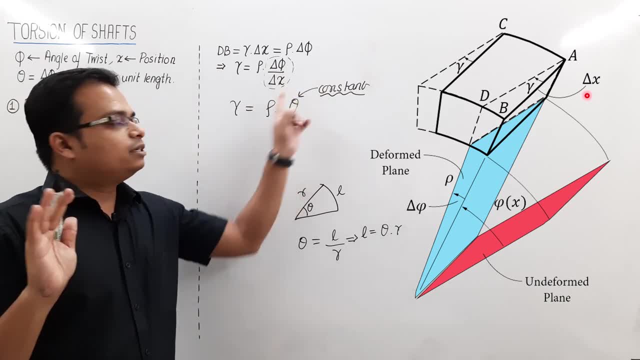 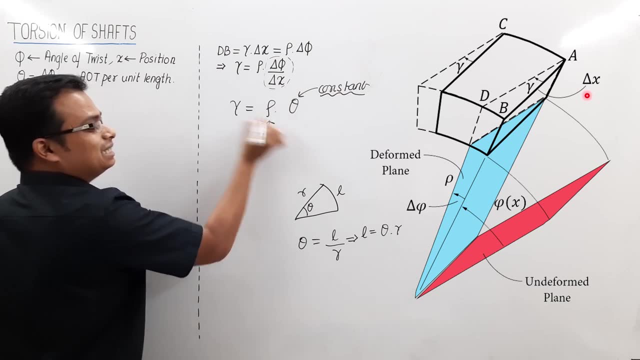 at any radial distance on the disk, it is going to remain same. Okay, I will show you in a figure also. So if rho increases, if the radial distance increases, it is constant. So, if rho increases, it is constant. So if rho increases, if the 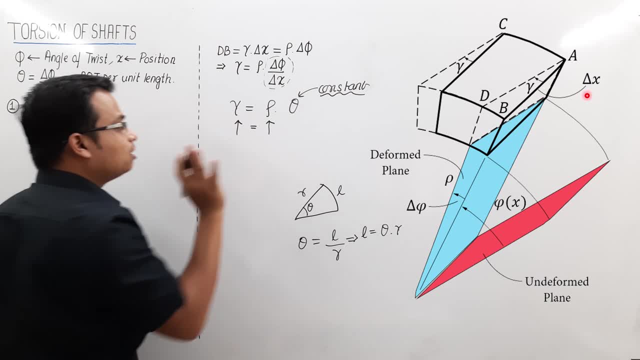 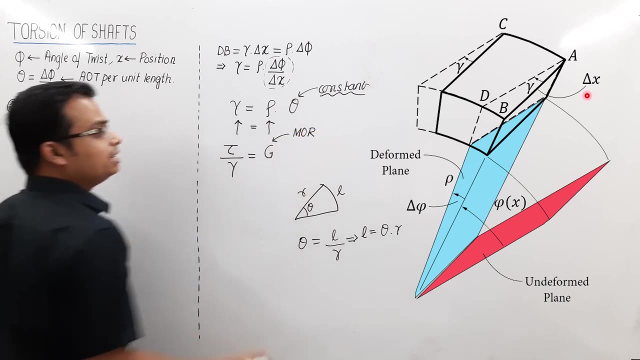 radius increases, then gamma would also increase. This is a very powerful equation. There are different versions. Now you know shear stress and shear strain. This ratio is g. What is g? Some people also write it as c, Modulus of rigidity. Once again, modulus of rigidity. 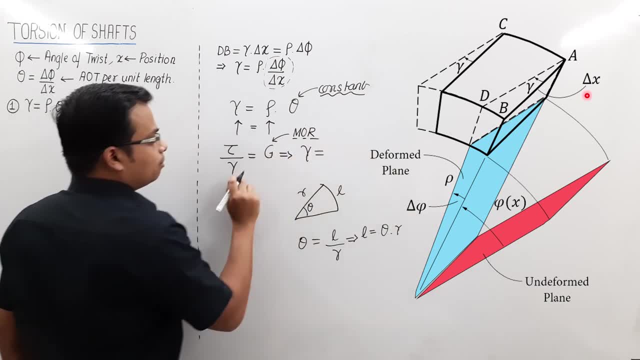 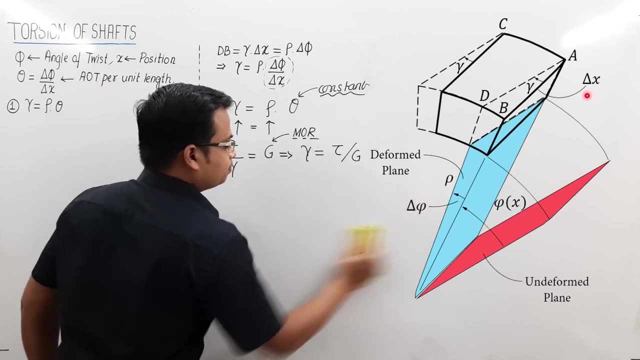 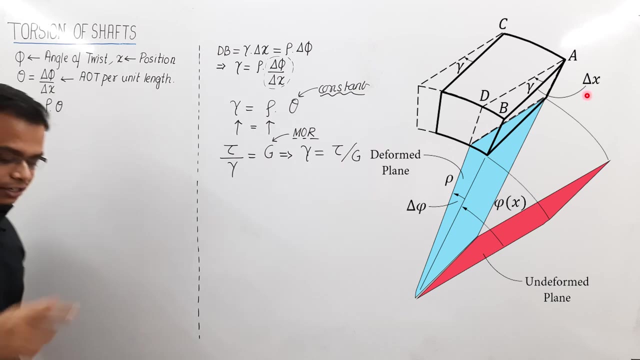 So what you can do is gamma equals tau over g. You can replace this. Let me come to the point Straight away. Just like this relationship of shear strain, with this angle of twist per unit length, we can have the same relationship for shear stress, As I told you, if the radial distance 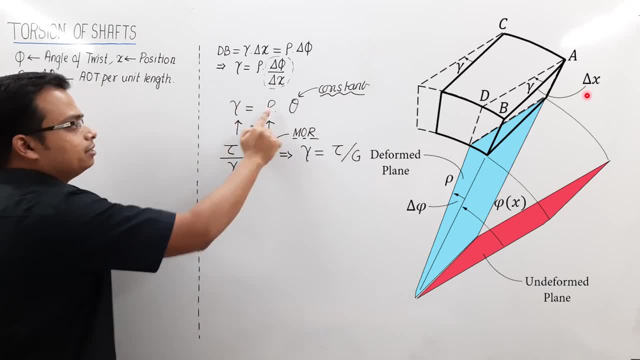 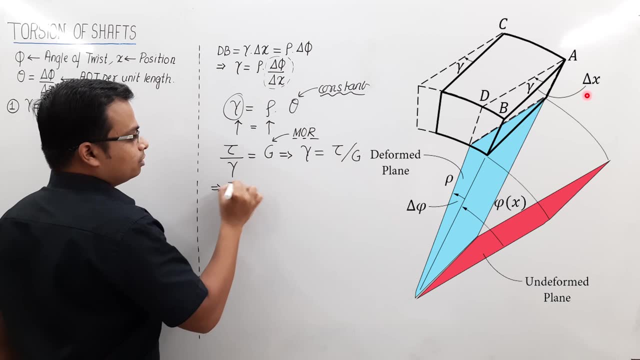 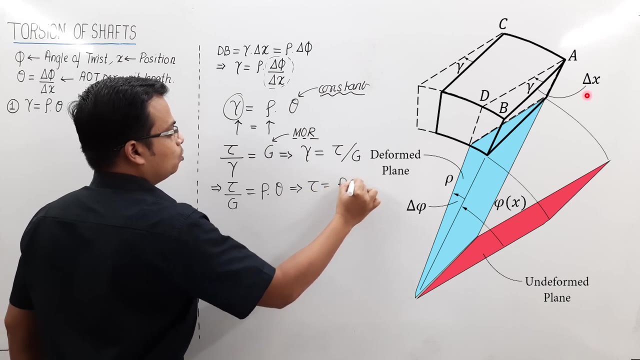 increases, shear strain increases. Please note it down. Radial distance increases. shear strain increases in the same fashion. Let me replace this gamma with this gamma with tau over g is equal to rho theta. Let me write this in a better fashion: Tau is equal to rho theta, and. 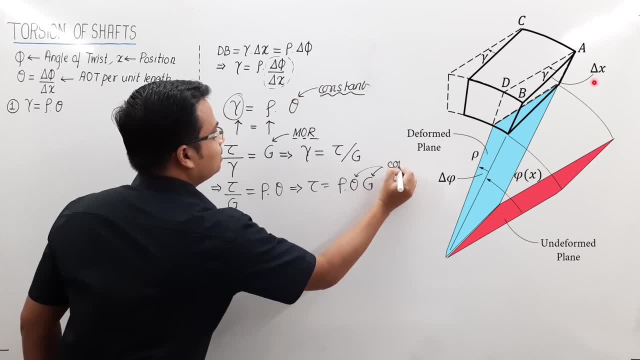 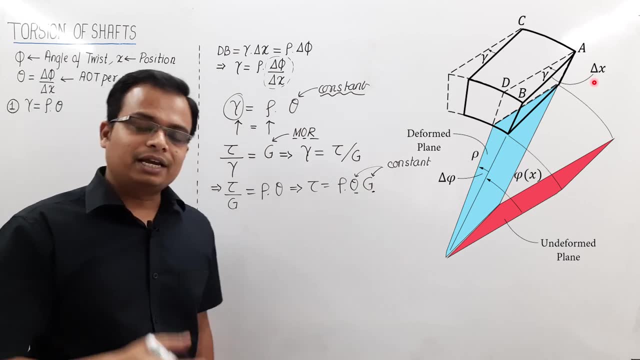 g. So theta and g, What are they? These are constants. For any fixed material of the shaft, g is constant Theta angle of twist per unit length. for any element. it is going to be same Right. So what is going to change? Rho is going to change. So if rho increases, 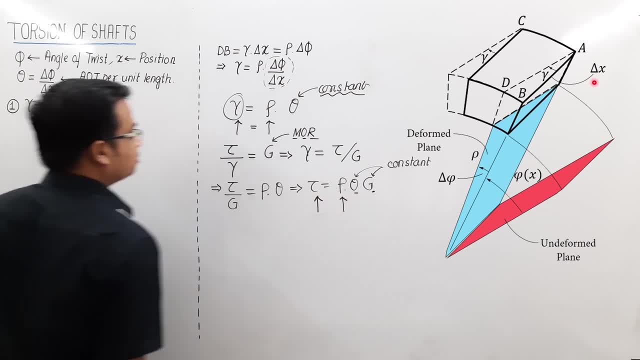 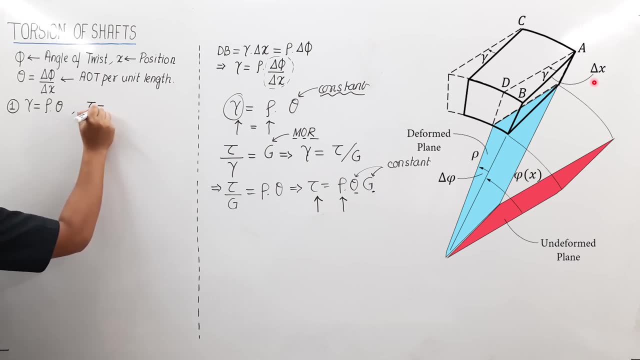 angle of, not angle, but the shear stress also increases. Another important relationship which I am going to be using. Let me write it: Tacoma shear stress is equal to rho g theta. Alright, How can we go ahead now? That is very important. Let us try to compare. 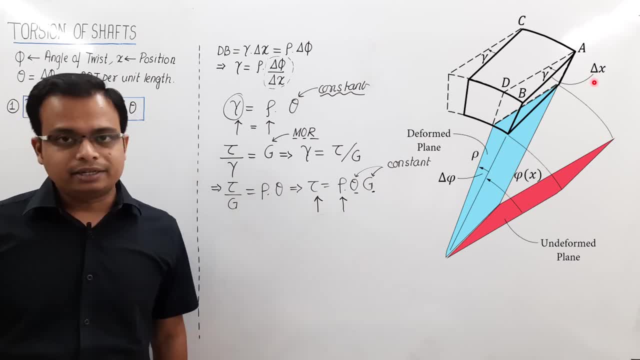 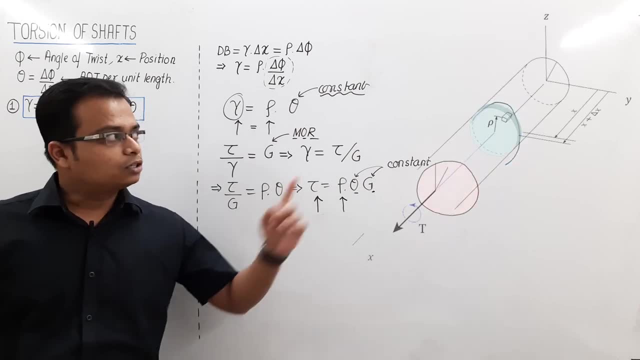 two elements now. Okay, Let us try to have two elements. on the descent, Let us try to make a comparison between shear strain, Let us try to make a comparison between shear stress. and here we go. Watch this Same figure Back, face, front face. added distance x and added distance of x. 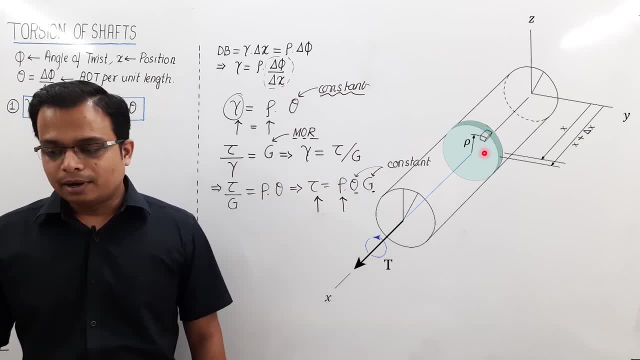 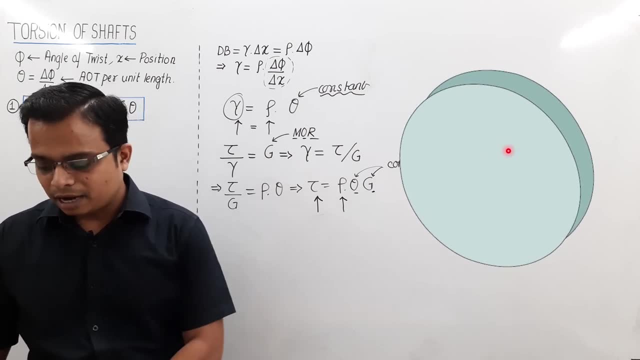 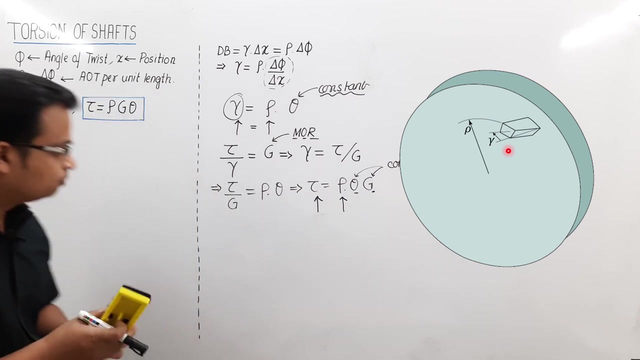 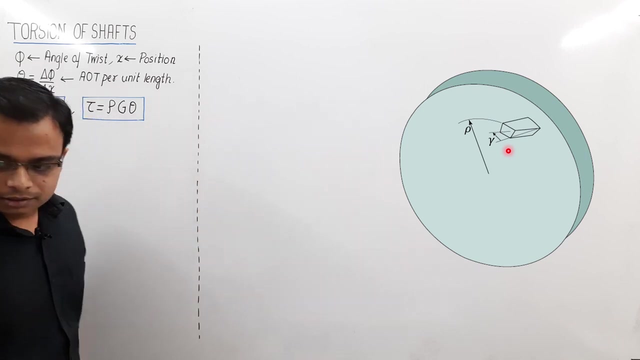 plus delta x, Thickness being delta x. Let us now enlarge this disc and let us have two elements. The first element which I am going to have is at a radial distance, rho like this. Let us do this. Watch This is going to be super, super interesting. Watch this. So we already know. 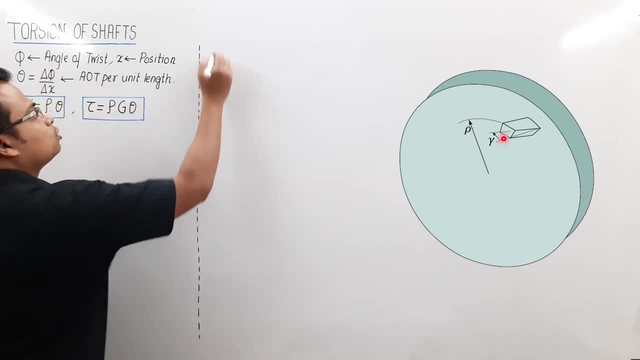 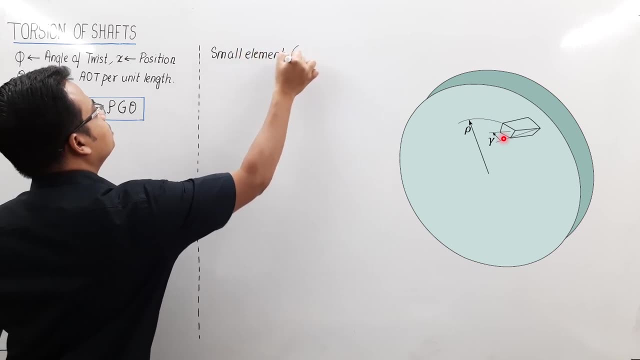 about this element. We know everything. Okay, This is the small element. What Small element? How far is this element From the center? So it is at a distance of, or a radial distance of, rho. So you have this relationship, Gamma. what is the shear strain? 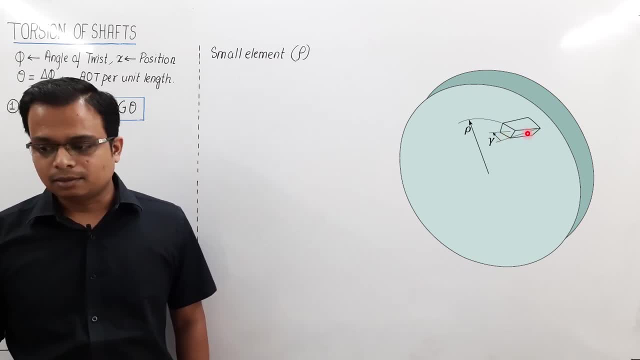 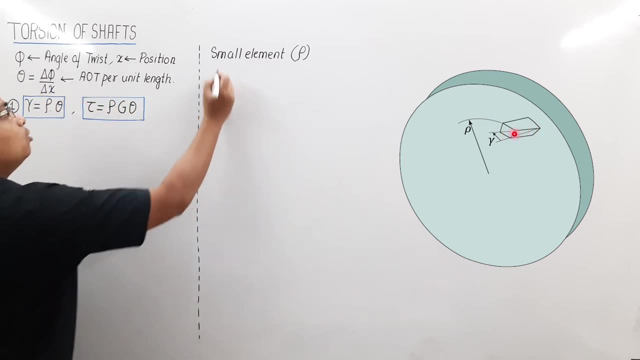 It is gamma. You can clearly see. Okay, The back face has, the front face has turned by an angle of gamma with respect to the back face. That is gamma. So you already know, at a radial distance, rho you have this shear strain. gamma is equal to rho times of theta. Theta is going to be. 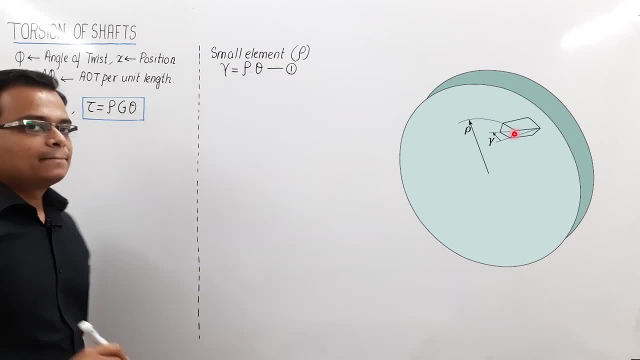 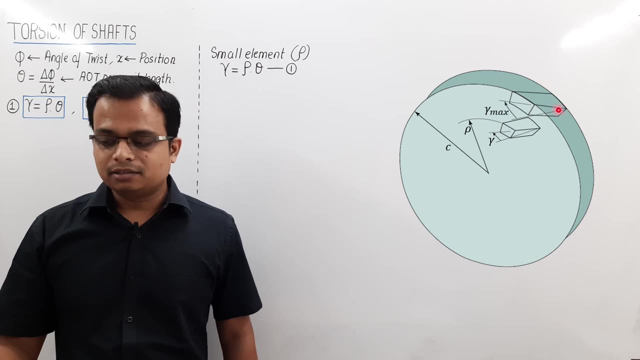 same. Let us say this is our equation number one. Let us have another element, a slightly bigger element. Thickness will remain same Here. this thickness will remain same. Look for both the elements. if you look at it from the front, you will realize that angle d5. 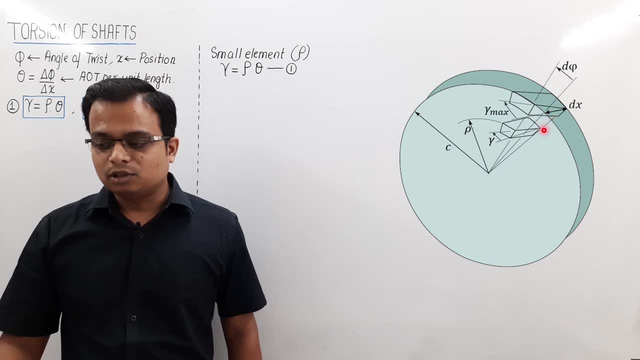 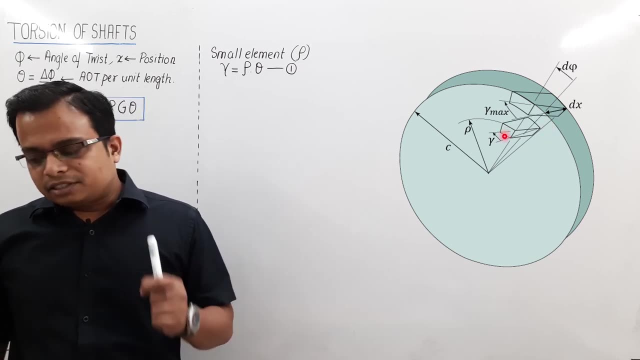 for both the elements is same and this thickness of the element is also same. That is dx, Delta x or dx, let us say They are extremely small, infinitesimally small. The thing that is changing is that, at a radial distance, rho- the shear strain is gamma and at a radial distance c, the shear 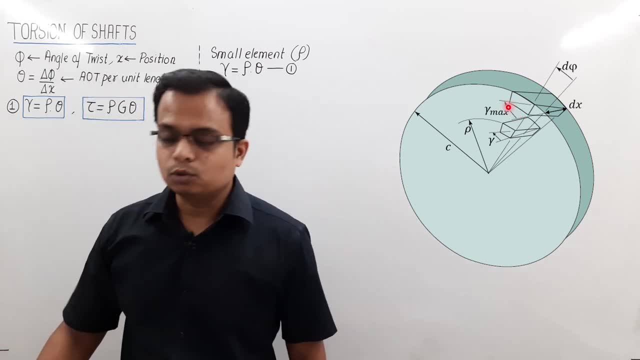 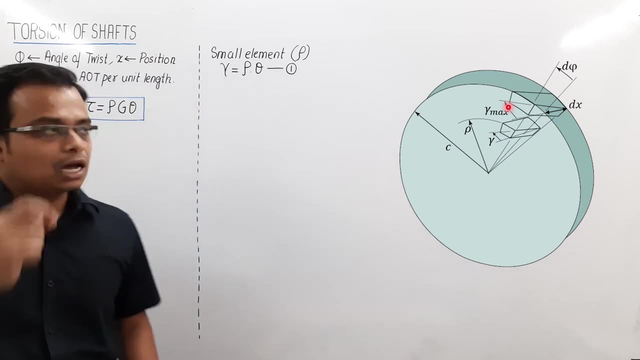 strain is highest or maximum, That is, gamma max. So what we wish to do is develop some kind of relationship between both maximum strain and the strain at any radial distance, rho. How can that be done? So for the larger element, big element, let us say small element and let us say large. 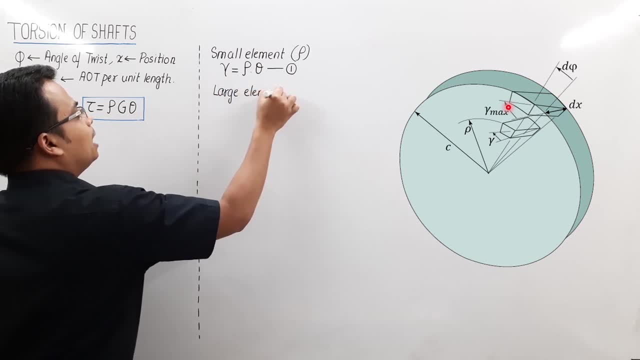 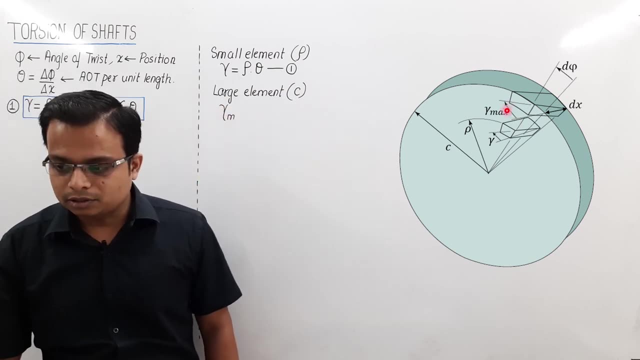 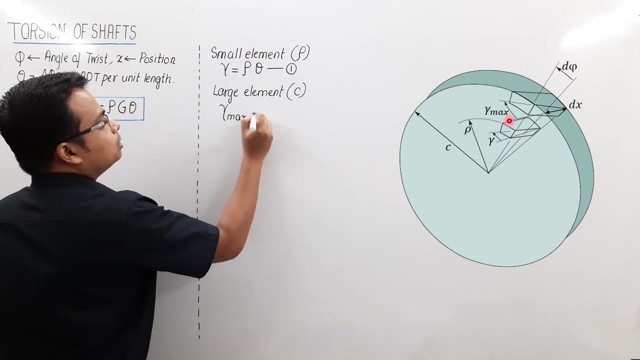 element, Large element, And that large element happens to be at a radial distance c, So shear strain is also maximum. You can see this. Here we go. This is maximum shear strain. This angle is more than this one, So maximum shear strain is equal to radial distance, that is c and theta is. 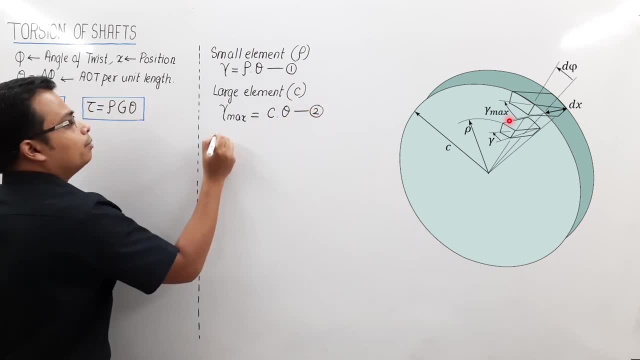 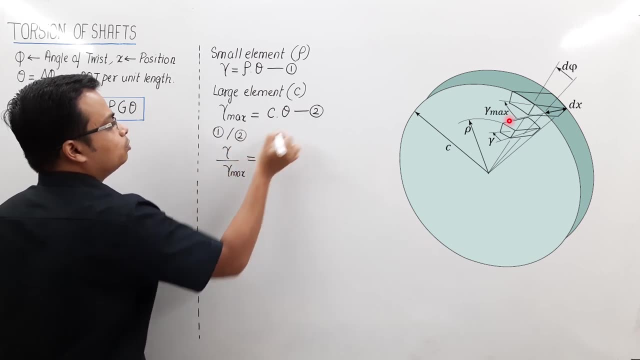 going to stay same, Does not matter which element you are talking about. Now, when you divide these two equations, you have this relationship: gamma divided by gamma max is equal to theta, and theta will cancel each other out. Rho divided by c. If I can write this in a better fashion, I can also: 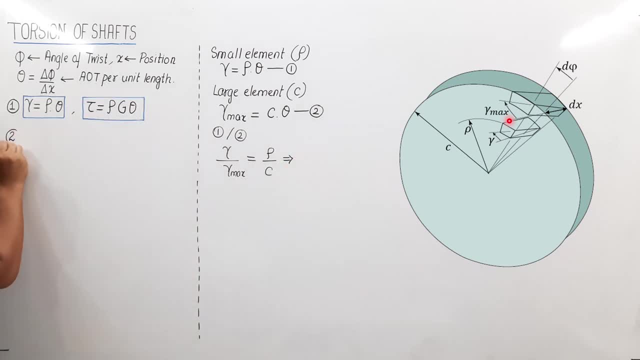 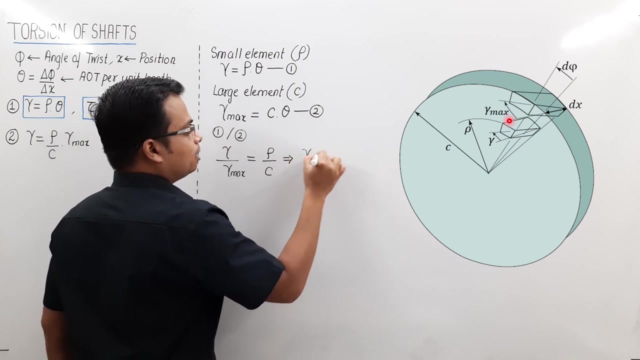 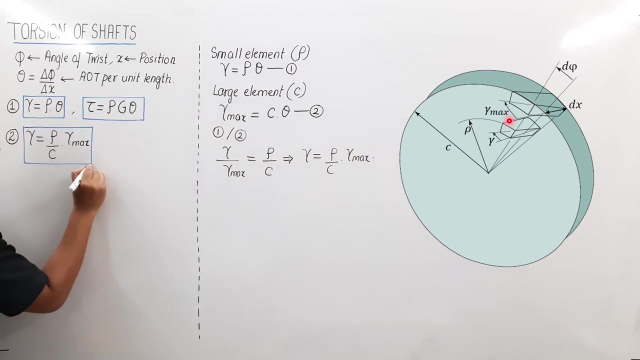 write this as. let me write it over here. Point number two: What Gamma equals. gamma is equal to rho by c times of gamma max. Lovely, Okay, Let me write it here also: Gamma is equal to rho by c times of gamma max. This is one version of shear strain. Another version is going to be. 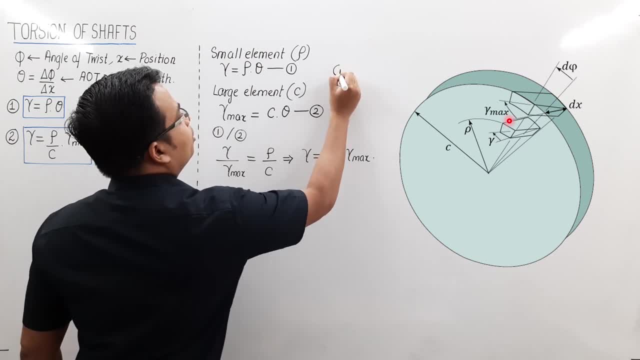 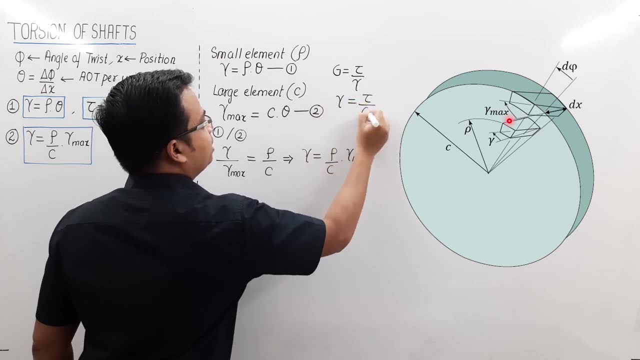 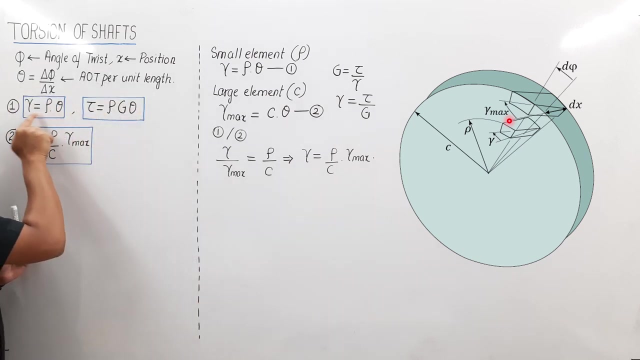 shear stress. Let me tell you how Modulus of rigidity Shear stress upon shear strain. So shear strain is equal to shear stress over modulus of rigidity. Just watch this, Keep watching. Just like this relationship tells us that on increasing radial distance you increase shear. 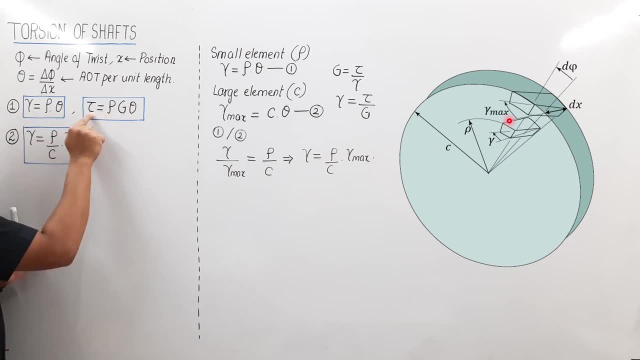 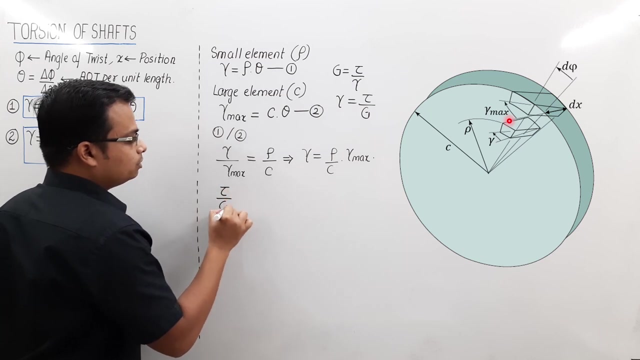 strain. This relationship tells us: on increasing radial distance, you increase shear stress. This relationship, well, this sort of, connects the maximum shear strain with any shear strain at a given time. Okay, In the same fashion, let me have: gamma equals tau over g, Gamma equals tau over g. 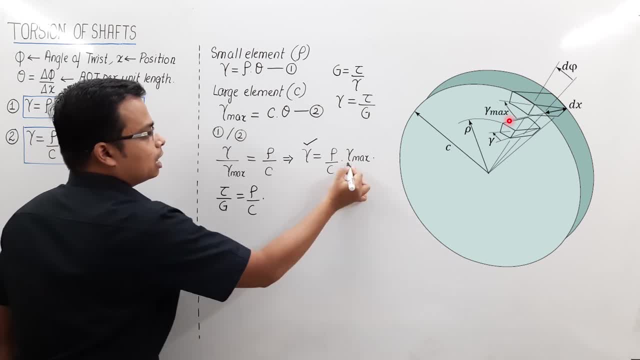 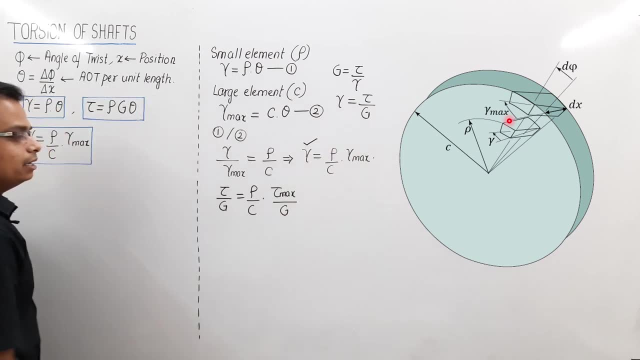 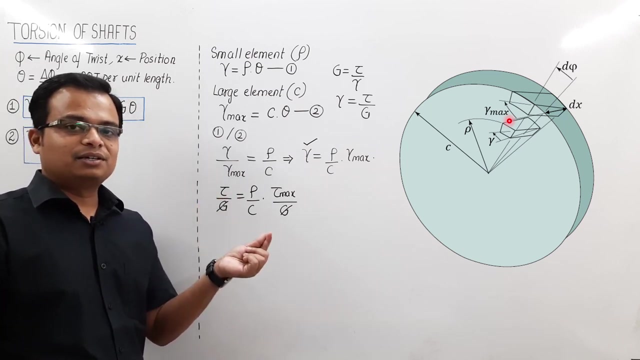 Here Is equal to rho over c, Here Gamma max, meaning maximum shear stress, And this is going to be obviously modulus of rigidity. So g and g will cancel each other out. Obviously these are the elements from the same disk, from the same materials, So modulus of rigidity will stay same. 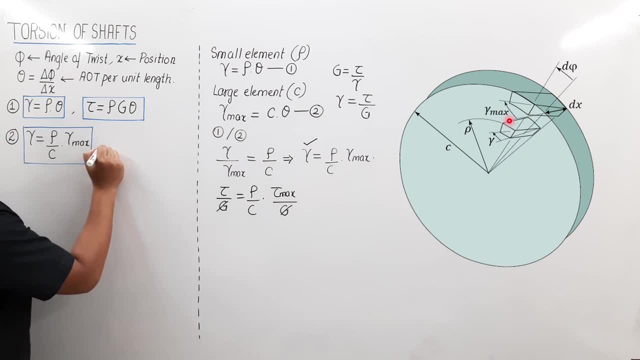 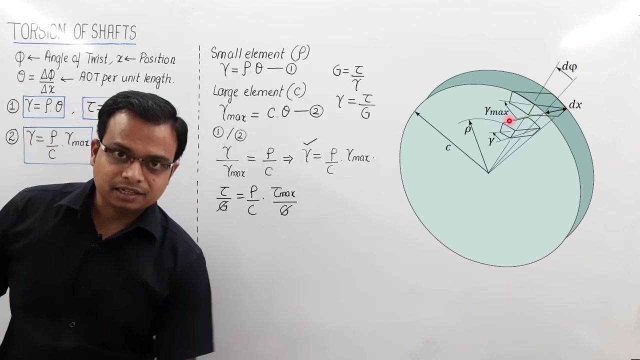 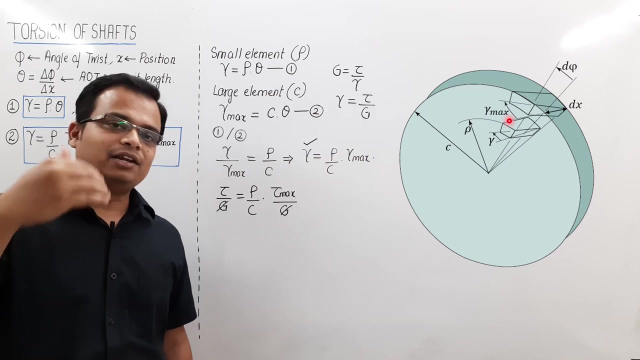 And this is another important Relationship, Which says that tau is equal to rho upon c times of tau max. Comparison is done Time to time to work out the torsion formula which will give the value of shear stress at any point on the cross section. Okay, Let's do that. That's the comparison. 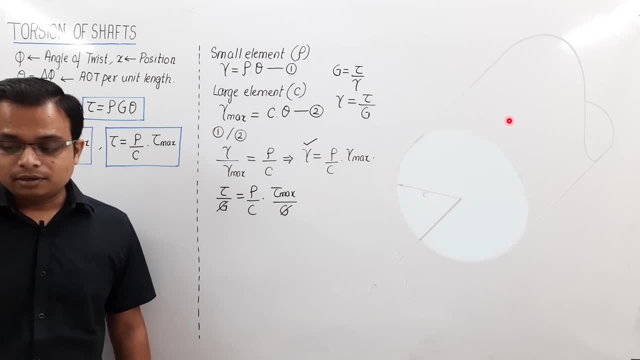 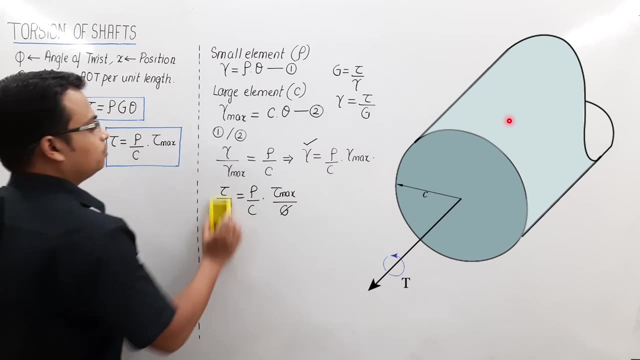 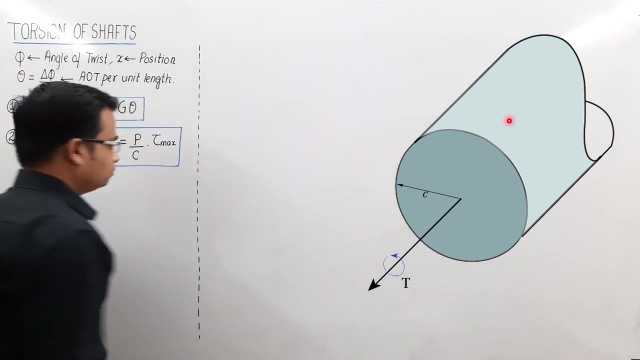 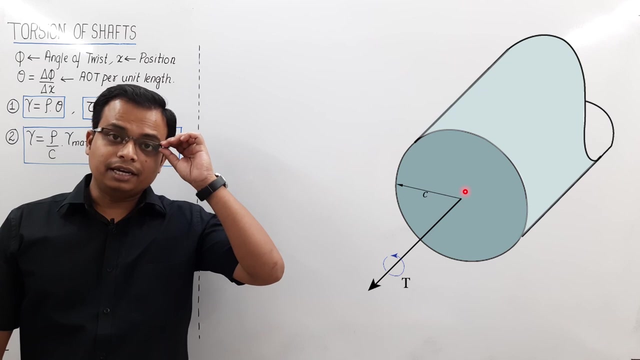 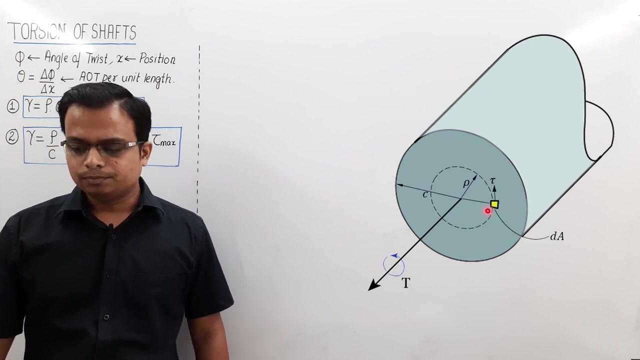 All right, Please note this down, and We are at the final stage of our today's lecture. Just watch this. As I told you, Increasing value of distance will increase shear strain will increase shear stress. Take an element over here at a distance rho. this length of the arrow represents the magnitude of shear stress. 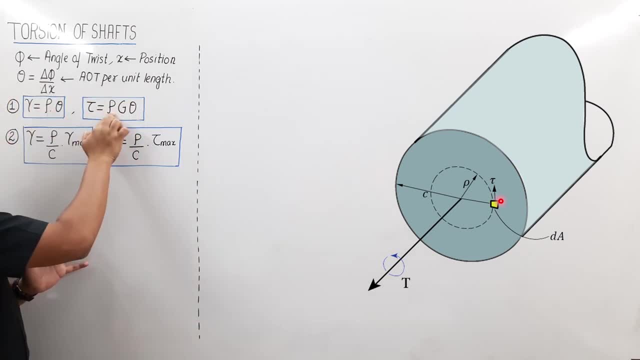 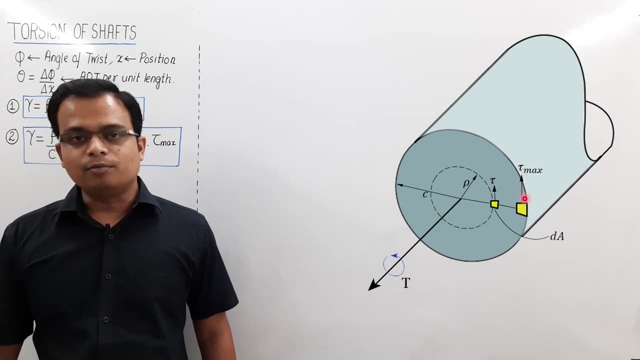 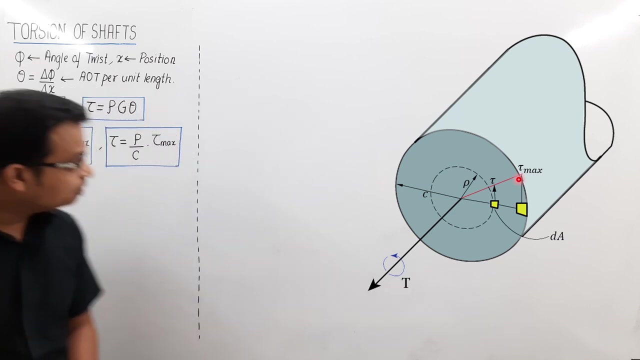 So if rho increases, shear stress increases. If rho becomes c, this tau will become tau maximum. Here it is: Rho becomes c, then tau will become tau maximum. Obviously, this is a linear plot, Linear plot. Why is this a linear plot? You will understand this from here. Tau is equal to rho. 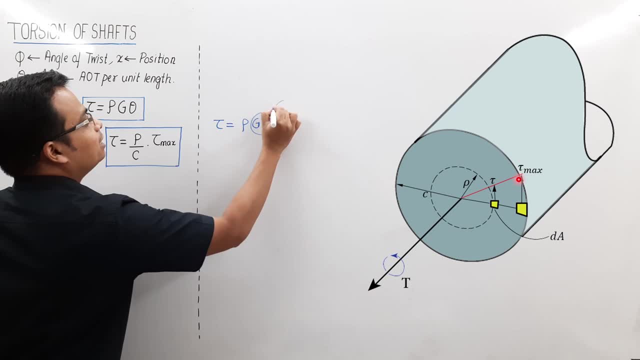 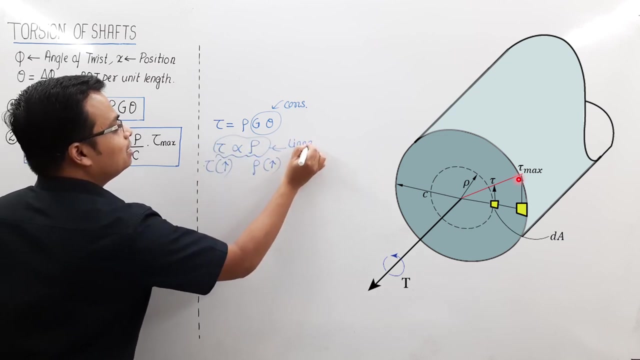 g, theta, g and theta. what are they? These are constants. So tau is directly proportional to rho. So if rho increases, tau also increases. What kind of a relationship is this? This is a linear relationship. And if it is a linear relationship, if it is directly proportional. 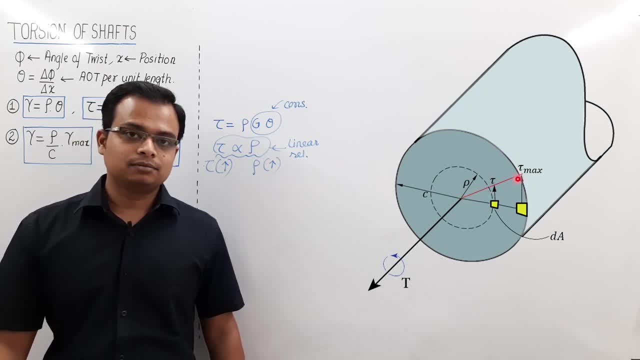 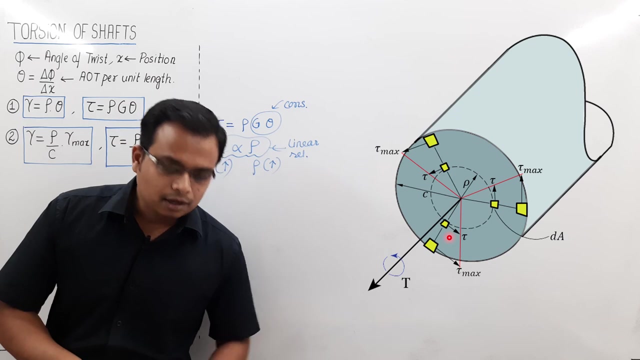 and if you happen to make a plot, you will see this straight line. That's it. If you mark any other point, Like here, you will again have this relationship. This is the sketch Mark anywhere else. Again, that is exactly. this is how shear stresses can be plotted across any radial line. let's say: 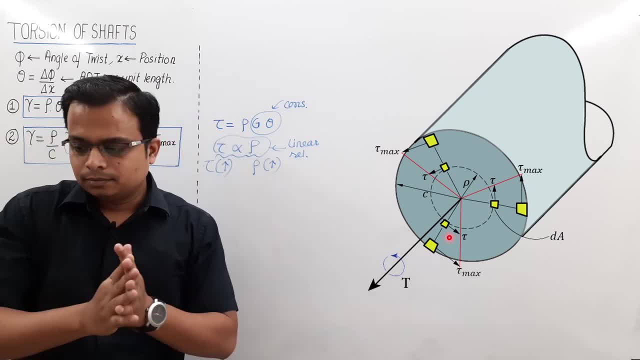 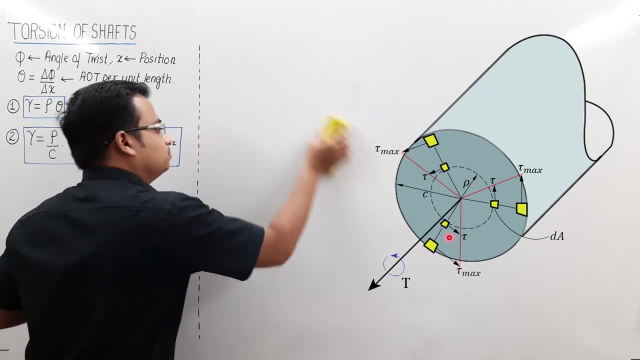 Okay, But sir, what are we getting at? We basically need a formula to calculate the shear stress. Be patient, Be patient. Now, just try to focus on this very single line. We are going to calculate the shear stress. We are going to calculate the shear. 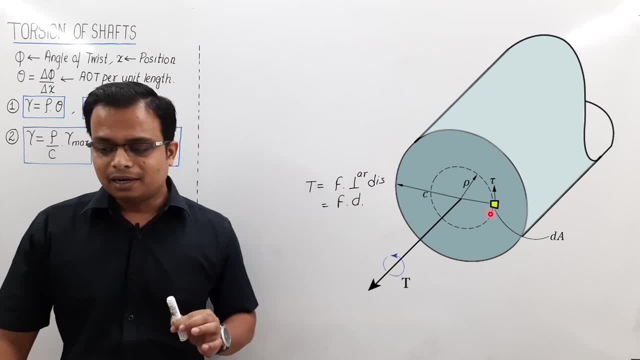 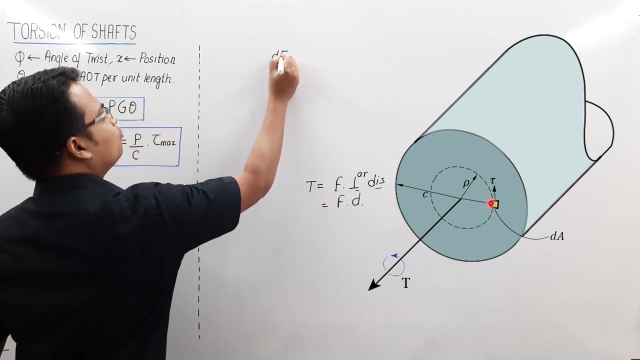 stress of each single element. There are other elements also, I know that. But let us try to work out the torque. because of this torque acting due to the force on this small area d Torque, What is torque Force? into perpendicular distance, Small area, there is going to be some very small force. 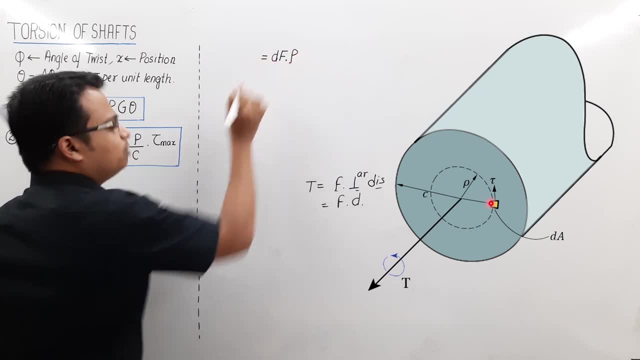 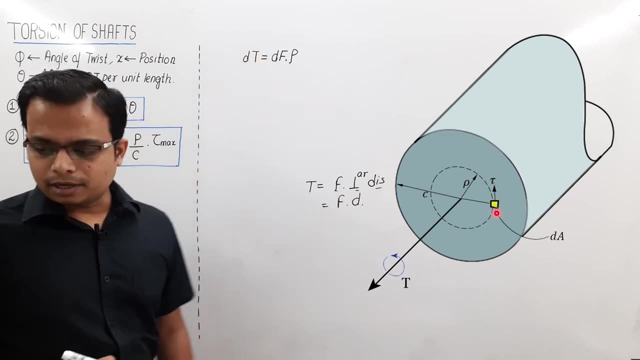 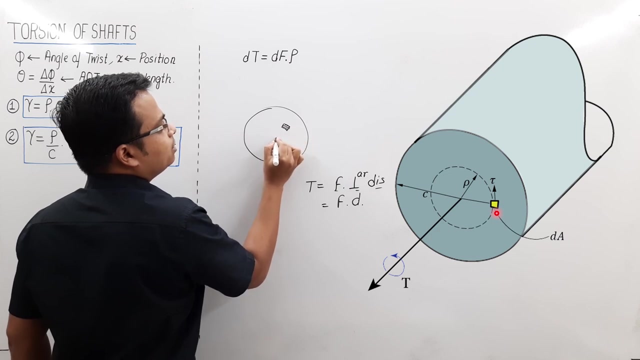 multiplied by this perpendicular distance is rho. Because of this, because of this extremely small area, there is going to be some extremely small torque, isn't it Okay? For example, if we are talking about this cross section, we are talking about this very small area which is at 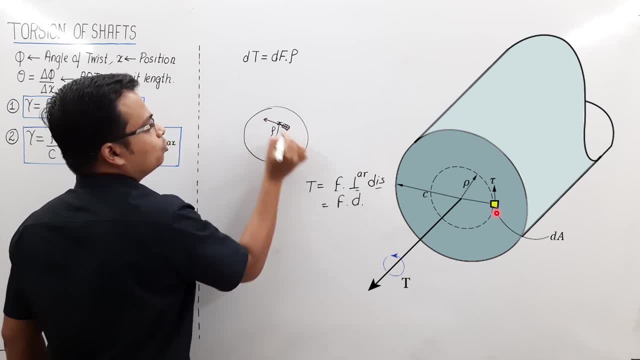 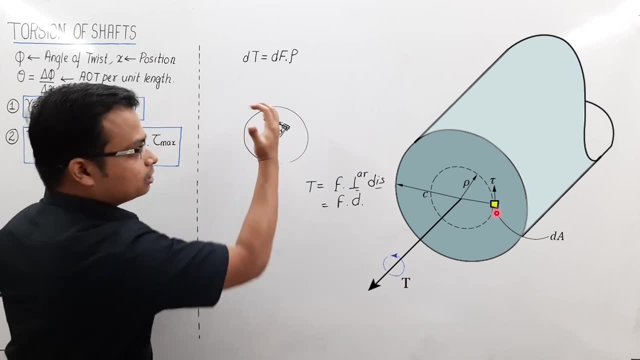 the distance of rho, right. so this is the force and this is the radial distance, r. this is the force, df. so df multiplied by r will give you the torque this way, in this direction. this direction i am talking about, all right. similarly, there will be other elements also somewhere here, some kind of 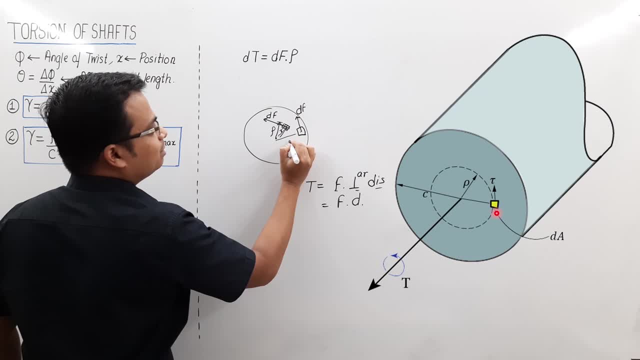 force, right, some kind of force. and let's say, the radial distance is something else. let's say this is alpha. so this df multiplied by alpha will give you another torque. similarly, there are going to be so many elements which are going to contribute towards this final torque, so this torque, essentially, 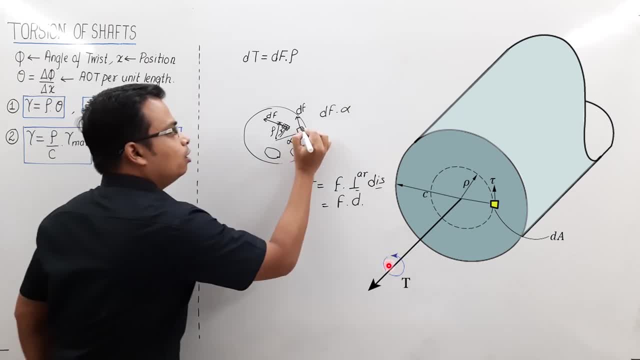 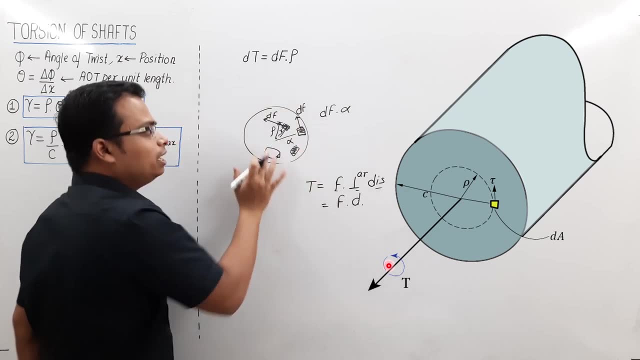 can be written as the summation of: torque due to force on this area, torque due to force on this area, torque due to force on this area, and once you, once you, once you take into account all the areas and you sum them up, it is the area of the entire cross section and when you do that, you will have 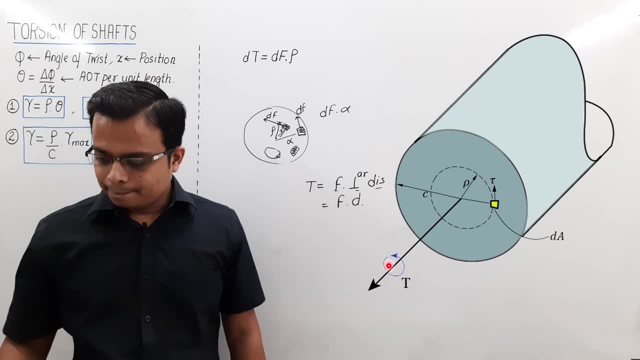 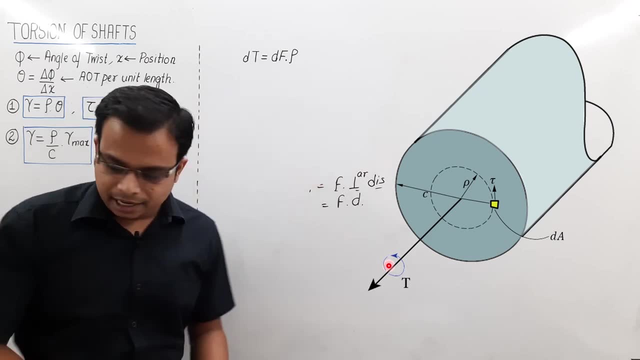 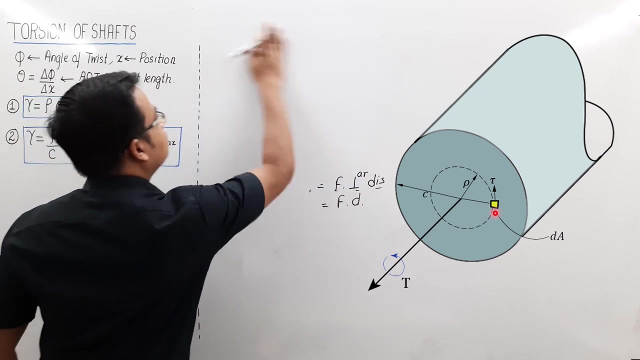 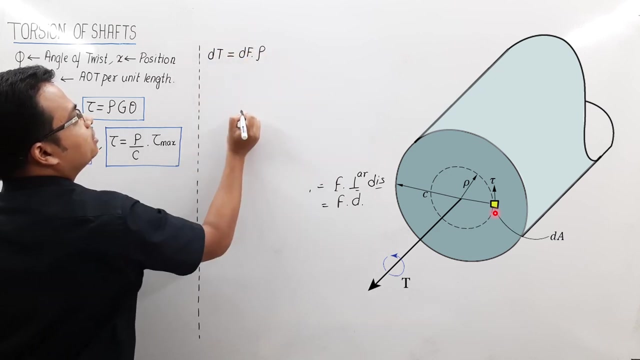 a torque about this axis, right? okay, let's simplify this. so take the torque acting due to a force on a very small area, da, that is df multiplied by rho. and now the stuff is going to be very simple. let me rewrite this small torque: dt is nothing but equal to df multiplied by the perpendicular distance, rho. 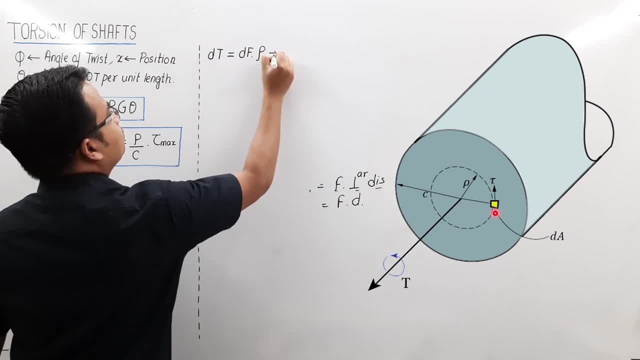 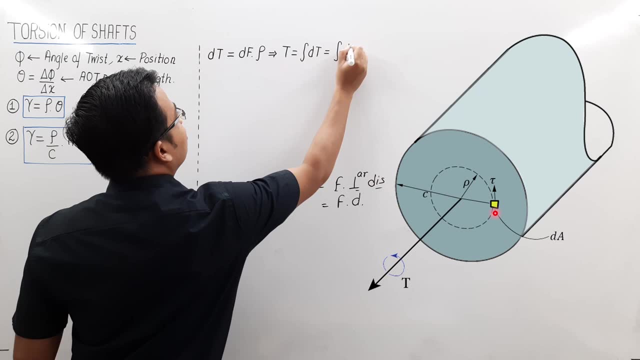 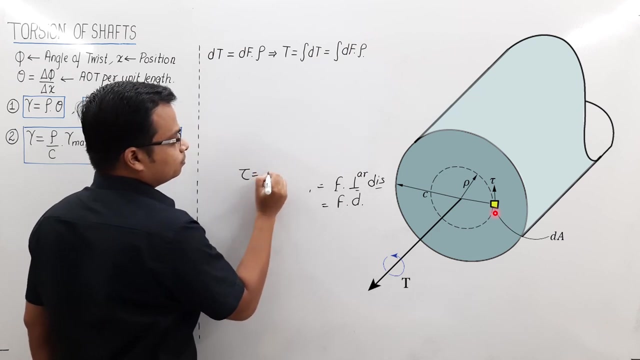 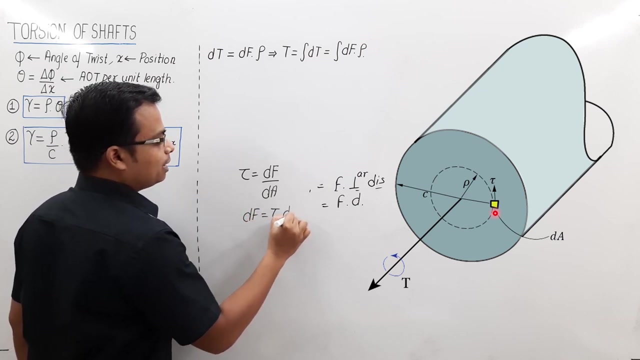 so in order to get the value of total torque, total torque t can be written as an integration of all the torque, df multiplied by the integral of df multiplied by rho. so what is df equal to? you know very well: shear stress, force over area. so force is equal to stress multiplied by area. let's do this, let's. 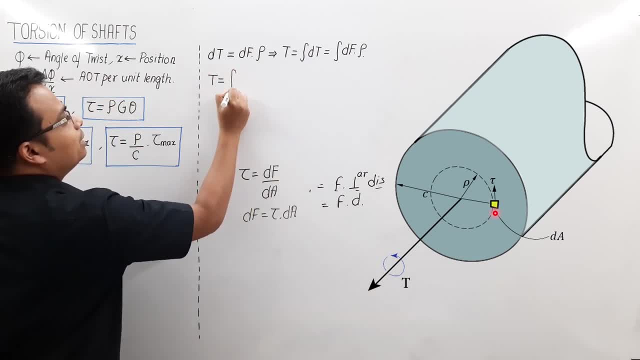 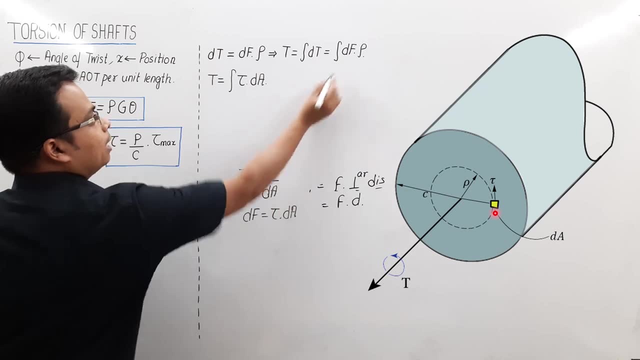 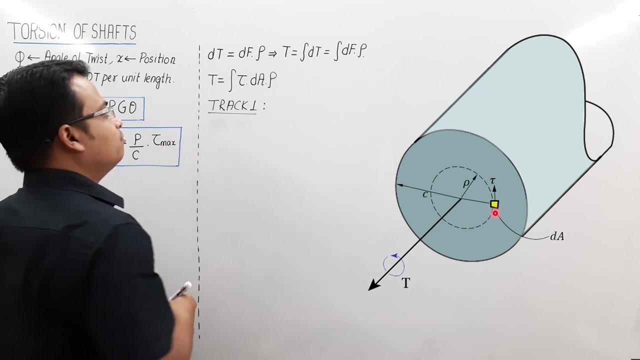 finish it, torque. t is equal to integration of what is df, tau, d, a, and that's the integral of is row. So let us not divert this analysis into two tracks. Let us talk about track one first: tau da and row tau can essentially be written like this: Okay, so what t is equal to integration? 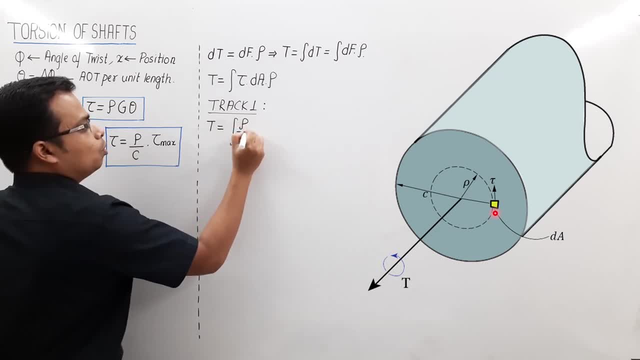 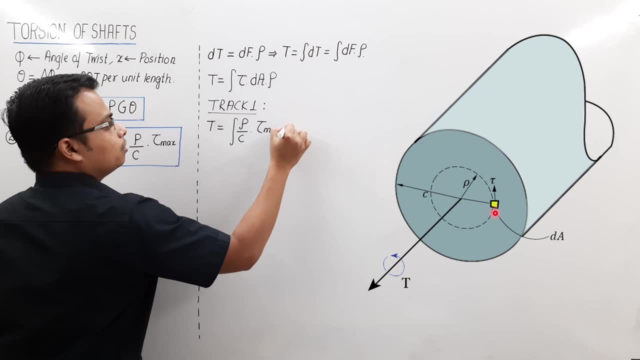 of row by C, row by C, times of tau max, lovely, Okay. and then you've got da and you've got row, So row and row will become row square. So, essentially, what are the constants? Well, tau max, well, it's a constant, and the outermost fiber, tau max, and C is also a constant, Okay. 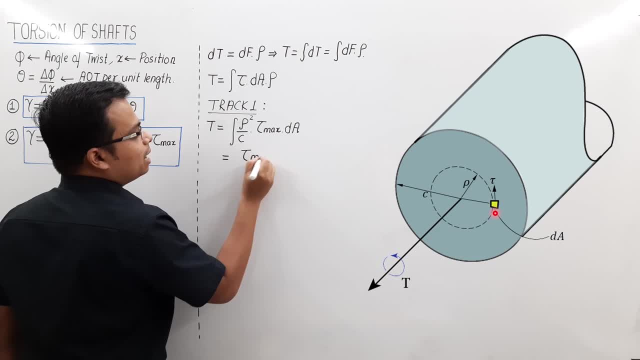 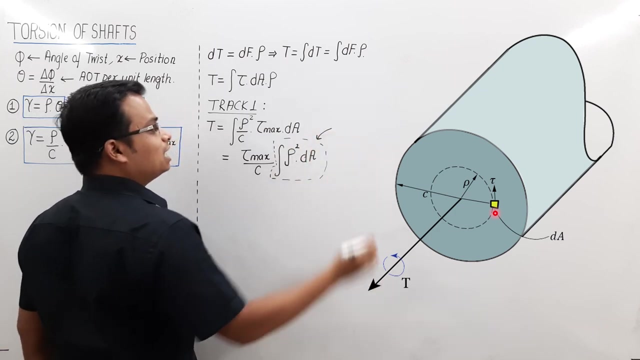 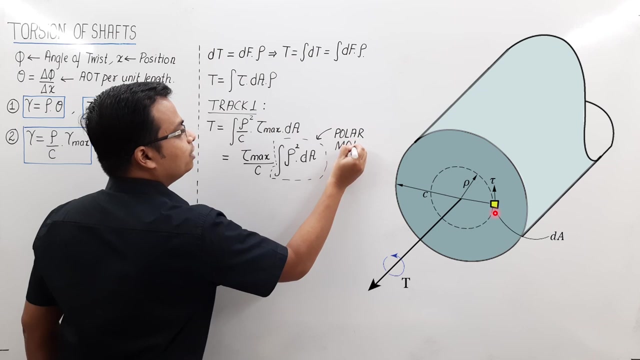 so what we have is this relationship: tau max upon C, integration of row square. this is row square da. Now, this is a very important junction of our analysis. This is what has been defined as- please note this down- polar moment of inertia. must have heard about it. This is polar moment. 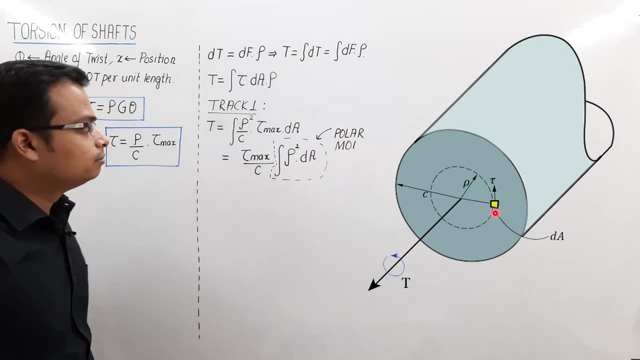 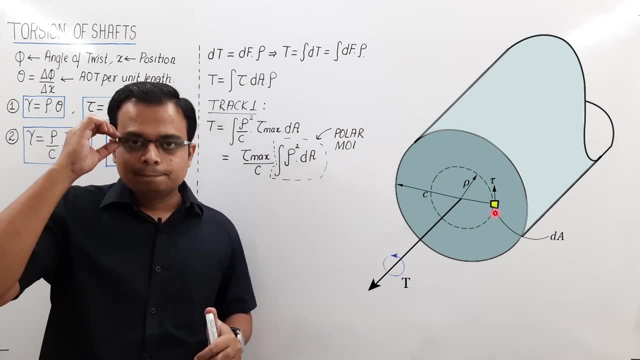 of inertia, And this comes into the picture of when we analyze a circular shaft subjected to some kind of torque. If you've seen my video on bending moments- not bending moment, but bending of beams, rather- there also we come across a different kind of inertia. That was the area. 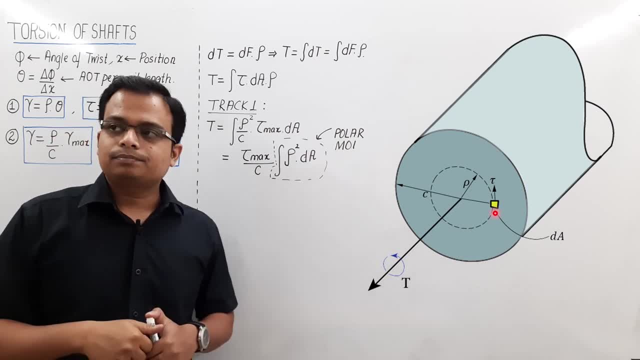 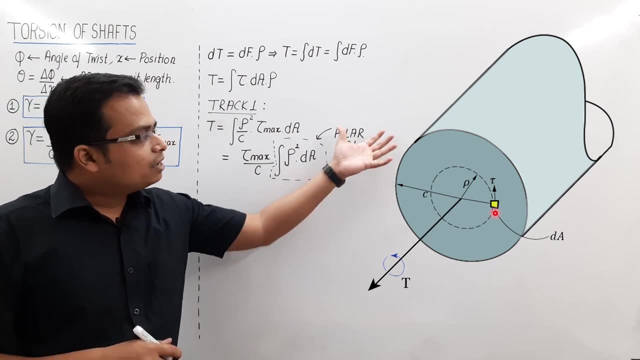 moment of inertia right depends on how the beam mints You could have. you can calculate xx, you can calculate I yy. Here this is a different sort of arrangement. Here we have polar moment of inertia. So this is the radial distance, row square da. But what is the value of this polar? 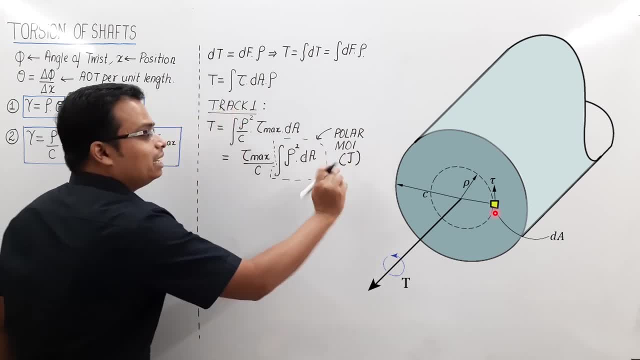 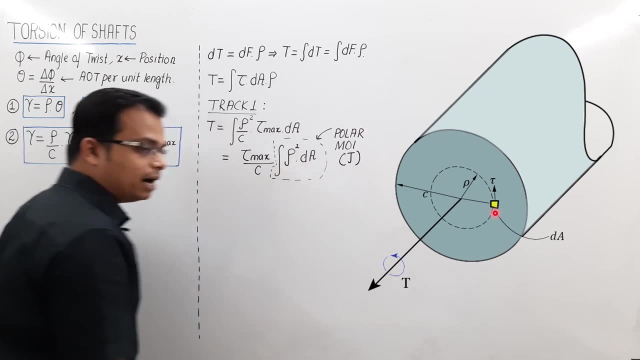 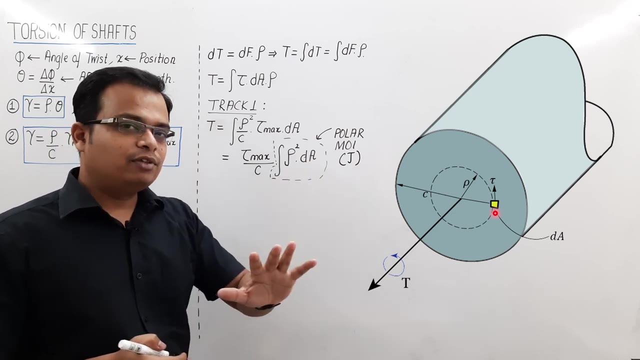 of moment of inertia, and it is represented by j. what is j equal to mathematically? how can we calculate that? that is also very important, and it is a geometrical property. does not matter what the material is. You can calculate it. Right At the end of the video I'll let you know how. for a circular: 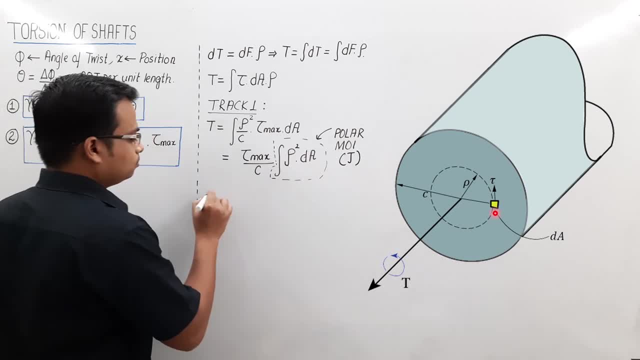 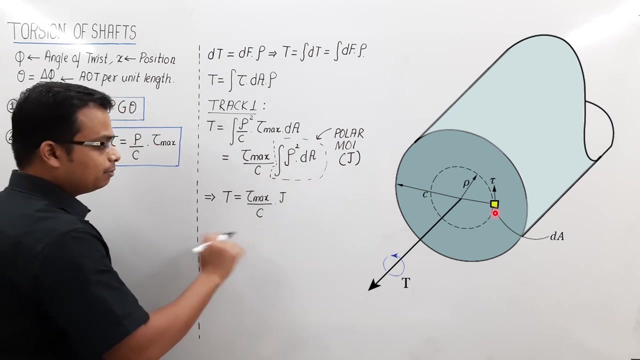 shaft j can be calculated. Okay, right now Let me just write: torque t is equal to. this is going to be tau max by c, tau max over c times of polar moment of inertia, j. So this, essentially, is the torsion formula. Let me frame this in a better fashion. tau max is equal to t by j, c, or t, j by 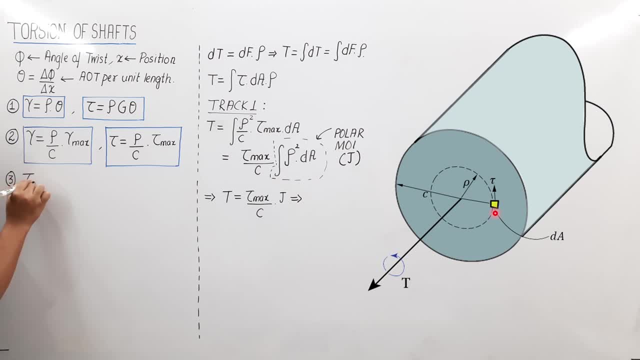 c, Third version. one tau max maximum shear stress can be calculated using. this is the torsion form line, part t, that is the torque multiplied by the c, that is the radius, radius of the shaft. you know this divided by polar moment of inertia. This is the torsion formula and the much more simplified 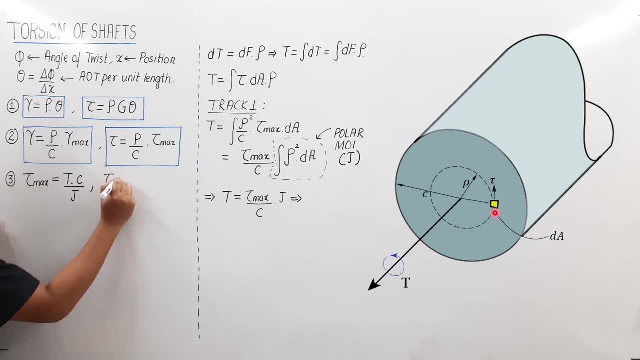 version. replace this tau max by simply tau. this torque t multiplied by at any radial distance row, at any radial distance row, The torque is not the torque, but the shear stress is tau divided by, obviously, the polar moment of inertia. This is the torsion formula. Both the 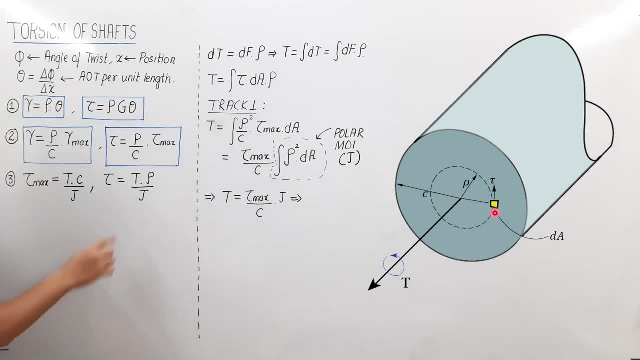 versions are absolutely accurate. You can use either of them. This is what you need to remember. keep in mind, right, Can you? can you? can you relate this to the bending stress, My eye formula, my eye instead of bending moment. we have torque instead of this distance from the neutral axis. 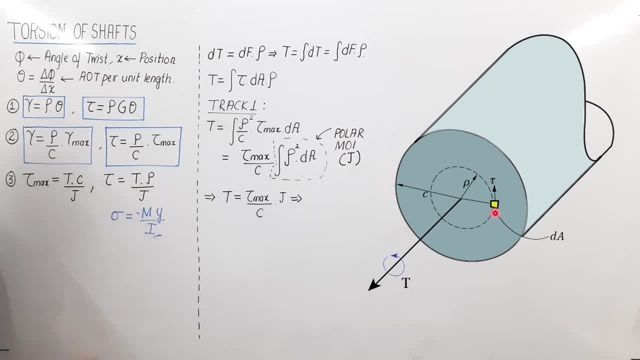 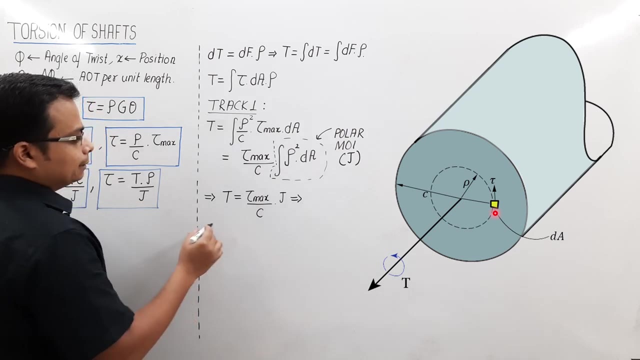 we have the radial distance instead of the area. moment of inertia. Now we have the polar moment of inertia. Try to relate it. Let me talk about a different version. track to track to. that is also very important Right over here. Watch this. We are going to continue from here. Okay, so torque t is nothing but an integral. 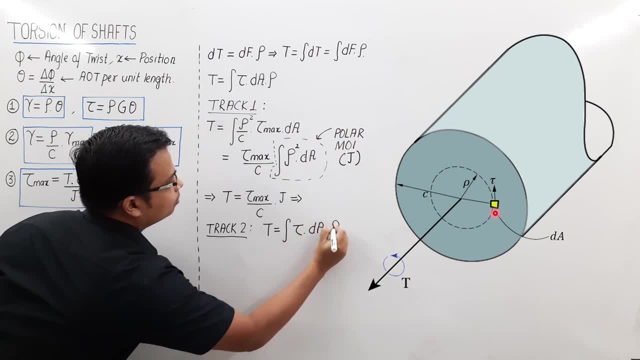 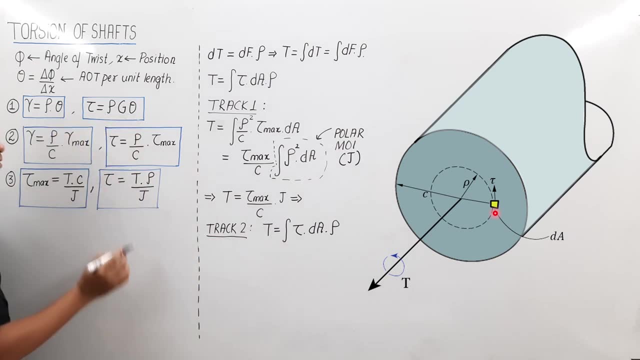 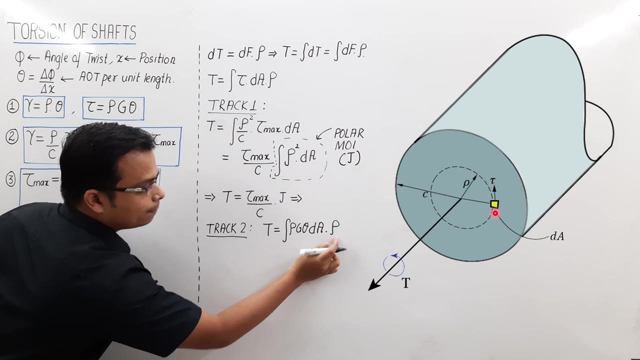 of tau da and lovely. Now, what is tau equal to in terms of shear? shear model is rho g- theta, So tau can be replaced by rho g and theta, isn't it? so this is going to become rho square And this is g, theta and da, So it's. 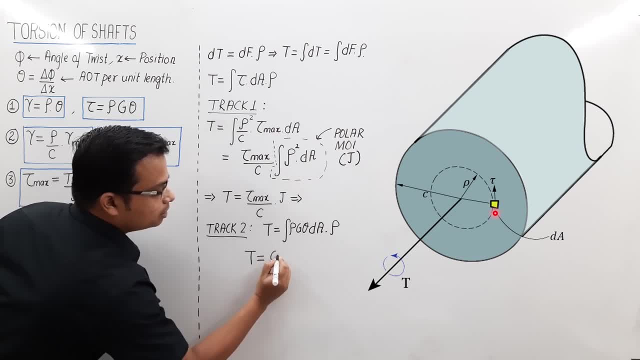 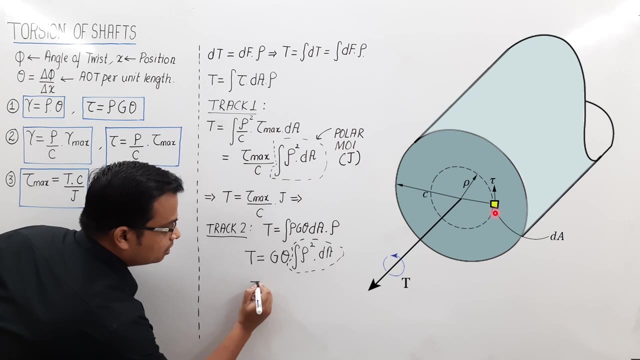 it's very simple: t is equal to, g is a constant, theta again is a constant inside the integral rho, and rho will become rho square, and this, da you know very well, Right now we have defined this as integral. integral, we have defined it as polar moment of inertia, and that is nothing, but t is. 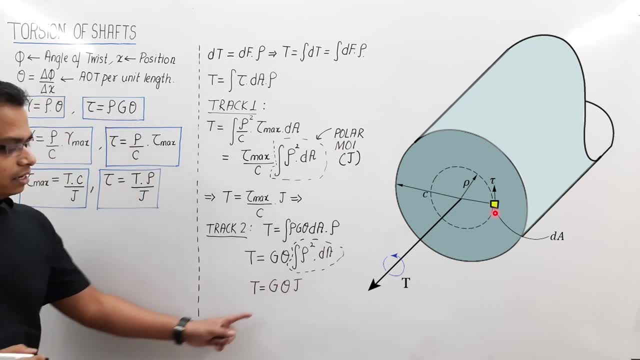 equal to g theta j. t is equal to g theta j, right? So some of the Indian textbooks you are going to find this relationship. This is track two. So t by j is equal to g theta. p is the torque applied, j is the polar moment of inertia. 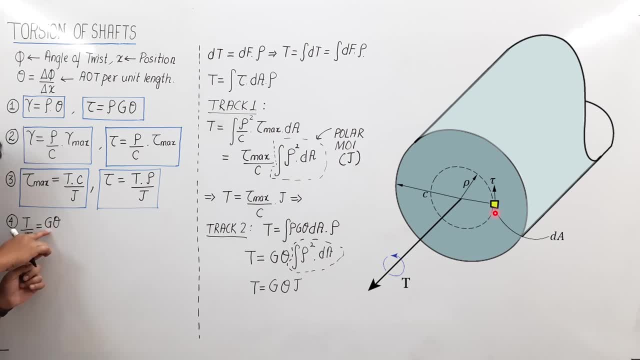 happens to be G, happens to be the shear modulus of whatever material it is. Theta is the angle of twist per unit length. Okay, This is further equal to something We can work it out. Just try to think about it. T by G, T by G, This is. T by G is equal to tau. Bring it over to. 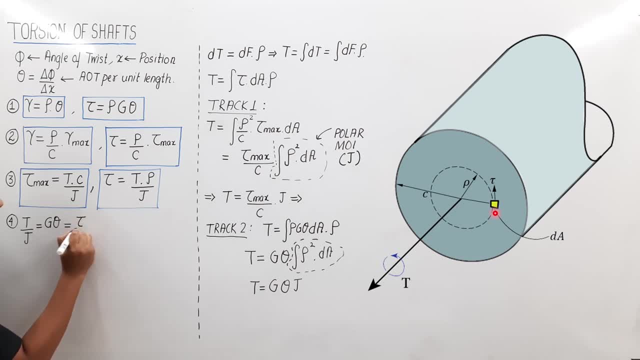 the LHS. Tau by rho. What is this equal to? Tau by rho Done. Well, basically, this is the torsion formula, Right? This is one more way of writing things up. Both of the tracks have been explored and we have reached this final conclusion. Lovely, isn't it Talking? 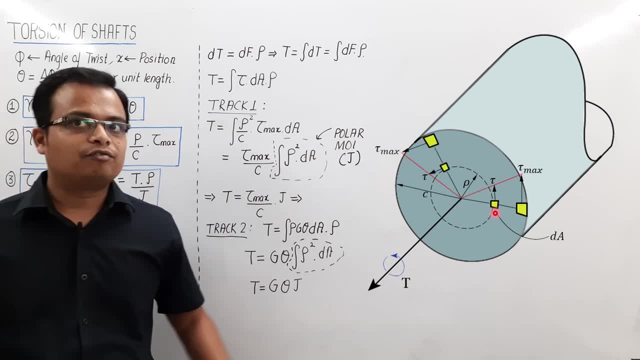 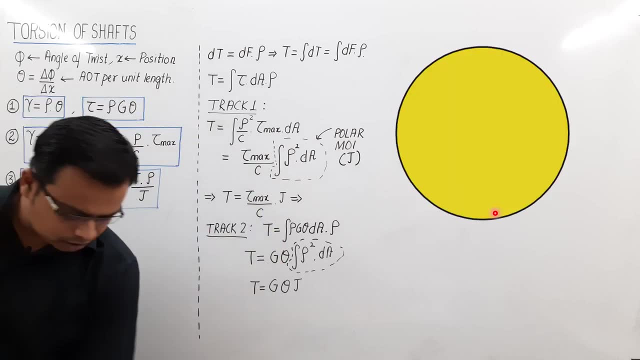 about polar moment of inertia, Of a cross section. let's say, Here we go. Let me show you. Consider this cross section. What is this? Obviously a circular cross section. How to calculate the polar moment of inertia. Polar moment of inertia: How to calculate. 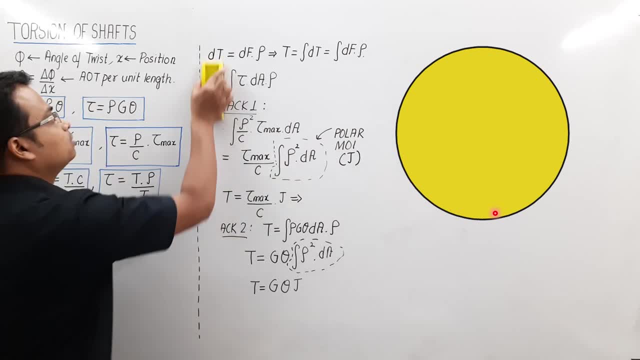 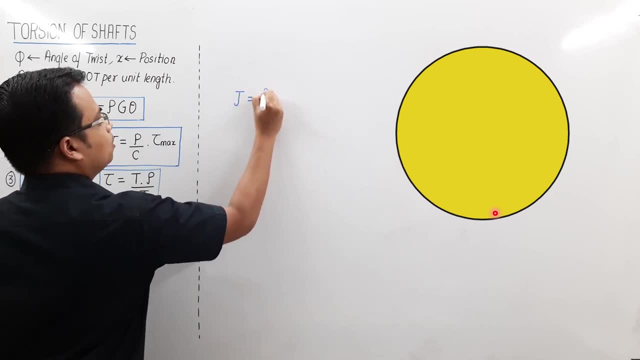 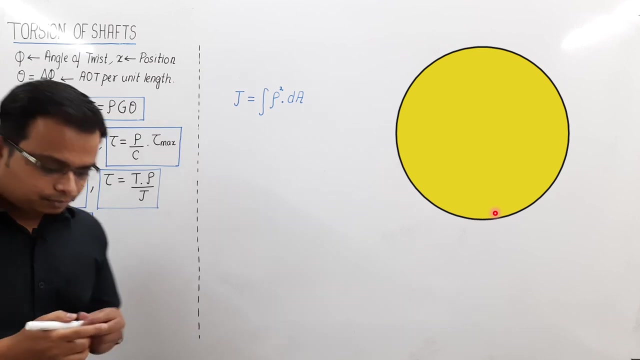 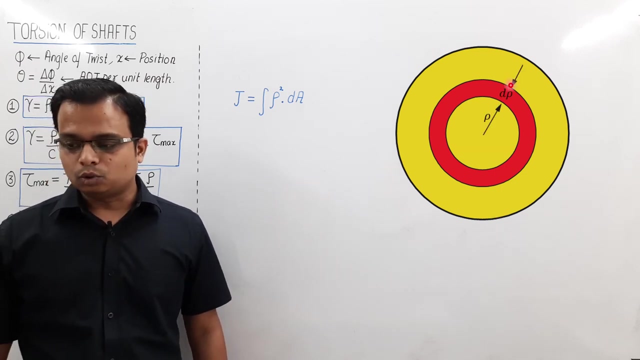 the polar moment of inertia. How to calculate the polar moment of inertia? How to calculate inertia? is integration of rho square da? Okay, let us explore this. Rho square da J is equal to integration of rho square dot da Lovely. Consider an element, a ring element, at a distance of rho, At a. 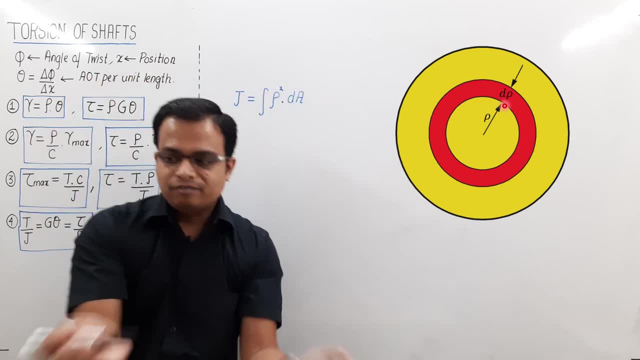 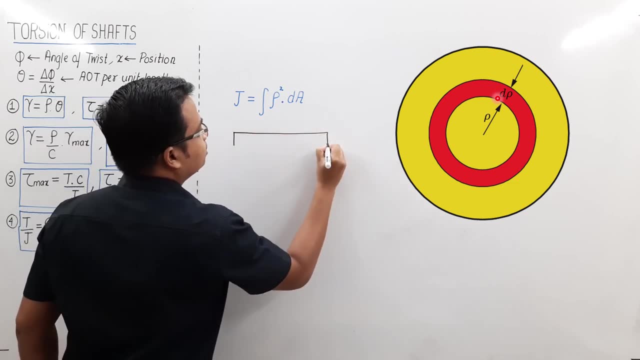 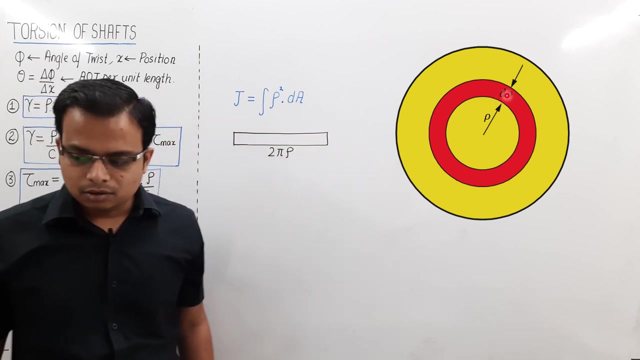 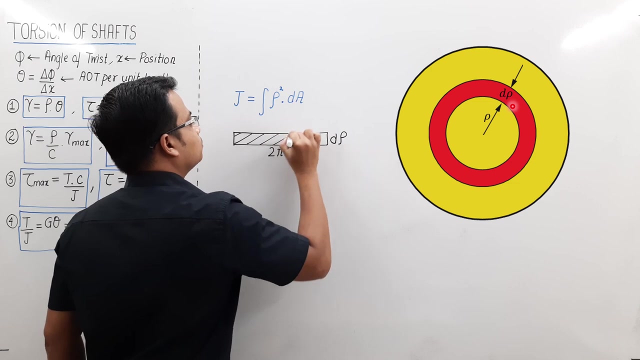 uncurl it, lay it absolutely flat. this red element, make it absolutely flat. It would look something like this, isn't it? This is going to be 2 pi rho. what is the thickness? Okay, that's a d? rho, d rho. What is this area going to be? Area of the rectangle, Nothing. 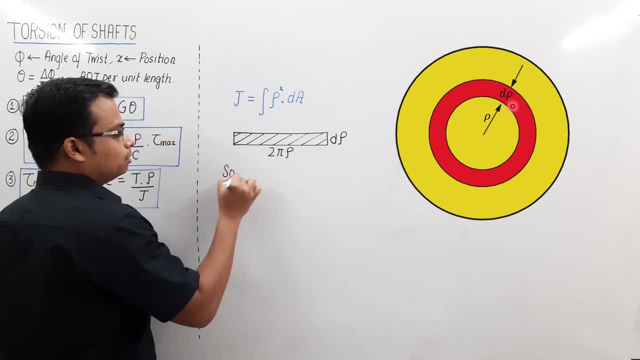 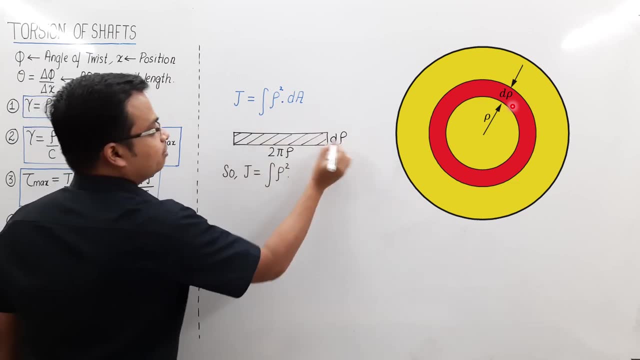 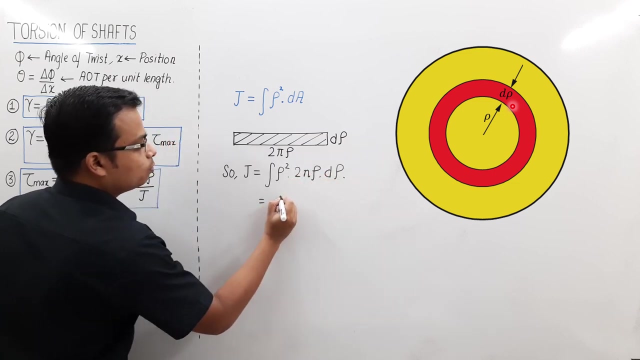 fancy: 2 pi rho, d rho. So j is equal to integration of rho square and that's dA. What is this? This is nothing but dA. this much and this much. So 2 pi rho multiplied by d rho, just solve: the integral is equal to. this is going to be 2 pi. take it outside. 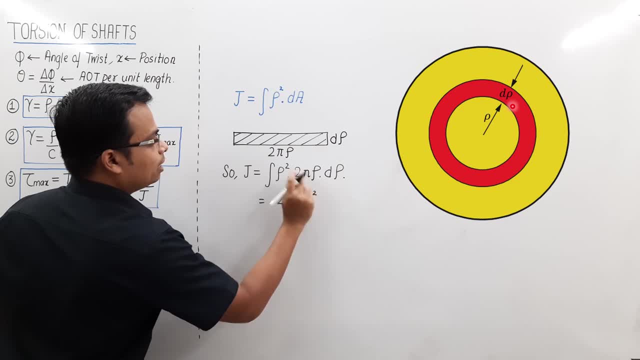 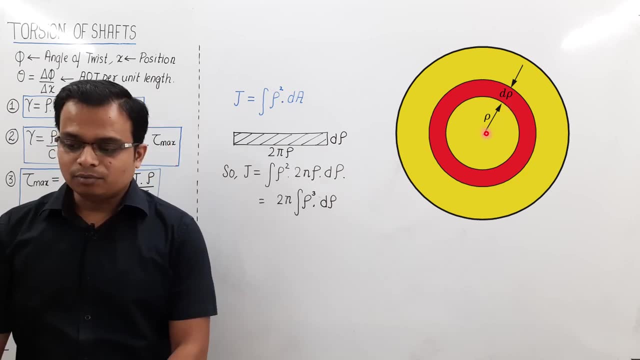 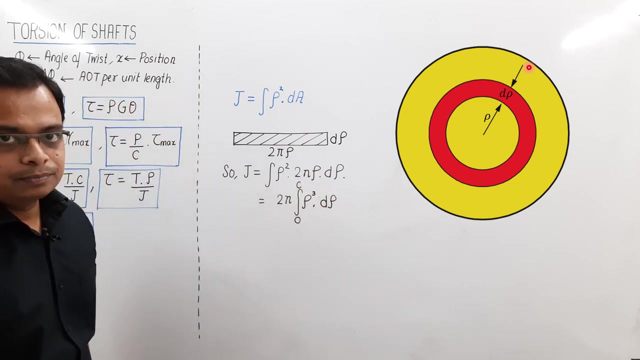 inside the integral you have got rho square and this rho cube dot d rho. So let's say we are extending from this centre to the outside. so this is from 0 to C. C happens to be the radius of the circle or the cross section. Just solve the integral. This is going to 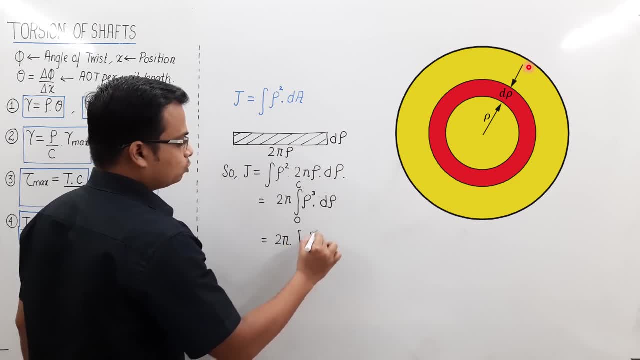 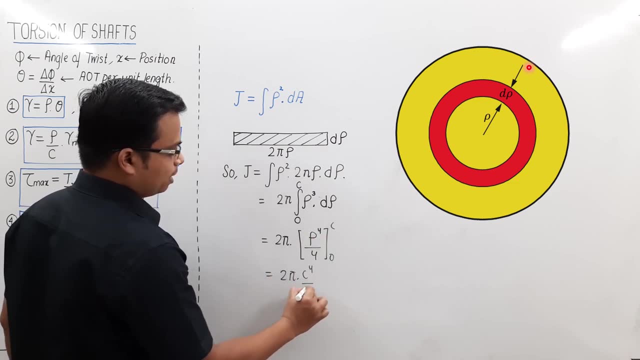 be 2 pi. this is going to be rho raised to 4 by 4, the limits are from 0 to C. So this is going to be 2 pi times of C to the power 4 by for undone pi by 2, pi by 2 dot C to 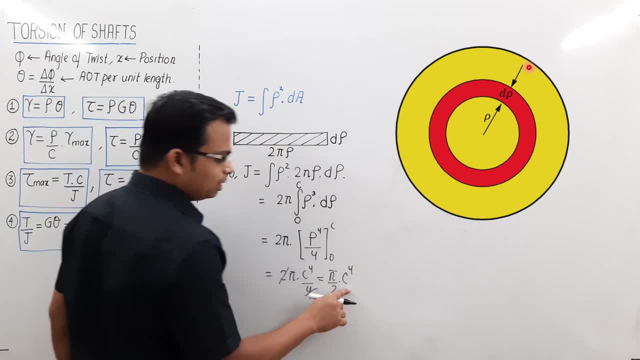 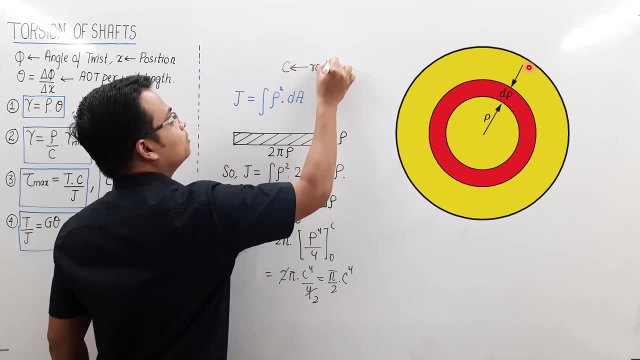 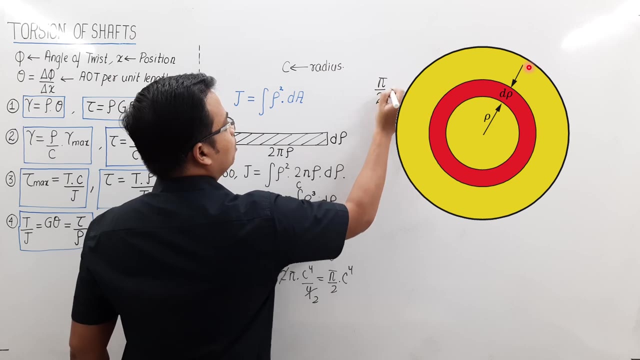 the power 4.. Some of the embedded textbooks- they usually this is in terms of radius. C is nothing but the radius. let me clarify: C is the radius, Ok, in some of the textbooks you will also have found diameter also. So its pi by 2 and C raised to 4.. This is the 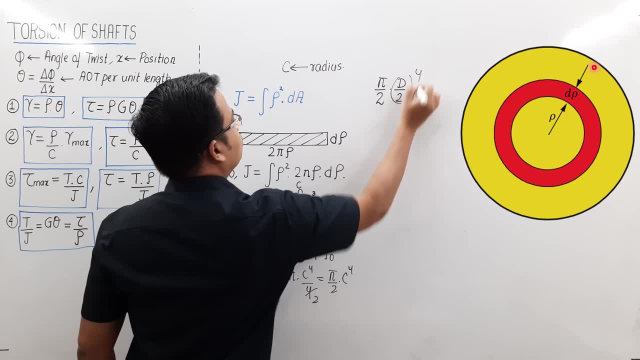 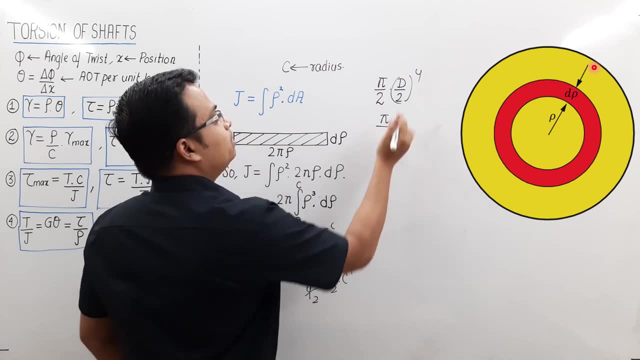 radius. Radius is half of diameter and Auf r leader band parts Docker, month and Zoe a raise to 4.. But I think it is So in some of the textbooks you will find. fondant 2 is 32 pi by 32 d to the power 4, so that is also perfectly correct. this also can be used in terms 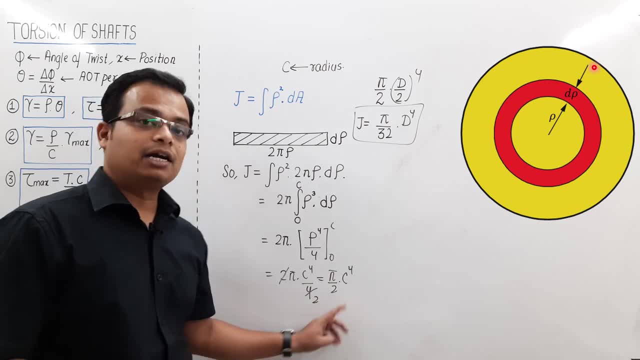 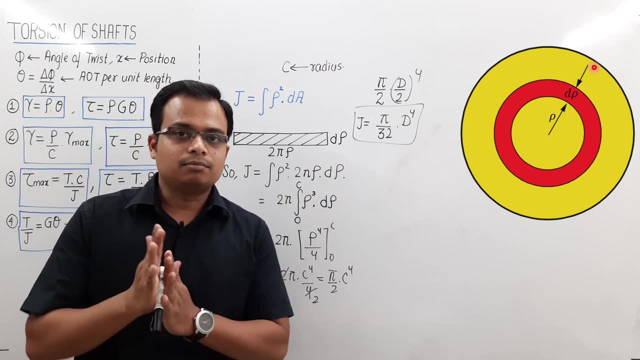 of diameter. this is in terms of radius. radius, i have taken it as c and not r, right? so, guys, that was all for today's lecture. i'm going to see you again with some numericals on this very topic. it's going to be fun. that was all for today. i'm going to see you again in the next video. until then, take, care, have a nice day, keep learning, keep watching. thank you.